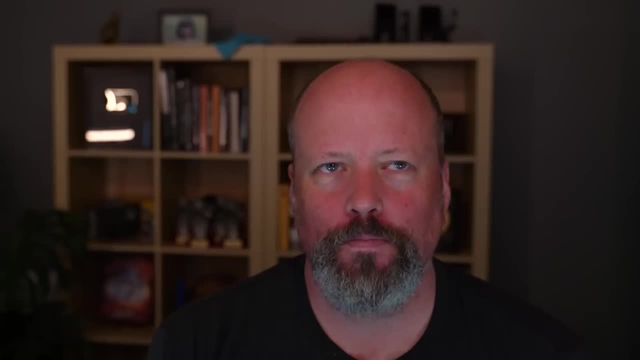 scenes. there's an incredibly complicated process to take images taken by a telescope that could be orbiting the Earth, that could be more than a million kilometers away from Earth, to transmit it to our planet, to process the images so that the scientists can work on them And, at the same, 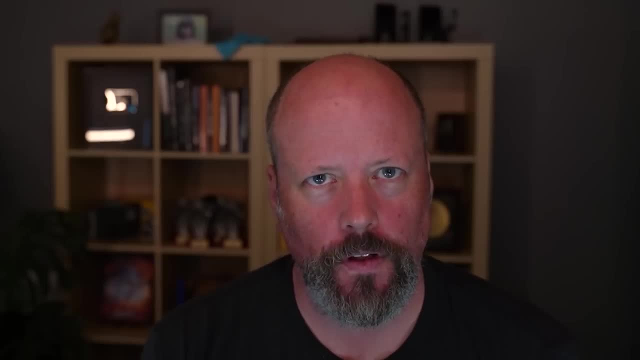 time. there's something to be said for making these images beautiful so that we can appreciate them. I mean, who hasn't got an image from the Hubble Space Telescope as the background on their phone? It really takes us, transports us to these places, So it's a lot of work to produce one of these. 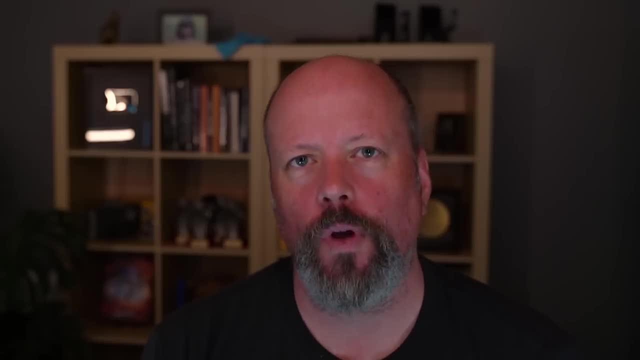 images, And I think the best person in the industry right now is a woman named Judy Schmidt, And she's not a scientist, but she is one of the most skilled and capable image processors out there. She goes through the Hubble archive, the JWST archive, as well as archives. 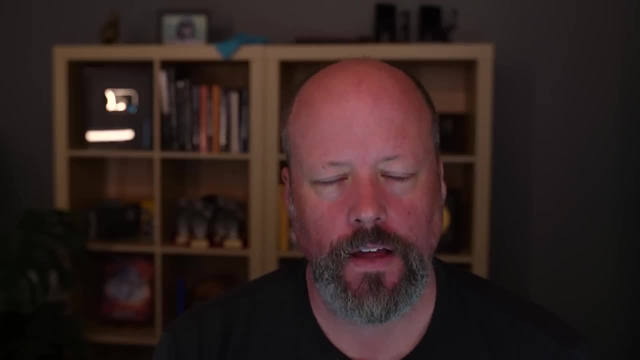 from other spacecraft and pulls in the raw data and then works with it in Photoshop to be able to produce images that are just objectively beautiful, And so I had a chance to sit down and chat with her. She's made some great tutorials out on the internet So you can learn how she finds the raw. 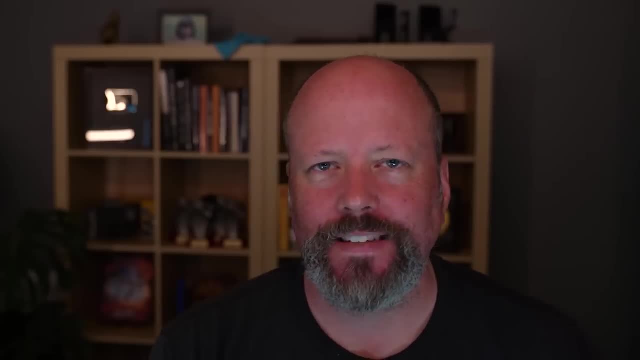 data, how she processes them, brings them into Photoshop, makes aesthetic choices about how they should look. we talked about that, some of the science that she's actually been able to get involved in, and really how you can go through this process as well. I. 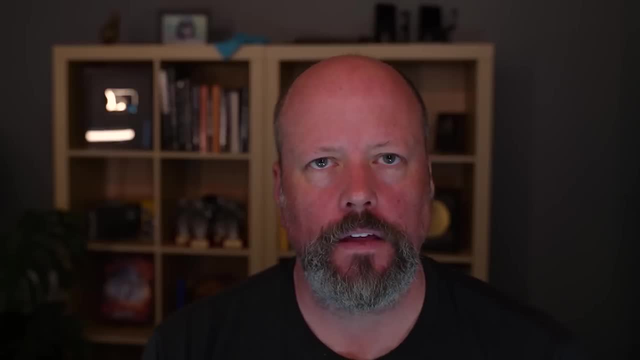 think this interview is really important. If you want to get into astrophotography, if you want to take pictures of space, it's more important to learn how to process images than to take good pictures, Because if you take good pictures but you can't process them, then you really can't make. 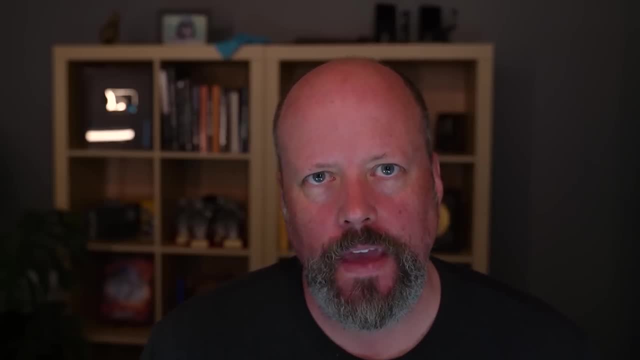 these images As good and as exciting as you know they can be, But if you learn to get really good at working with the images, then the final product will be really great. So here is a great conversation with Judy Schmidt. We talked about all these and more. I hope you enjoy. Hey, Judy, how's it going? 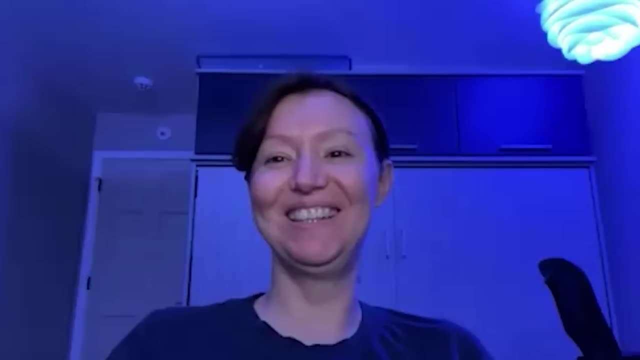 Hi, Fraser, it's going good. So how did you get into this? Well, about 10 years ago, ESA did this thing called Hubble's Hidden Treasures And they provided some resources like some tutorials and stuff and mostly just let everyone know. hey, the data are out here for any member of the public in the 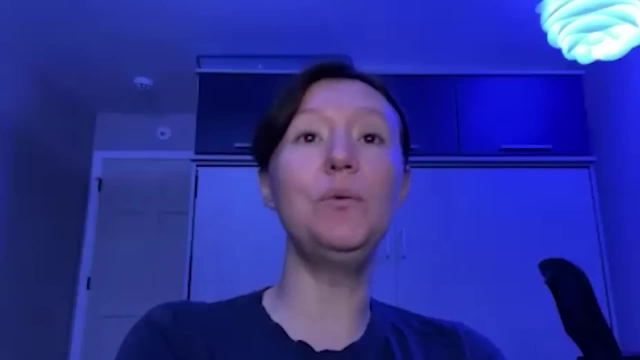 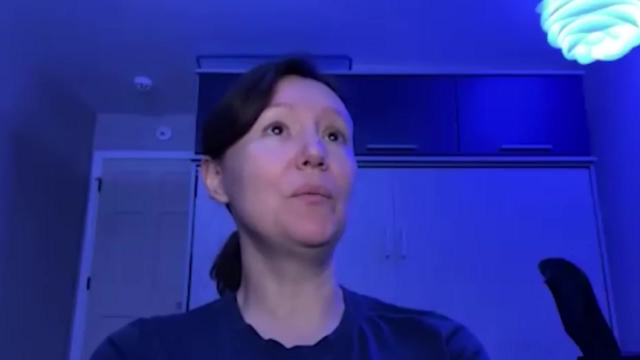 world to go download and do whatever you want with them. You could make mouse pads out of them if you want, But anyway, once I learned that, it was like what Really? I did not know. I thought you know, I thought in: 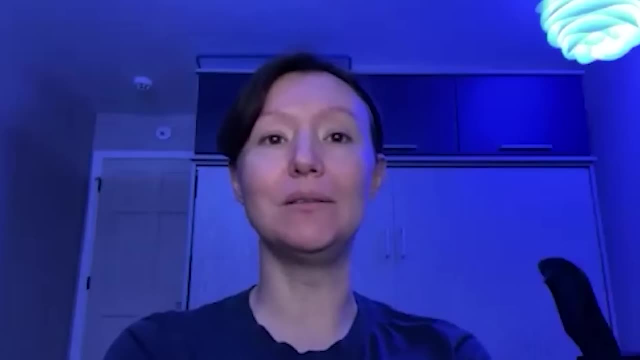 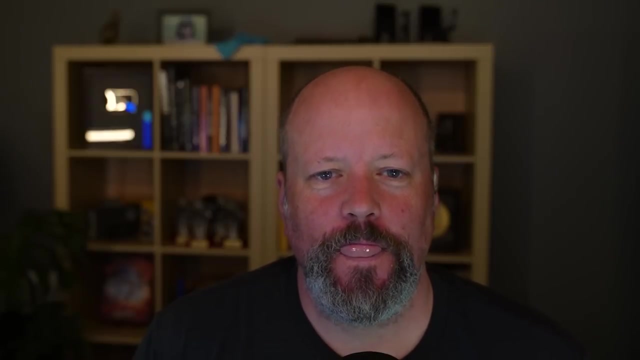 order to make space pictures, I would have to get my own telescope, learn how to go to a place where there's dark skies, And I'm just like it would never be very good. Anyway, so you had been into space And and wanted to do astrophotography, but didn't have the, the gear and the and didn't know where to. 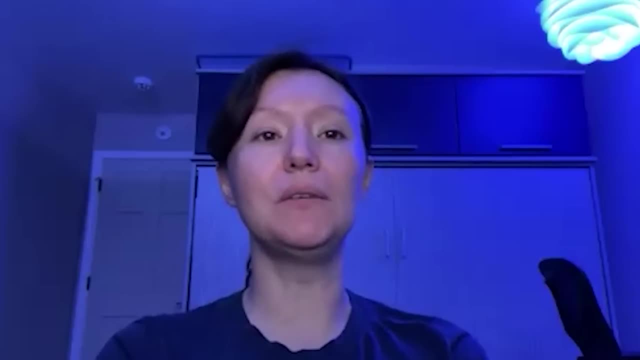 start. I probably never would have like, if anything, maybe buy some time on a remote, a remote telescope of some sort, But no, I mean I I always like it's just it's expensive And you have to go and 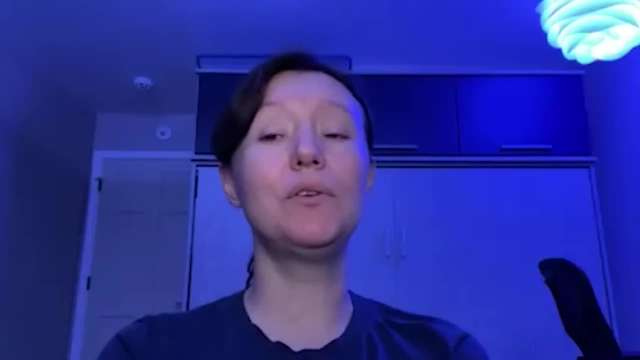 freeze your butt off. And I mean kudos to the people who who do that, who actually sit with their telescopes out in the cold of night and take some really good astrophotos, Or I don't know like people who just are so into it that they 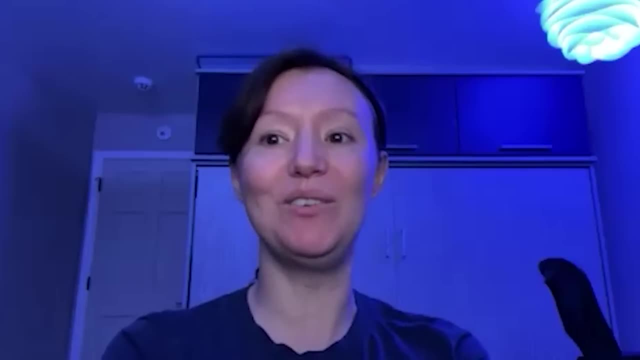 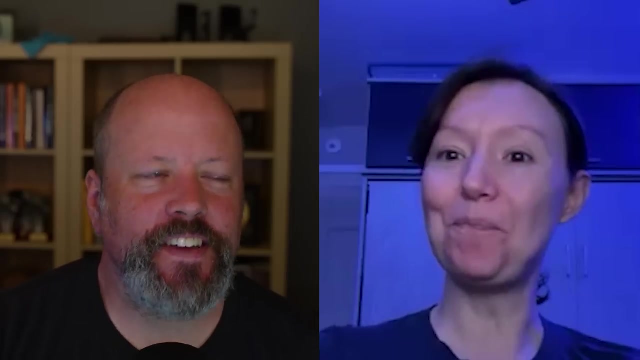 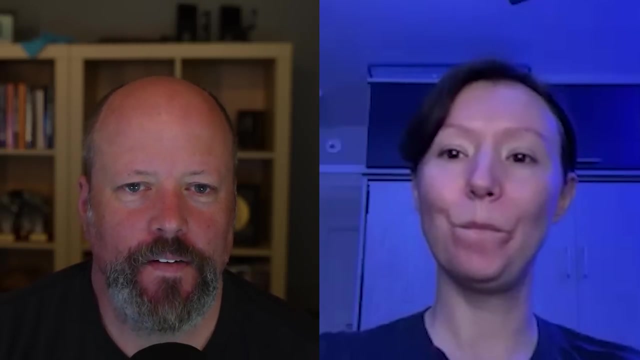 buy a whole like they build an observatory with with a retracting roof and everything for their telescope. So that's amazing. The hilarious part about this is, like I- you know, we did a sort of like a session on the telescope that I'm using, And it was you know. 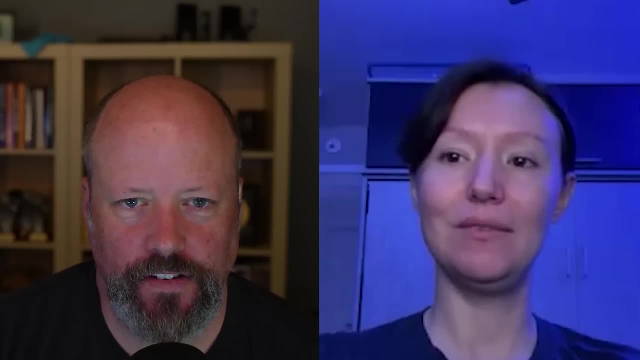 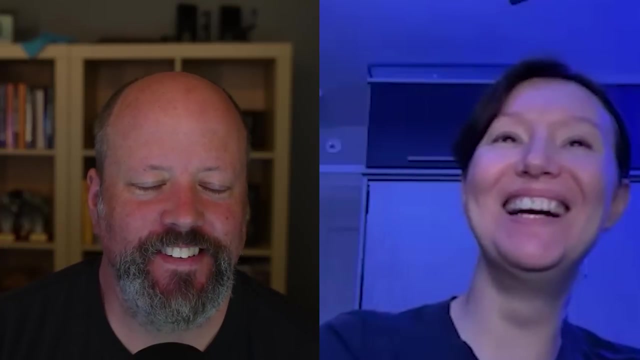 it was good, We got some great pictures and you were able to make some really nice, nice images out of them, But in the end you're like this is pointless. I have Hubble And I have no argument for you. 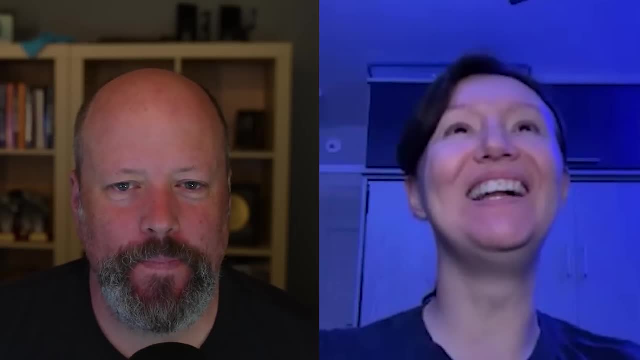 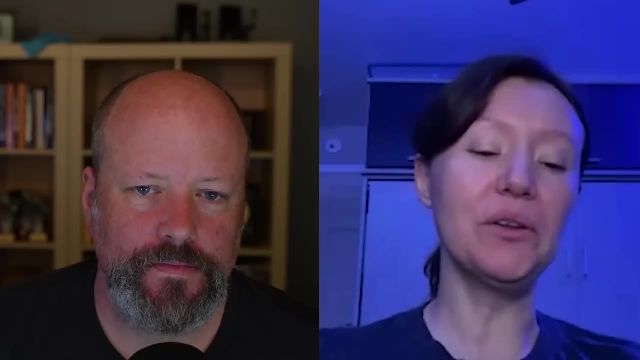 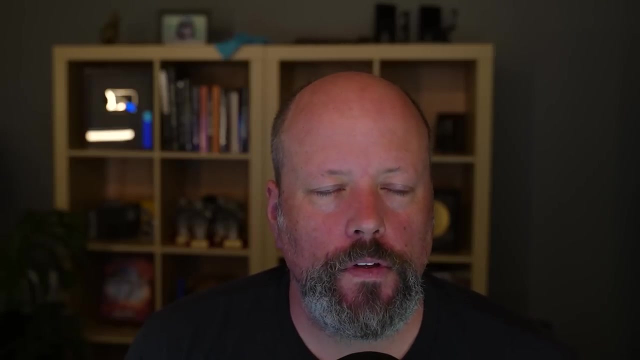 I was like I like Hubble and JWST. Now I just get really lost in exploring all the the beautiful pictures that come down from them. Yeah, yeah, So and so then you. so you worked on this project for the European Space Agency, So 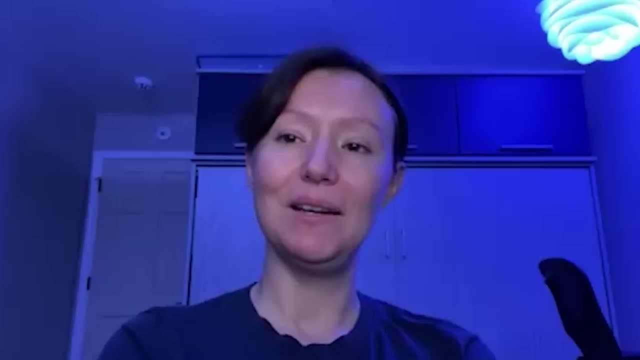 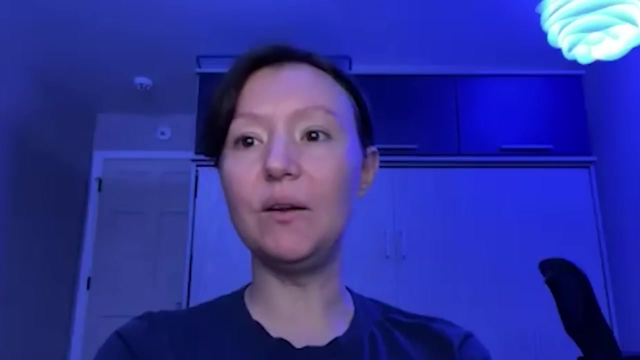 what? what were they looking for you to create? Well, it was a contest, So they just wanted people to go into the archive and find things that were never posted publicly as an image release by them, or, you know, Space Telescope before. 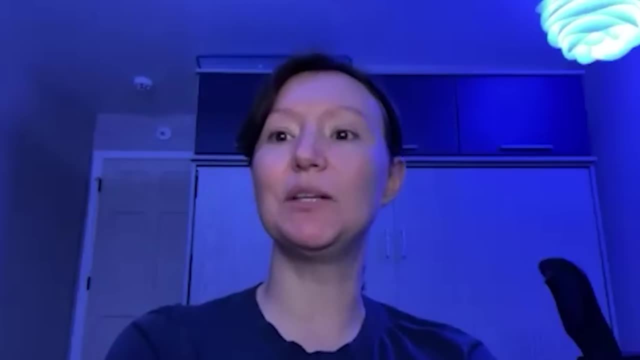 And I won third place. There were obviously some other people who knew what they were doing better than I knew at that point because I had just started. Some other people who had joined in. they had already done some processing and they kind of knew how to. 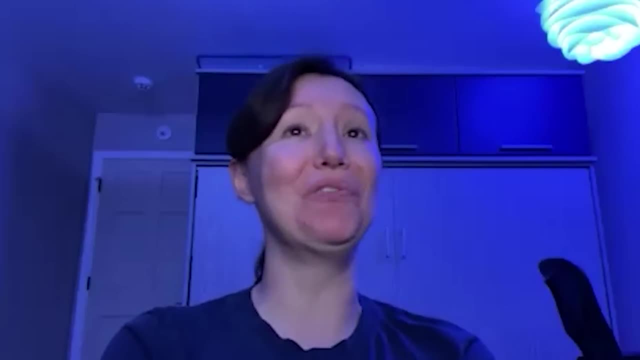 like look for things in the archive. And I was like the first thing I did was I'm like I'm staring at the search bar. I'm like what do I even search for? Yeah, So I typed in cat, I like cats, Okay, And for something actually came up when I searched. 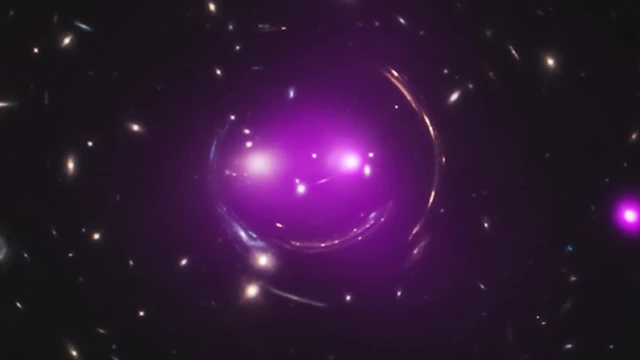 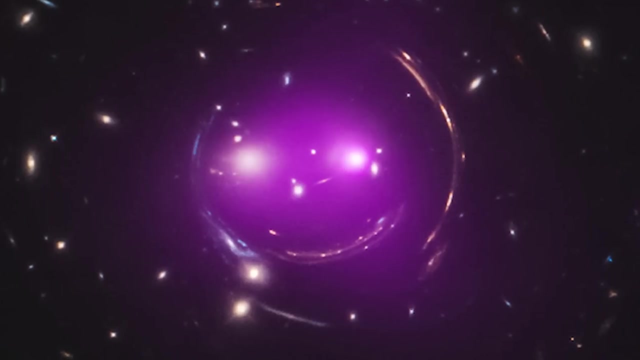 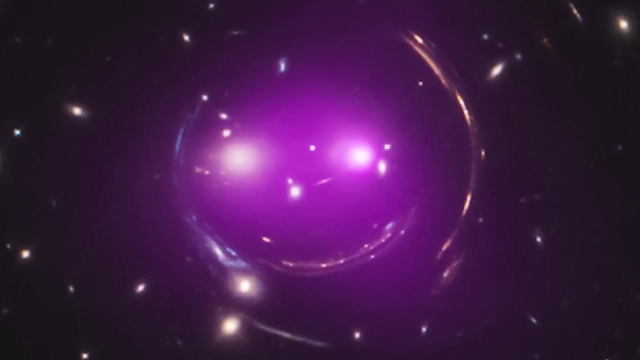 for cat. I didn't think it would, but it did. It turned out to be that Cheshire cat- gravitational lens- Yeah. So cat actually pulled up the Cheshire cat And that actually eventually turned into a semi-famous. It turned into my famous like gravitational lensing system because it does look like a 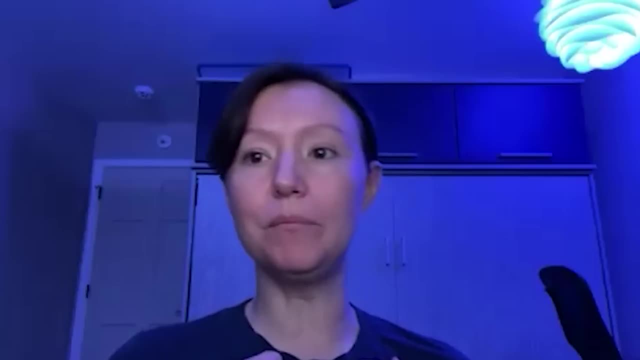 smiling face in space. CNN even posted it- Not my picture- but later on, when I think ESA did a version, they put it up and it was way better than mine because, I mean, that was my first ever picture. Later on I did redo it And, like the redo, I'm like super. 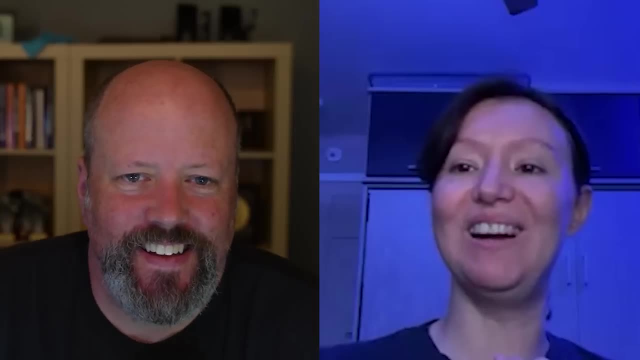 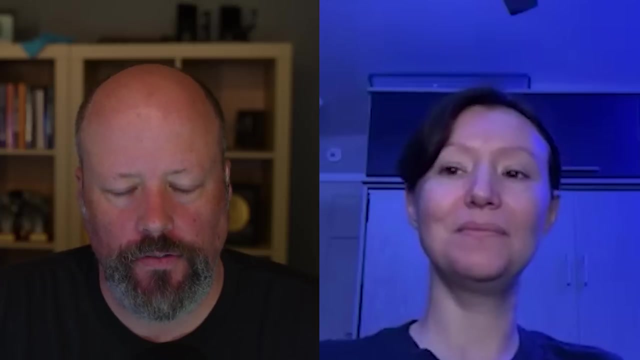 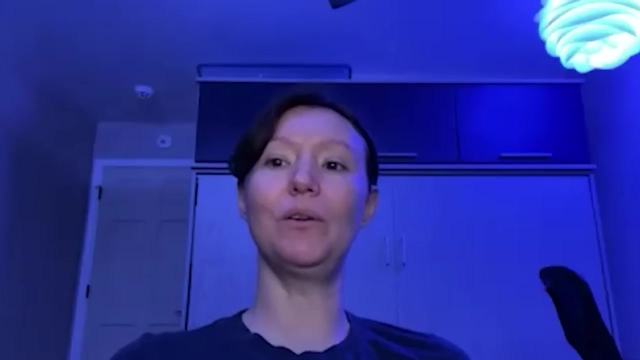 happy with, but you know it did not. it did not gain any fame. Yeah, Yeah, It's there. What was your experience with image editing tools, working with astronomical files and so on before that? I was very knowledgeable. I've already been working in Photoshop ever since, you know. 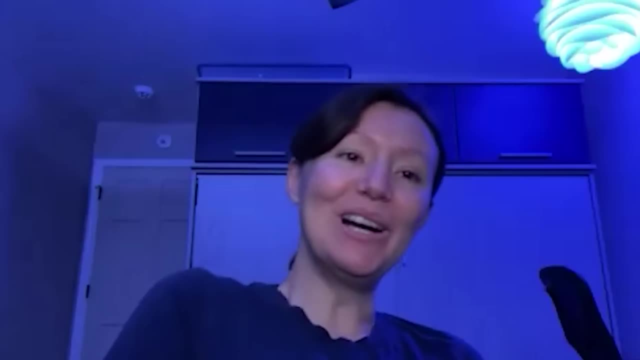 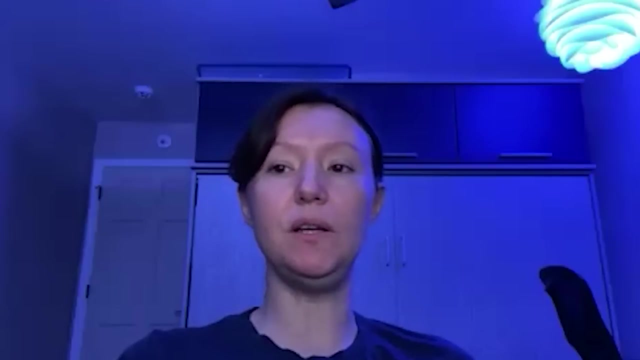 I was a high school kid and I could pirate the program. Uh, they'd been putting public images of, say, from the Mars rovers or Cassini for a long time And I kind of knew about those. but that's even a different file format. But, yeah, I didn't even know how to do those. 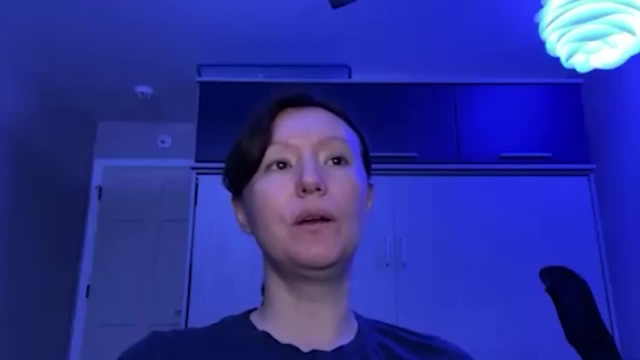 And I feel like those programs have a much more robust following because of the way they do their image releases And meanwhile, uh, like Hubble, it just kind of silently goes into the archive. There's no website. that's like: okay, this is up here, now You can go. 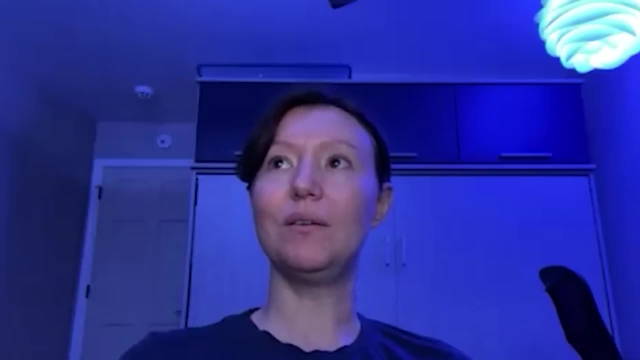 get the data, Yeah, So you just kind of go there on your own and find it and you can set up alerts, but that that's I mean. it's not like an alert that will tell you there's new stuff. It's like you have to know you have to go find something that's already been image and 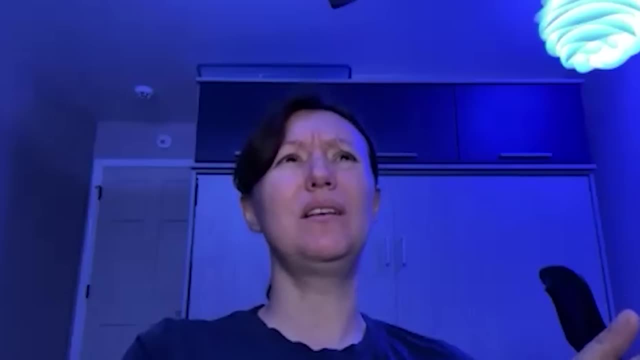 or scheduled. I think there's some data, BSC things that end up in there that are scheduled but not actually observed yet. I mean I don't know. but anyway, once it's there and if it's not public, you can say, okay, send me an alert when it does go public and you can sort. 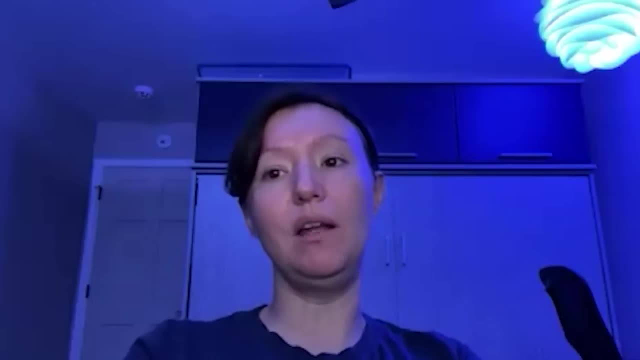 of like get right on top of it then. But yeah, there's no public outward facing, not even a a Twitter account like a bot that will say: Hey, this is our new couple picture. I think somebody set up one for JWST. 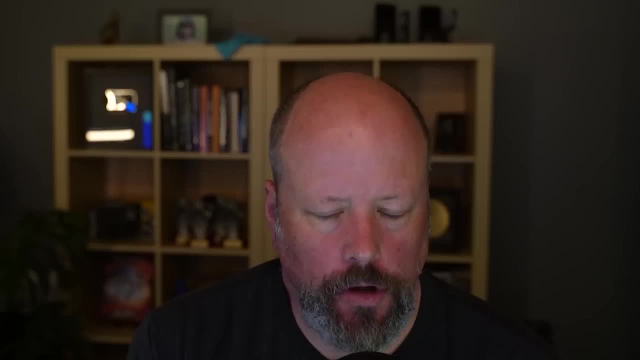 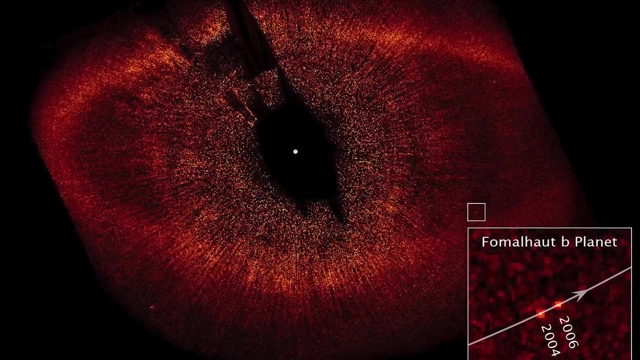 There's a, there's a bot that tells you what Hubble is looking at, what the target is. Yeah, And web will release a schedule of all of the targets for the week. So this week, while we're talking, they're imaging a formal hot which is a star, the eye of Sauron, star that. 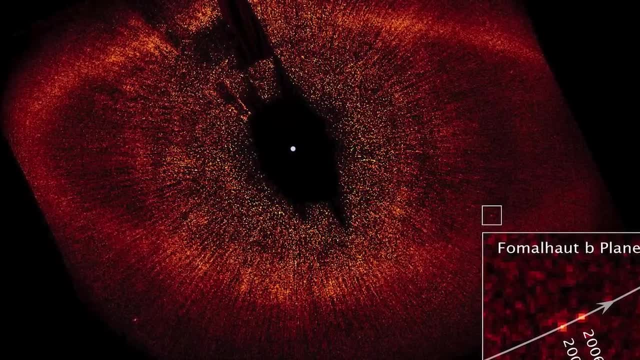 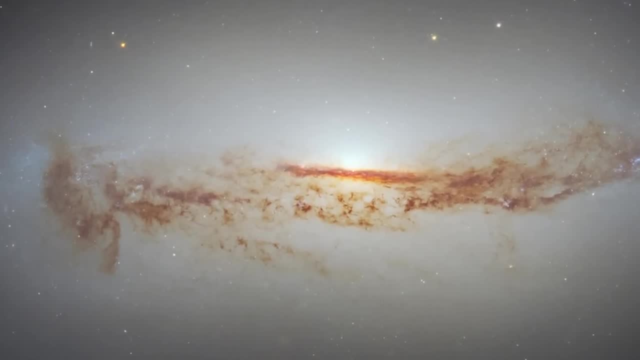 people have probably seen And they're also imaging like a brown dwarf, and they're imaging a pretty cool galaxy that Hubble has taken some pictures of edge on And but we won't see the data for those for another year. Right, right Yeah. So you kind of have to put make a mental note: 12 months from now, come back around, dig that data out. You can go in the archive and like, select them all and then say let me know when these go public. But yeah, you have to go in and do that first. 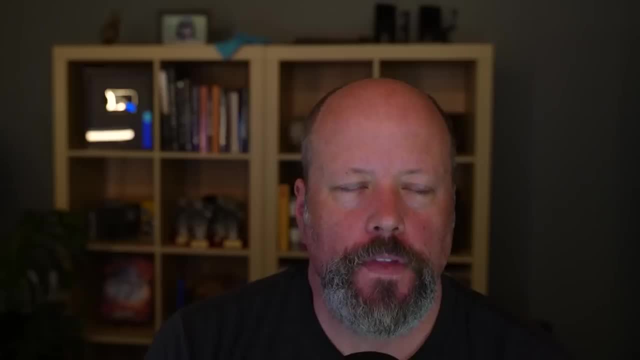 It's hard to explain, but I guess, like my job is as a journalist And so I have become very familiar with the way the machine runs- where a researcher puts together a proposal to NASA, to or to the folks the at the space telescope science Institute, they get time. 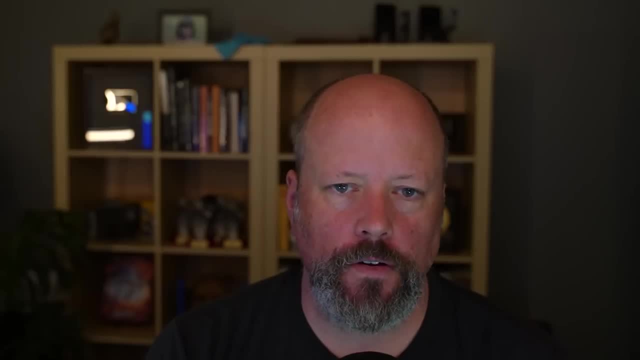 on Hubble. they do their research, they get their data. a year later or at some point, they write their paper. they publish the results. Someone at their university thinks that's cool and wants to write a press release about it, And if they're lucky, somebody knows what. 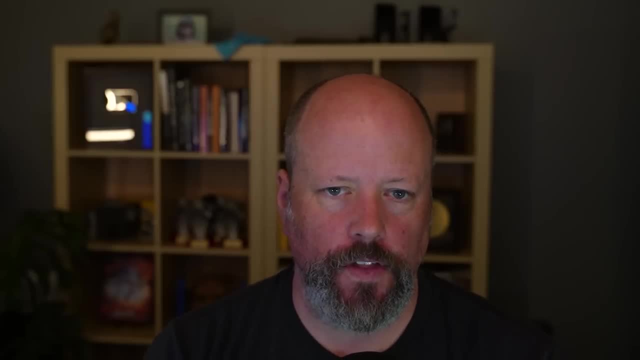 they're doing with images and is able to pull out some interesting images out of their research work and and and attach it to the paper, And that might help them get more, more results, And then and then, at the same time, they're. 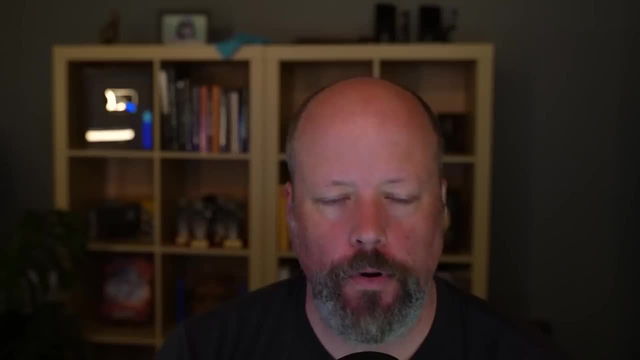 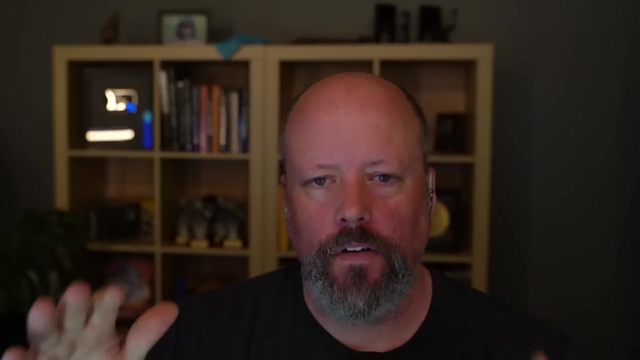 they're going to, they're building their various, their magazines, They're they're going to publish a press release, And then they're going to make their own press releases and get the readers to write them down, and so on, And I think that's a really good thing. 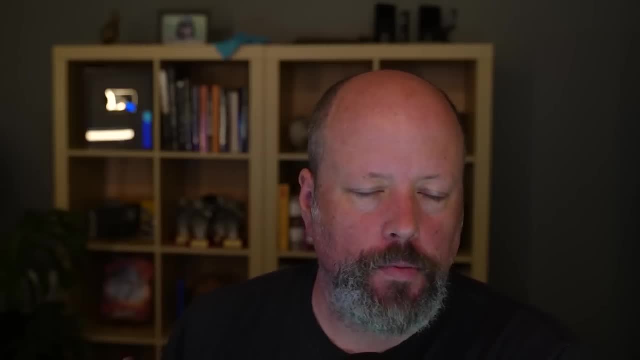 Yeah, Just some of the. you know the. the first thing I'm seeing is a lot of people are releasing something called a web of images like that they're sharing to them, And I think it's a pretty cool thing to see. 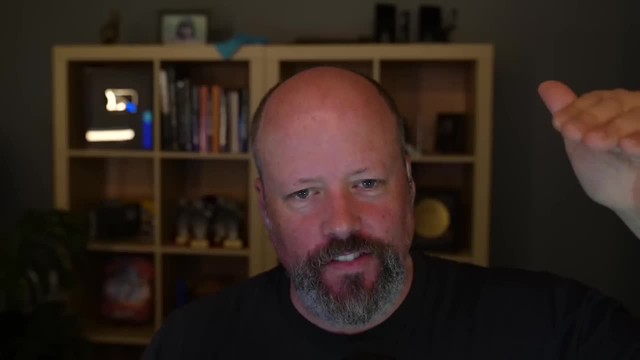 Yeah, Yeah. You see here there's people at SDSI who do image processing when they find really cool pictures, And they'll release those as press releases as well. So you you kind of have these two trains of of images that are coming. 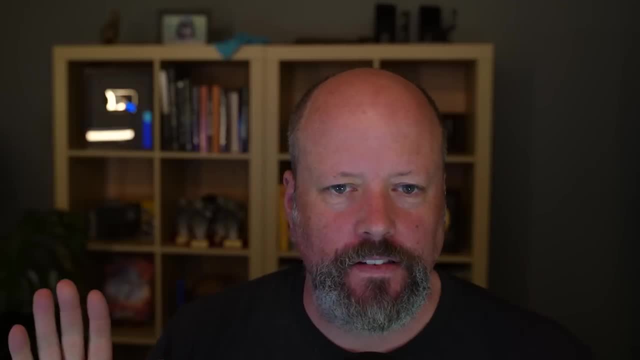 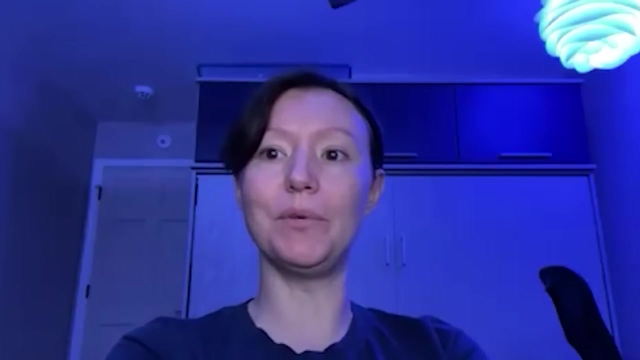 Looking through archive data that in many cases, nobody has looked at beyond writing a scientific paper about it. with an artistic eye, The astronomers themselves. they're always paying attention to their favorite topics and objects. So yeah, but that's a relatively small circle. 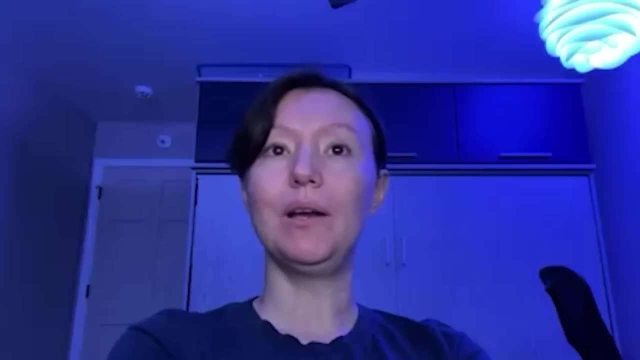 I mean, arguably it's the most important people to look at it. But my favorite thing is I'm not even looking for what they're looking at necessarily, Like I have a very broad interest. I'm not super specific, like, oh, I want to look at just AGNs. 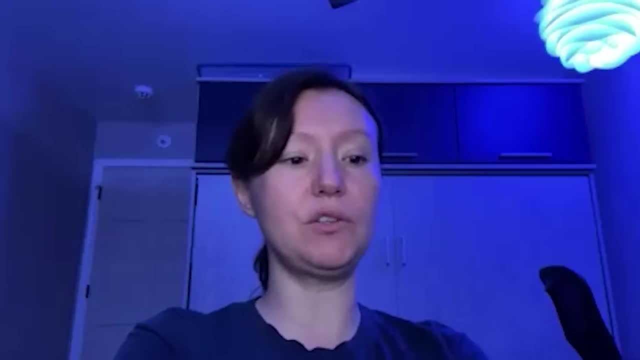 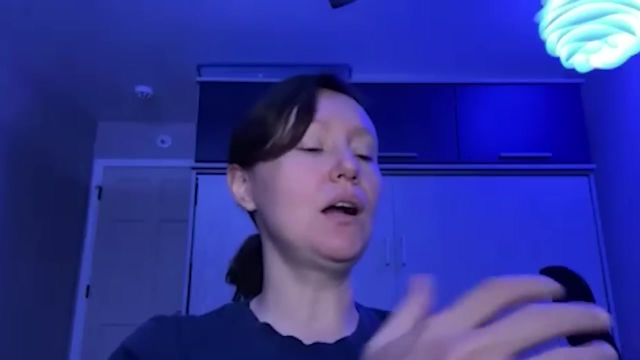 I want to look at just planetary nebulas or just newly forming stars or just planets or even one specific planet. I'm just like I'm going to look at an image and whatever, And a lot of times I'm pulling in old like because I want all the data right. 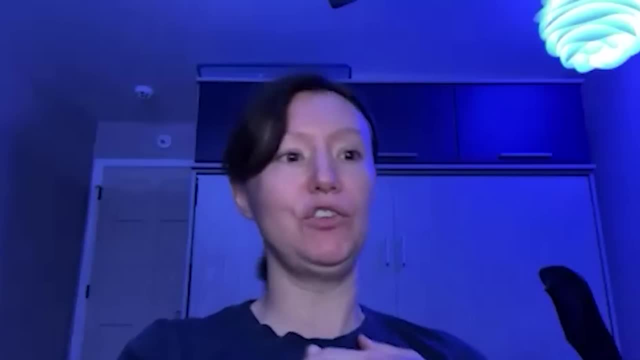 I don't just want my observations. Well, I'm not making any observations, So I have no like. I have no bias for like. oh, this is my brand new, This is my little baby that you know. I got Hubble time on. 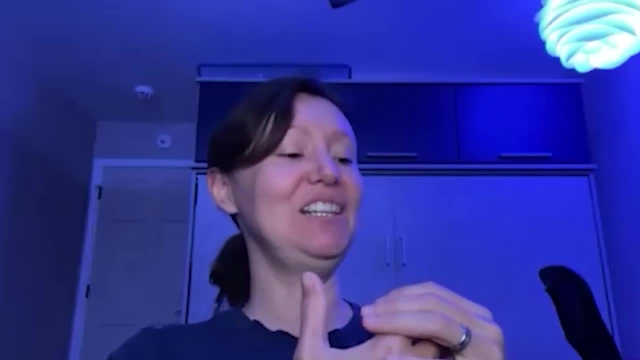 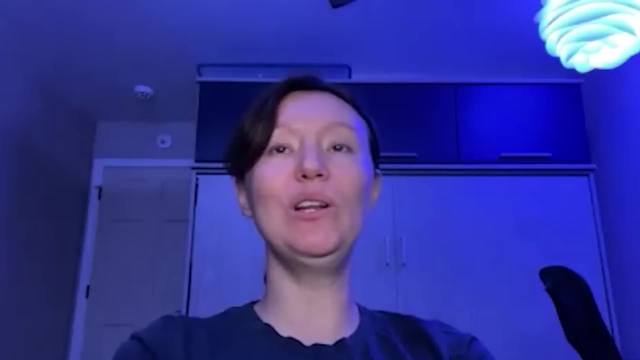 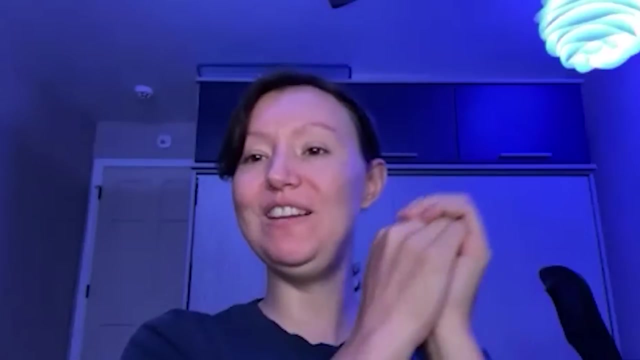 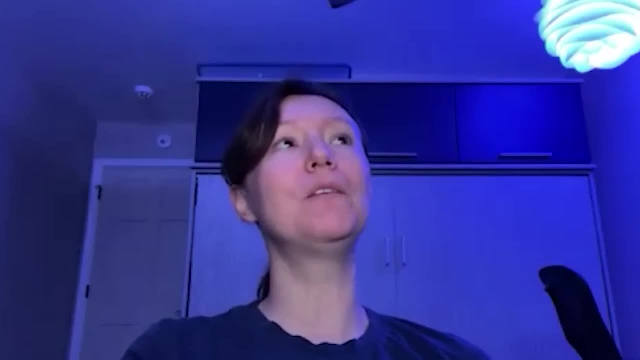 And I wish I knew more about them. But like it's proper motion of stars in the galaxy. It's funny the way, once you get to like Hubble's level of resolution, you can just see the galaxy is moving. It's not stationary at all. 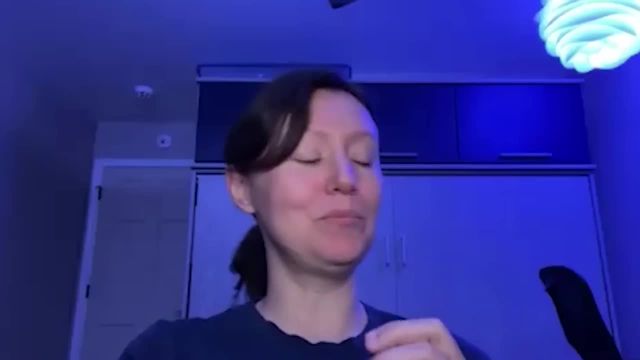 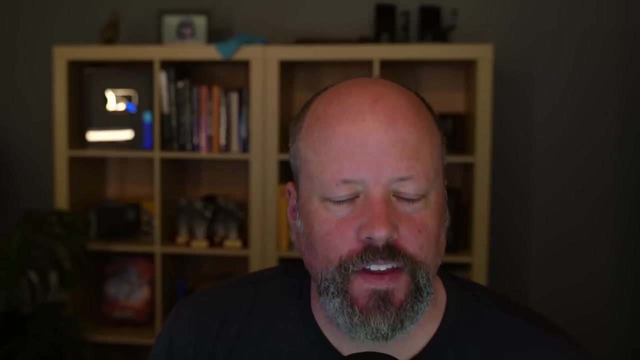 And while it's cool, it also does present- It's- some like processing challenges. If the if the star happens to be very bright and very fast moving, then it can, like really make the image look funky. Right, This was. this was an image that I saw that you had done recently, where you had had compared the Hubble data to the James Webb data. 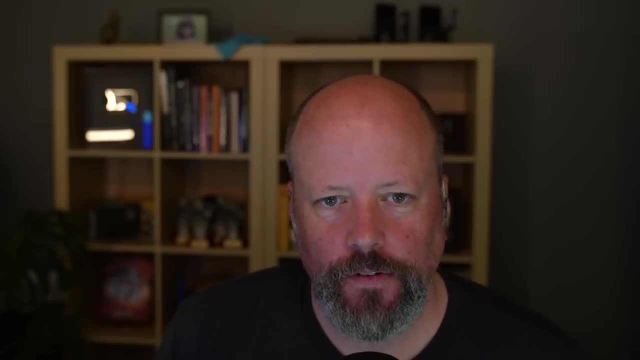 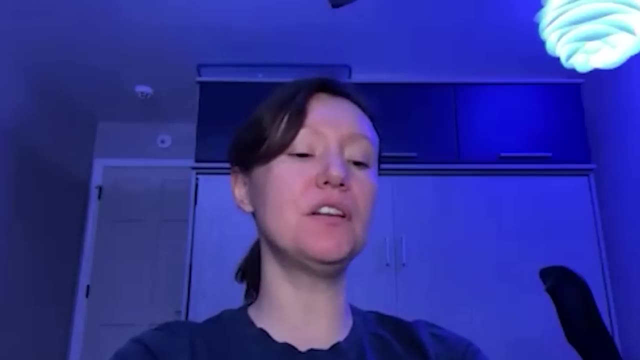 Yeah, Some of the stars had moved so much that it made it difficult to line everything up in the image for you. Oh yeah, I mean it's almost guaranteed that that If there's 10 years difference that they've moved, there's at least a few of them that have moved a lot. 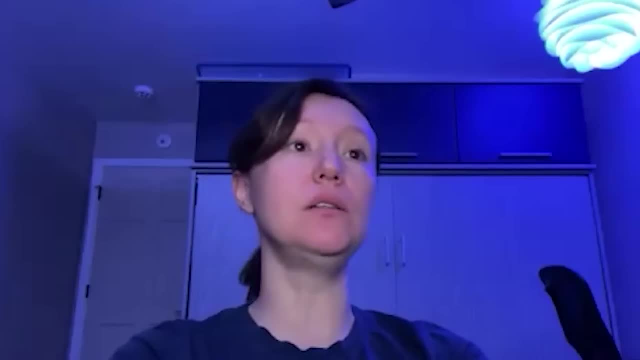 Wow, And yeah, some of them are moving so fast that it only takes a couple of years, And you can notice. I mean usually a couple of years, you're safe. But yeah, like just a few pixels makes it difficult to get really a good alignment though. 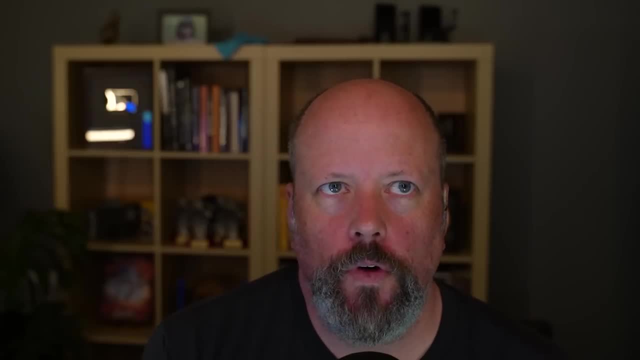 But I think about this like it's very strange to me that you'll have a researcher, scientist, who will be working on a galaxy That is, you know, subjectively very beautiful. The end, and and could be this in is- has a nice resolution. 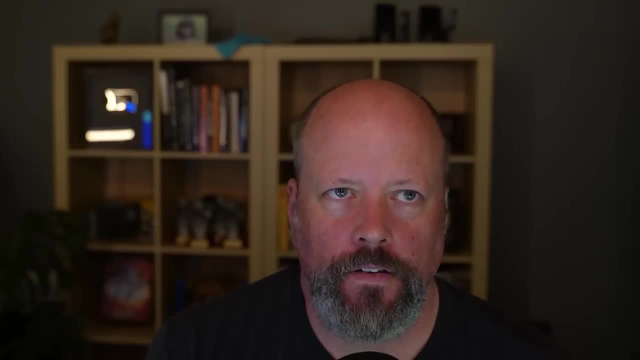 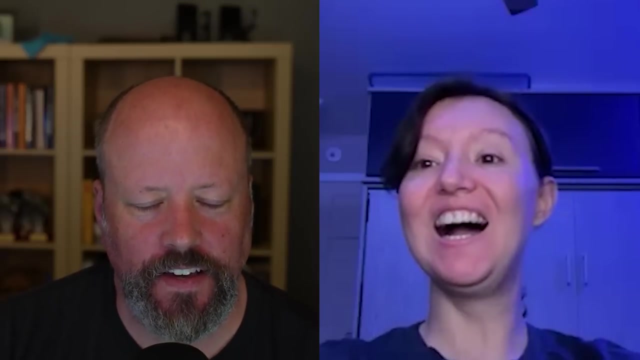 It's been captured in a way that is very aesthetic And for them, they just want the spectroscopic data on the active galactic nuclei and add it to their data field, add it to their database, So, and then move on, And and they don't spend any time thinking like, wow, that is an amazing galaxy. 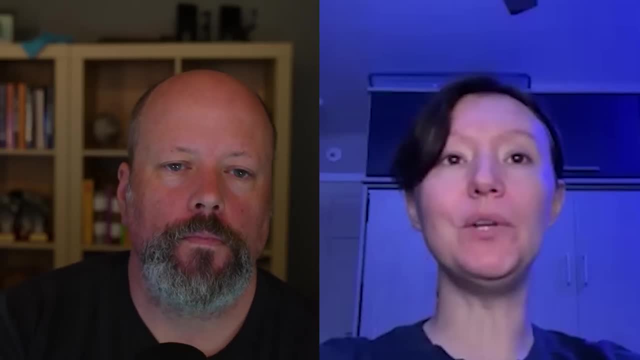 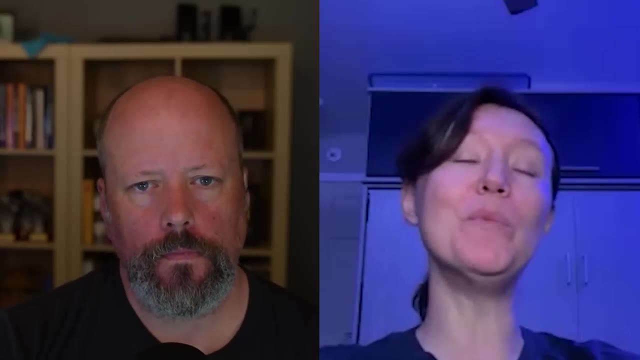 That's so beautiful, You think, Okay, No, they do, They do, They absolutely do. I think there it would be a very rare astronomer who doesn't actually take a moment to be like oh wow, You know, because that's kind of like what gets them into it. 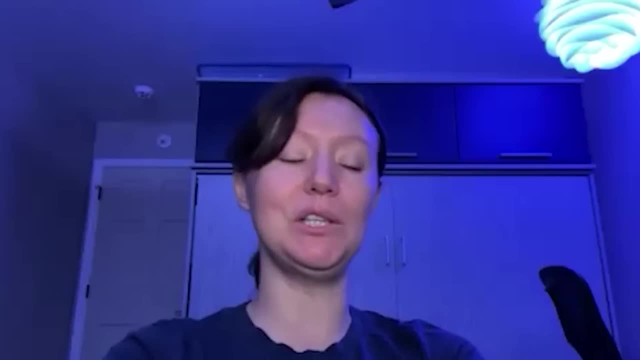 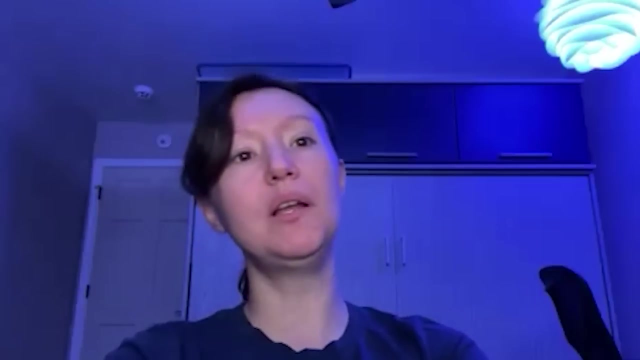 And, yeah, there's the. well, I really just need to get get this paper done and get these measurements taken and do the science. But they, they tell me, you know, like I just didn't have time, They don't have the resources, they don't necessarily have time to do it and do it beautifully, like they can make something pretty quick. but you know, they're not going to be like me where I sit here and take the image and be like, oh, this is a cosmic ray. 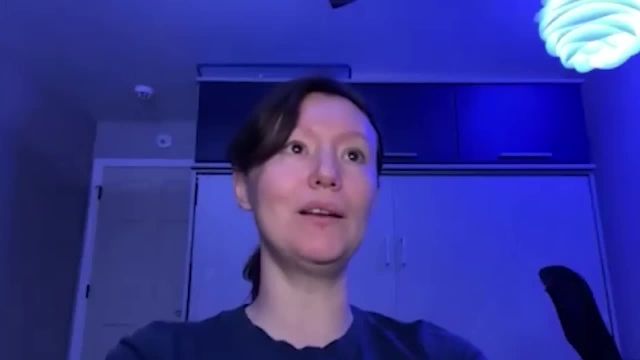 Oh, here's some stray light. Oh, I got to match the background and get it all nice and smooth. So, yeah, I feel like I can really fill in that, like there's a need for it, And I've, Of course, made that YouTube tutorial on processing Hubble data with with Photoshop, and I I've actually gotten quite a few people to start doing it too. 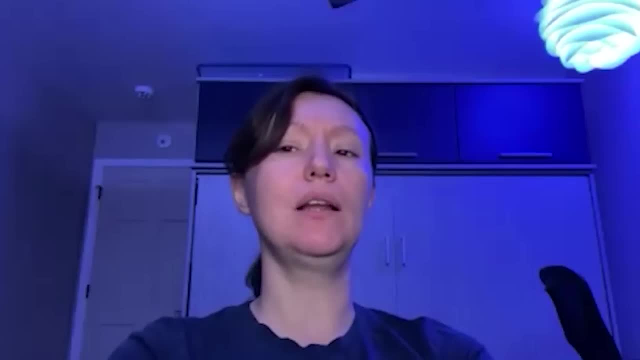 And since JWST came out, I feel like like there's there's even a few more who just got interested. There's like some guy I didn't even I didn't even know until now, But I don't even know who he is. 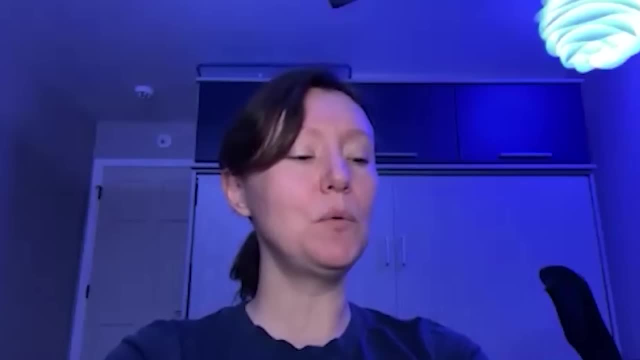 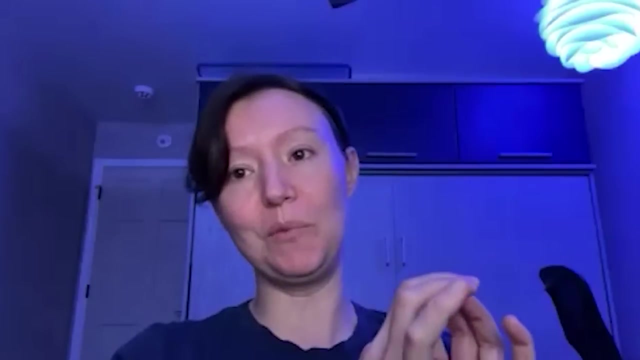 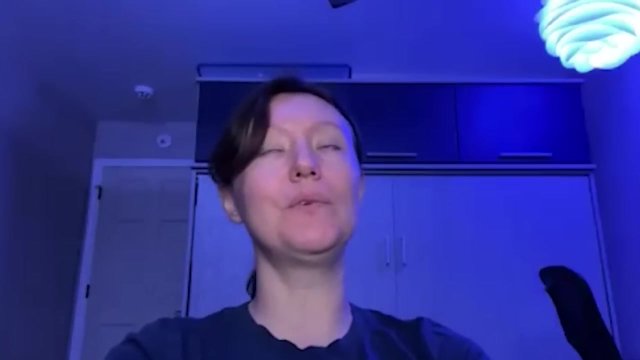 But he's, he's, he's been processing it with, I think, on a Linux system, And I was very surprised that he's writing his own scripts to try to like fill in the stars. Yeah, Which I will explain. stars put like the bright stars, have like a black circle in the middle because they're, they're overexposed and whatever, for whatever reason, the pipeline is, instead of making it bright, white is. 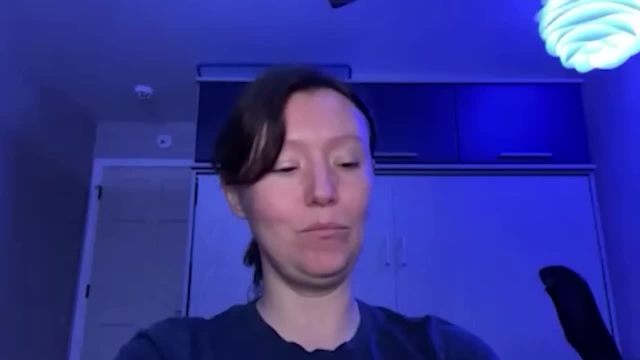 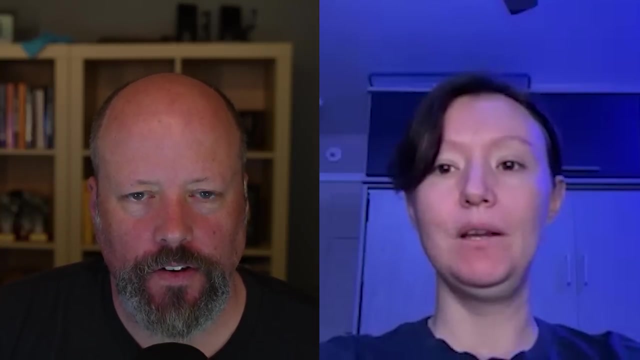 dropping that one hundred percent white down and making it black. sort of black. It's not even one hundred percent black, It's like blotchy. It's really, it's really annoying to deal with. Right, Because you have to. you have to decide like: are you going to try and swap them out with a lighter color, and what color? 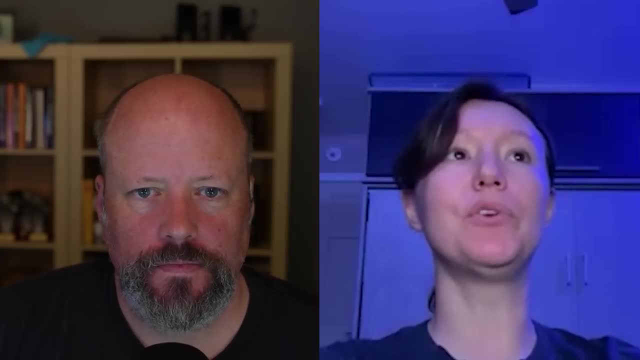 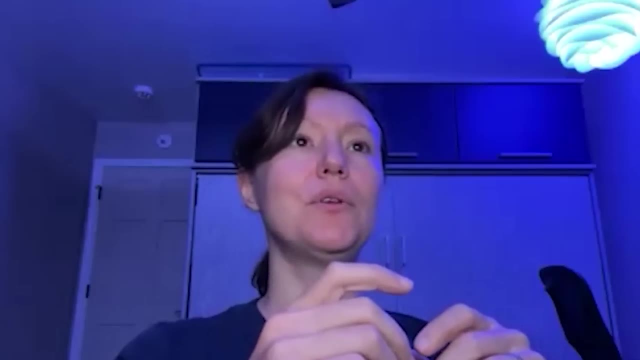 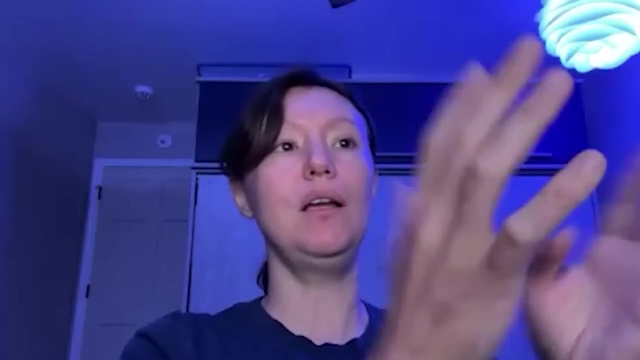 And well, I mean, obviously I need to fill it with with one hundred percent white. It's just going to be the most aesthetic choice. But because it's sort of fuzzy, I can't just use the Magic wand tool to automatically select all pixels that are at zero, because it's not all zero and there's this fuzzy edge around it. it just it's annoying. 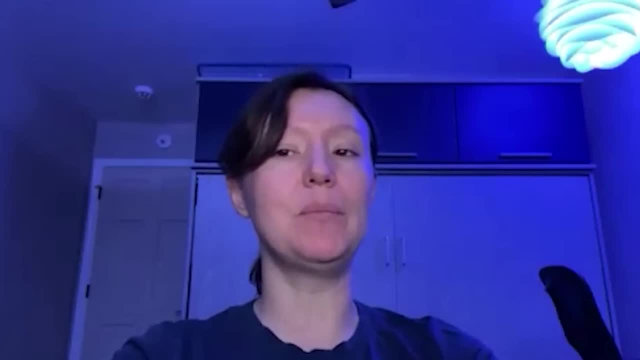 And I'm like: I hope, I hope the pipeline gets better. I know they're working on it, but aesthetics are probably not their number one priority, So OK, so I'm going to, I'm going to rescind what I said completely. 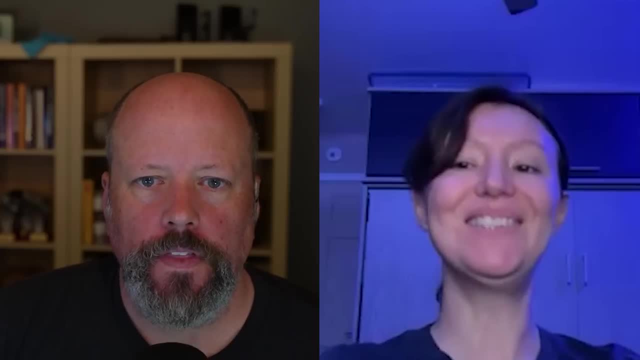 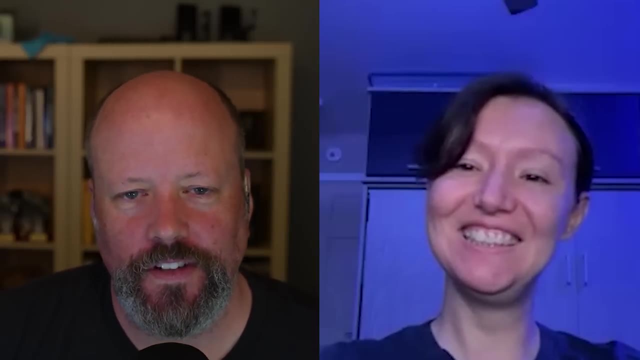 So the astronomers Know that these things are beautiful, right. They just don't have you in the course, of course. Right, It is. it's. it's like I don't know an ecologist in the middle of a forest every now and then stopping just going. wow, this place is amazing. 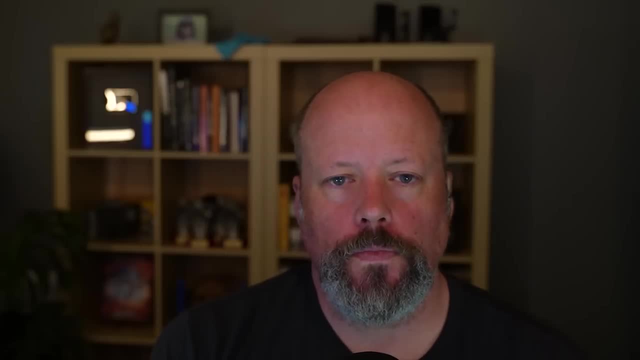 But they don't have the resources. They don't have either the skills to to bring this, this image of a galaxy or a nebula or a planet or whatever, to the level that it could be, And they don't have the time. there They're trying to gather the data. 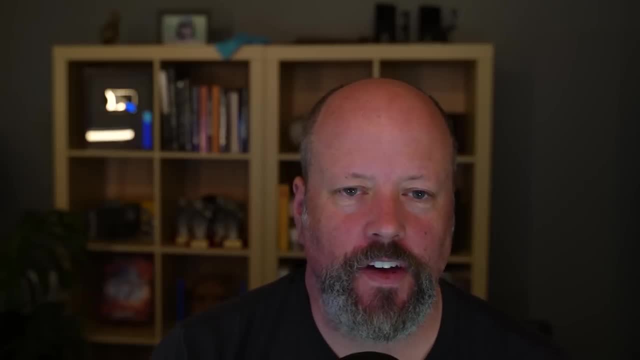 And then they got to move on. They got to, they got to attend the department chair meeting and they got to seek funding and they got to talk to the public relations and they got interviews with me and they don't have time to sit- Yeah, they don't have time to sit down and and process these images. 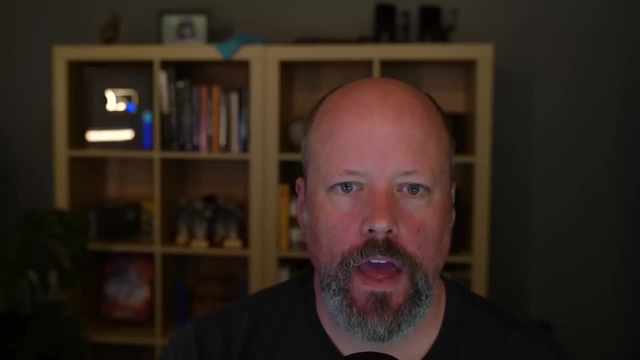 And you can swoop in and you don't. you're not trying, You don't have to be at the department chair meeting, You're not worried about the science. You're there to say: how do I make, How do I make this wrong? 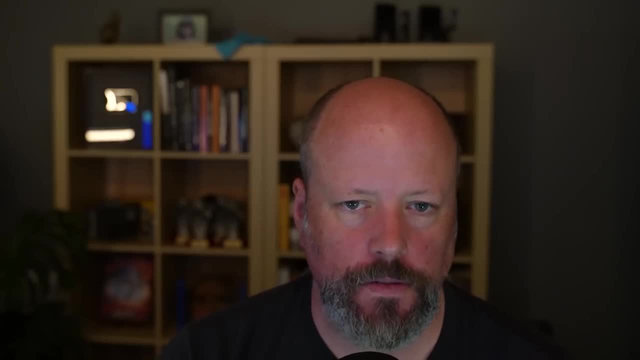 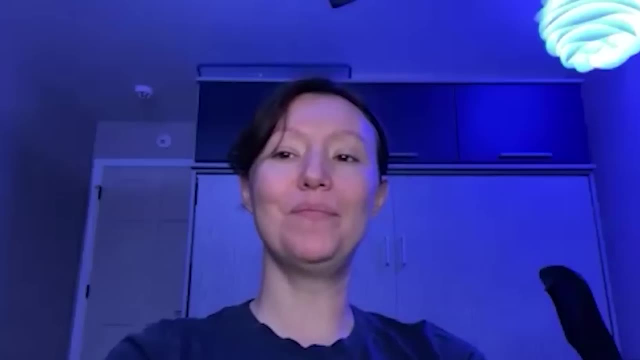 How do I draw data into something as beautiful as possible? Yes, exactly, My biggest worry is my baby coming in. That's actually like I have had like so little time of just like where I can just get you know two hours, two hours would be good. 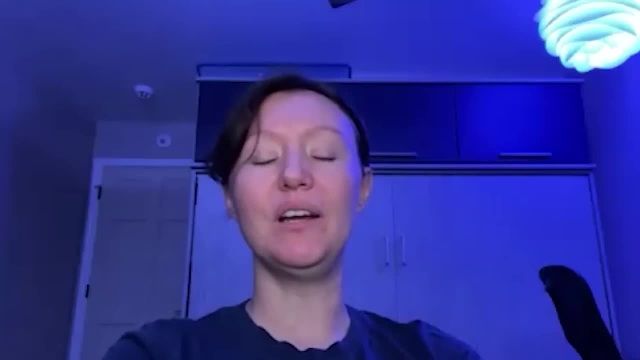 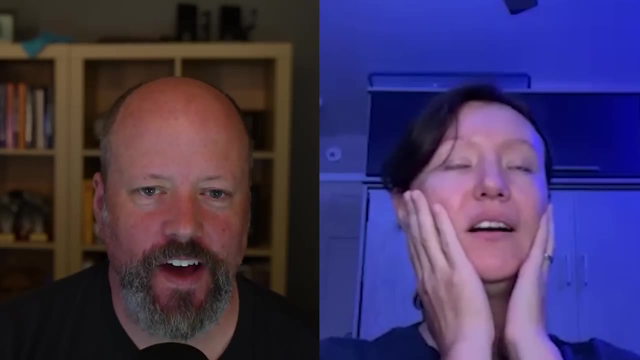 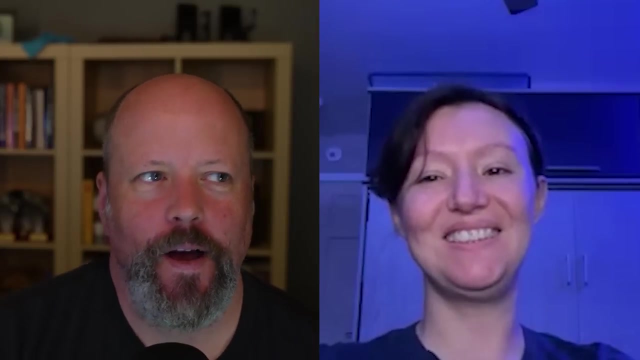 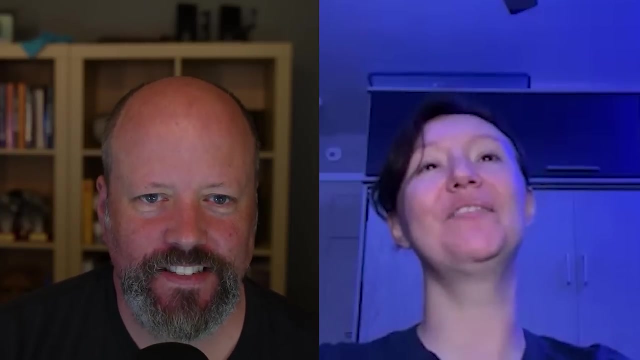 He comes in after about 30 minutes usually And I just feel so interrupted It like it just it. Both of mine have moved out and now have, you know, apartments of their own. So you know, enjoy. I'm sure people always tell you like, enjoy the time while you can, because after a while you sort of you know you have a lot of time on your hands. 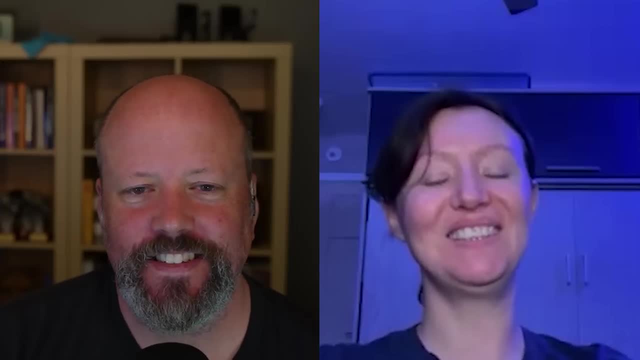 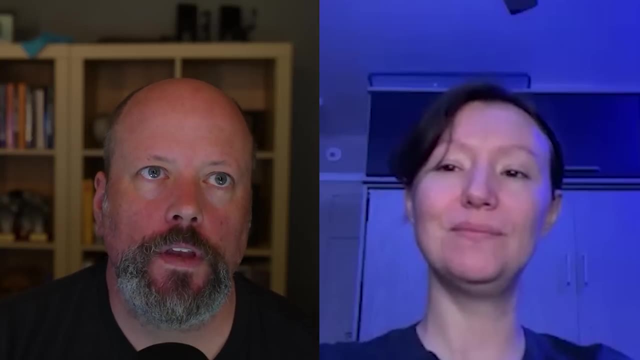 Yeah, I'm 13, and then you never see them again. So that's you know. you've only got another 10 years to go, or so until that. until that moment, Yeah, But, but then OK. so So then, what is the process? 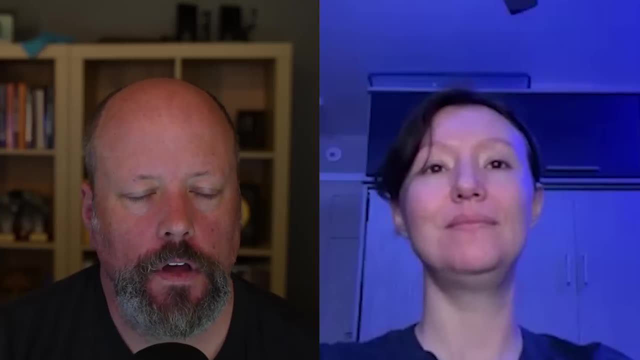 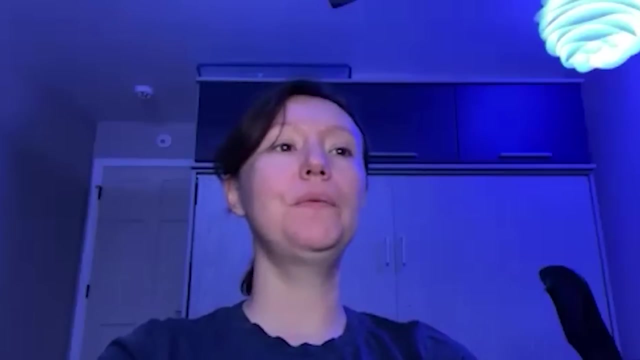 Like, how are you Searching for images for Hubble and I guess now for James Webb and for maybe other telescopes? There's a few different ways. you can go kind of random where you just say what was Hubble doing in 2003 in the month of June. 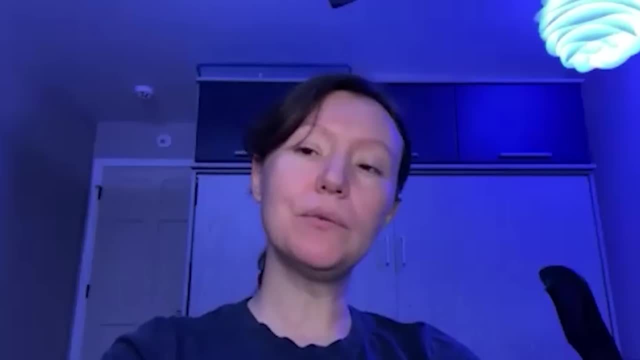 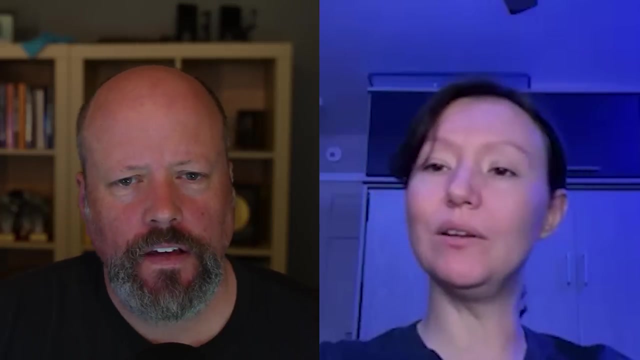 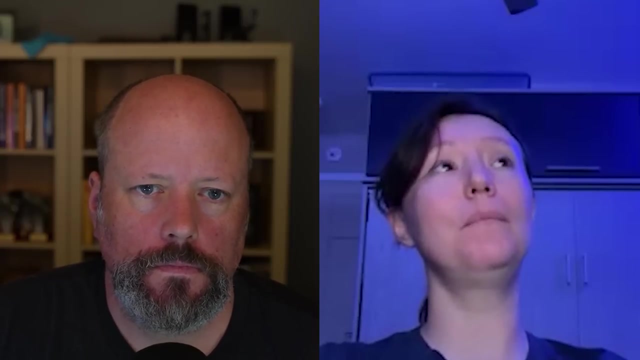 And just look at everything. you know. you can filter out the spectra or the, the calibration images and just scroll through And you can do some thumbnails, anything. that is that easy. Are there thumbnails, or yes, OK, OK. So actually, when they first put the MAST website up, I actually like they were looking for feedback and like: can I give them feedback as a non astronomer, random person? 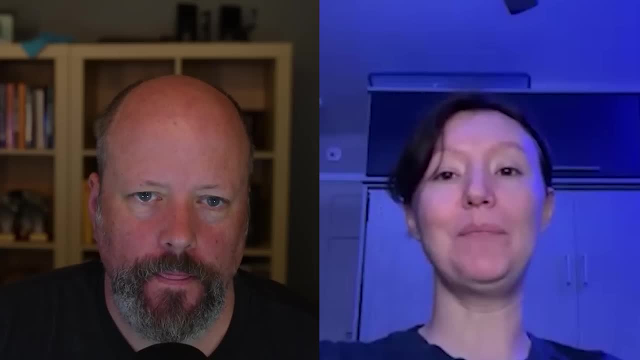 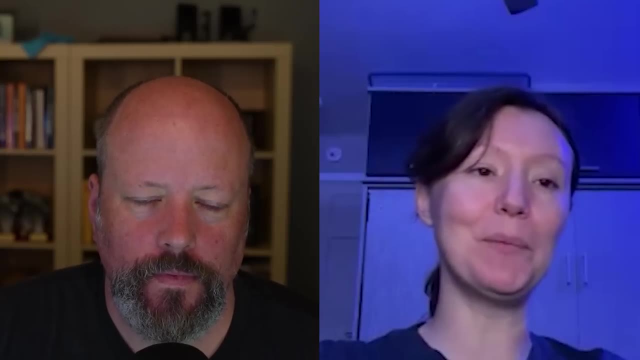 I sent them and they're actually like really like happy, happy, like happy to treat everyone equally. I think, And even though I'm just as I feel like I'm a random person, other people are like: no, no, you're an astronomer, you're, you're, you're, you can, you can. 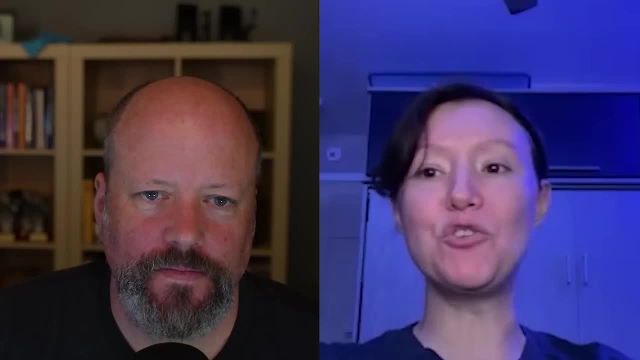 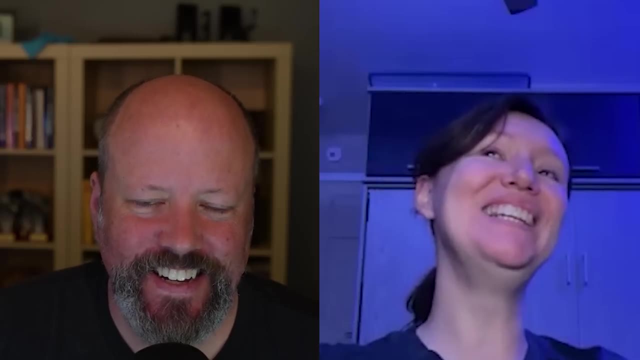 But anyway, I always feel like an outsider and like I'm intruding into the astronomers world. But I actually complain. I'm like I need the thumbnails so badly, They need to be there, And they actually put them up, like I think, a week later. 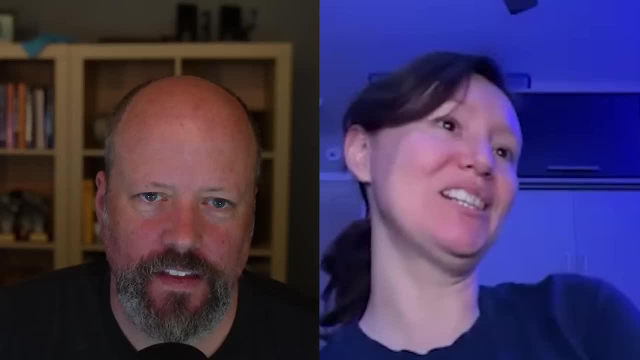 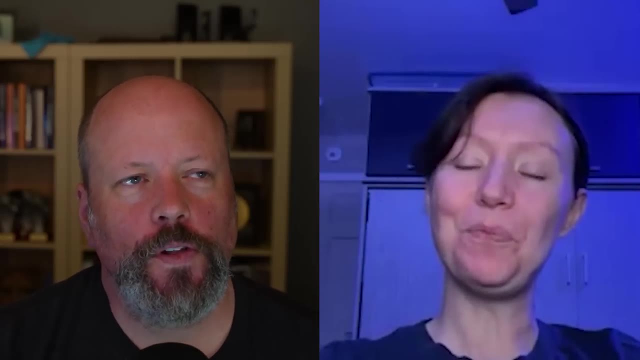 Right, It's probably already planned or something, But I just kind of gave them a little- Yeah, Bit of motivation. maybe I don't know what. I must have looked through them before that. Yeah, because I was following your tutorial and and looking through the data on the James Webb server. 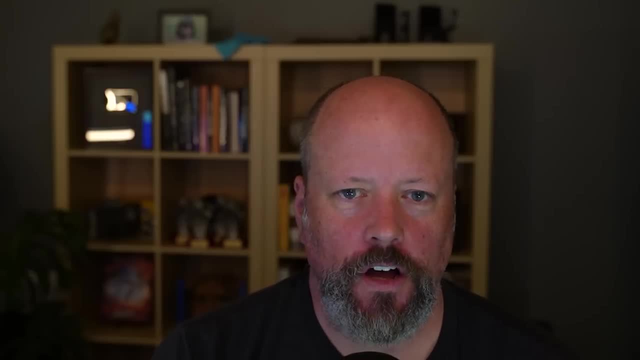 And all I could go by was my knowledge of what an object is to go. OK, that's a galaxy, that's and it's, and it's a galaxy that's only 30 million light years away, So it's probably a nice picture. 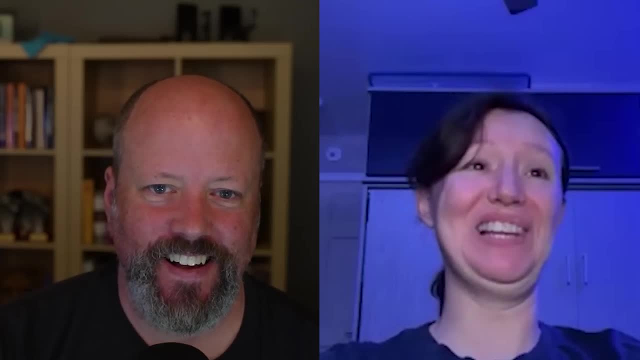 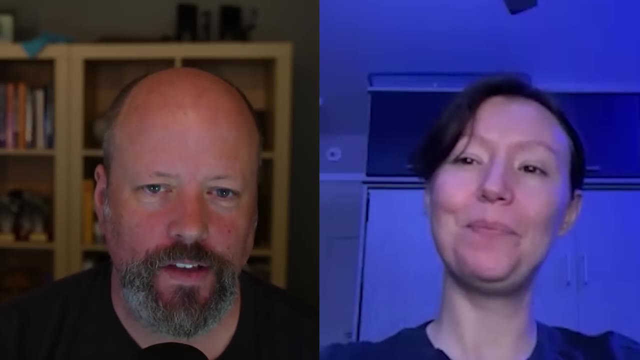 While that's a quasar, probably like a zoom in Of like a teeny little piece, Right, Yeah, it's a part of it, Yeah, it's a part of a galaxy, It's going to be nice, But, you know, while that object, that's a quasar, and so it's just going to be a blob of light, no matter how high resolution it is. 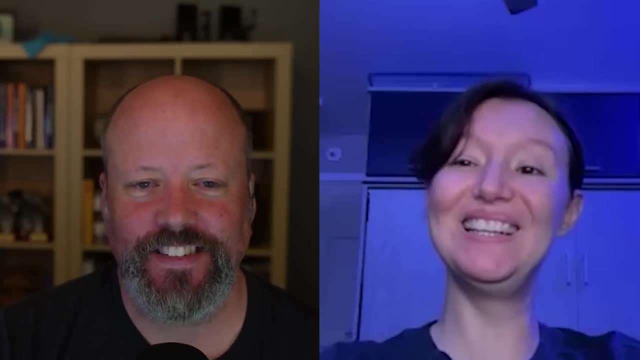 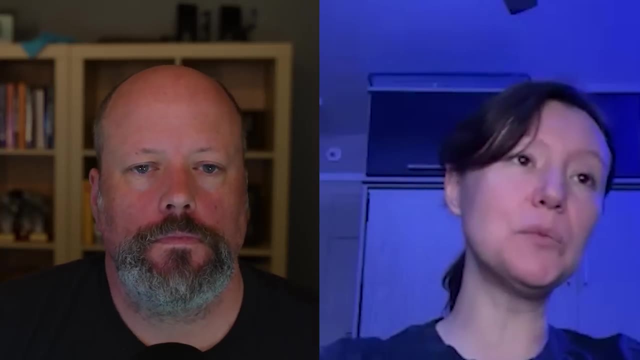 About that. Well, that's the thing. you don't know until you actually sit down and you take the time to look through it and start to tease in the data. Yeah, So with the quasars and space telescopes, like yeah, from down here with a little telescope, all you're going to see is that point. source. 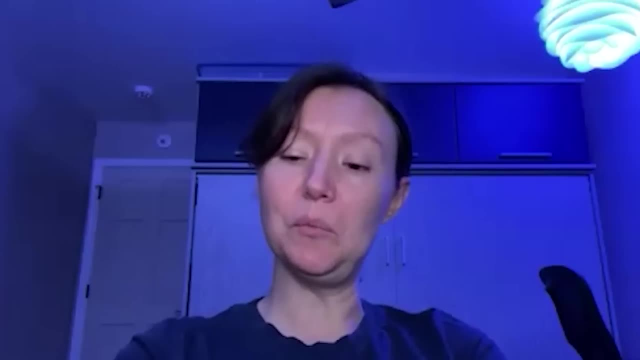 But With the space telescopes and they're, you know, massively good resolution and no atmosphere to deal with, a lot of the time you can see their host galaxy. It's pretty cool. Huh, Yeah, OK, fine, Fine, Quasars are interesting. 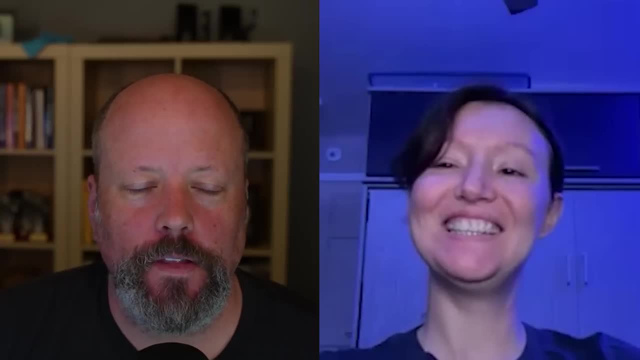 No, no, it's fine, It's fine. The point is like, I guess the point is: you can't see the thumbnails of the little of the little objects. but now you can, Thanks to you, You've you've encouraged them to provide thumbnails. 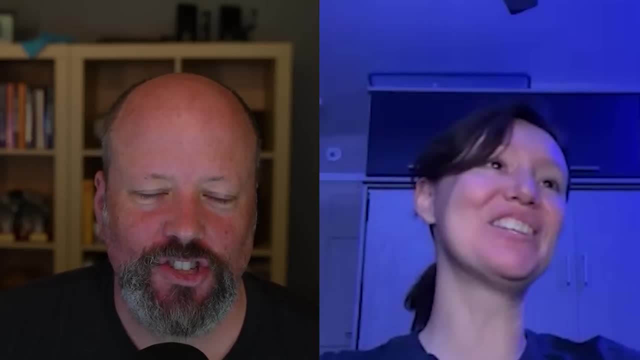 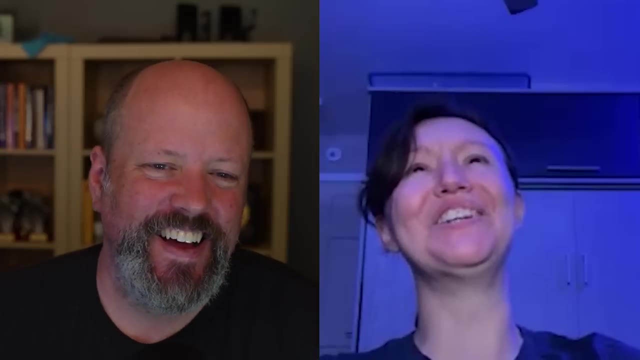 I don't think it's thanks to me. I think they would have put it up eventually. I was just sure. I just remember that day when I emailed them and I was like I need the thumbnail, please, Please. This is so hard without them. 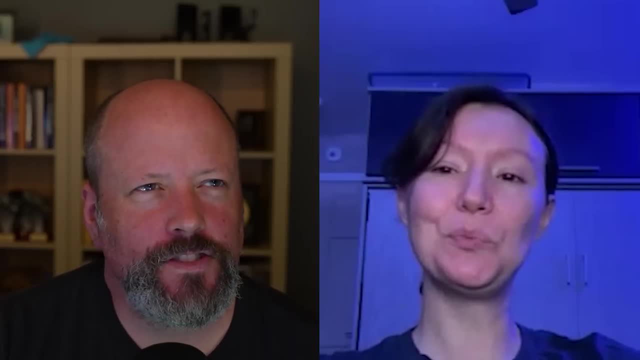 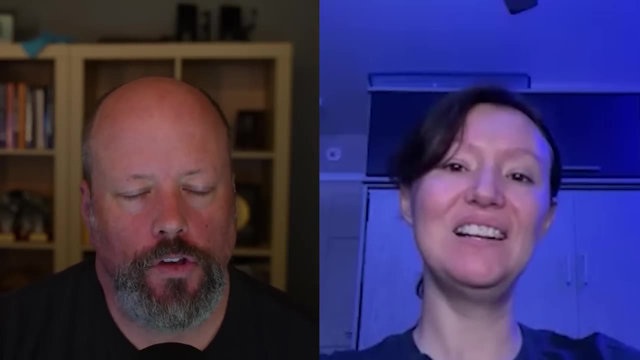 Yeah, Yeah, HD 614.. Like, is that a star? Is that an interesting star? Yeah, I can imagine looking, looking through that, that that data. So then you go through Hubble Archive data, James Webb data. Are there some other resources as well? 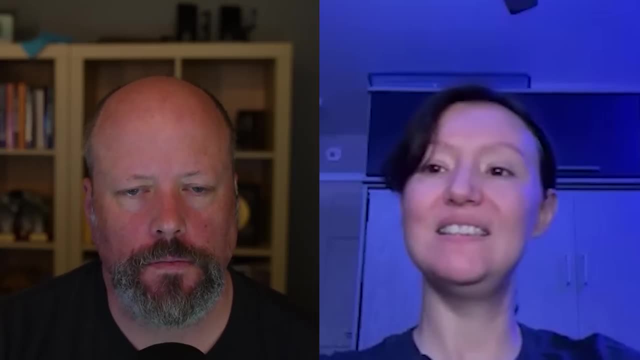 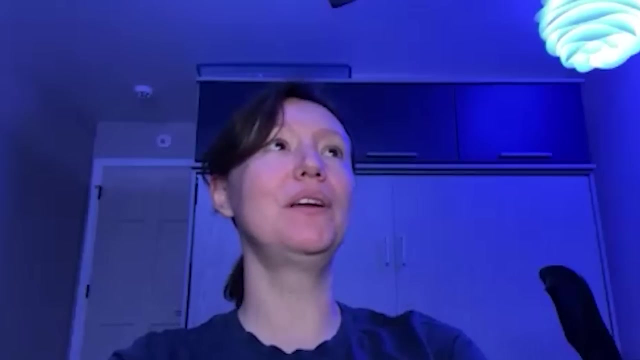 Because, like the European Southern Observatory, has a beautiful archive system as well. I don't I'm not as familiar with that. I kind of stick with what I'm familiar with. So I only- I've only ever gone to that- When I'm like desperate for, say, some color data or something. 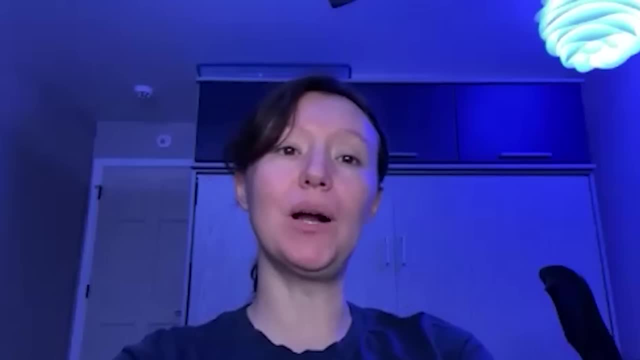 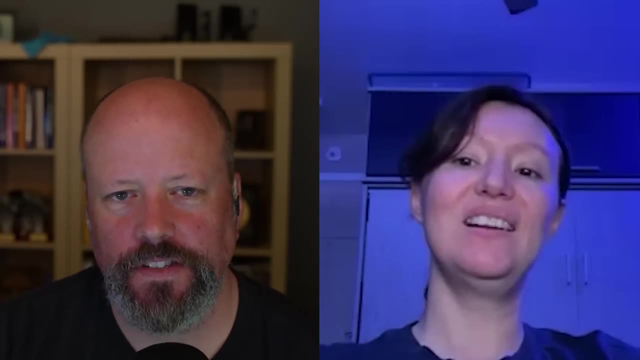 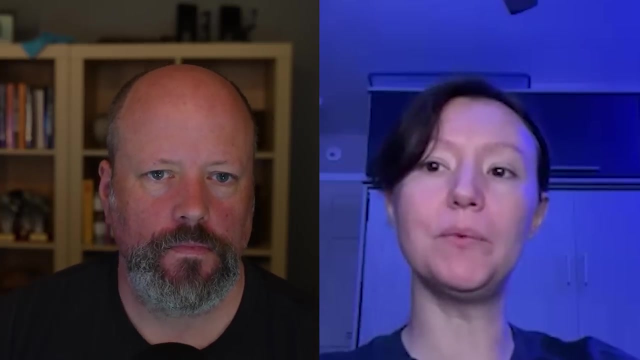 But you could absolutely search through that and probably do the same thing. There are images of planetary disks in there- Yeah, Newly forming planetary systems There. images of of exoplanet- Yeah, exoplanets. i think they do a really good job of combing through their data and getting them all. 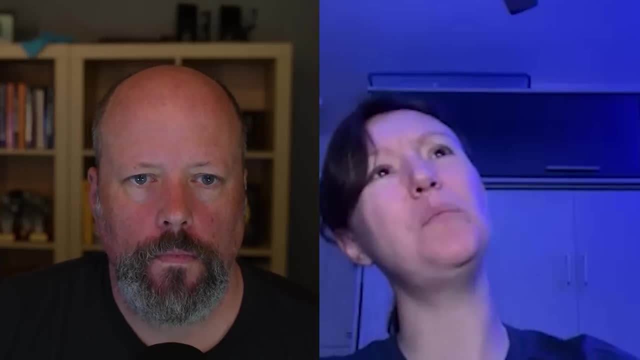 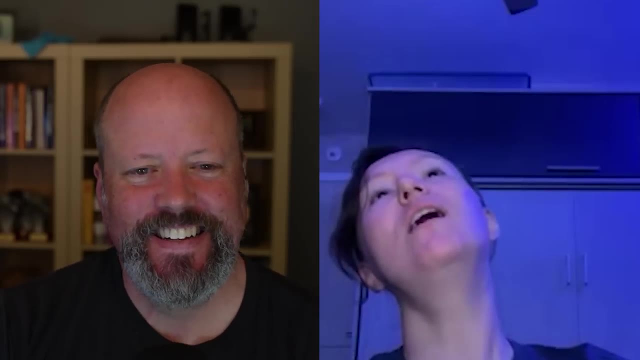 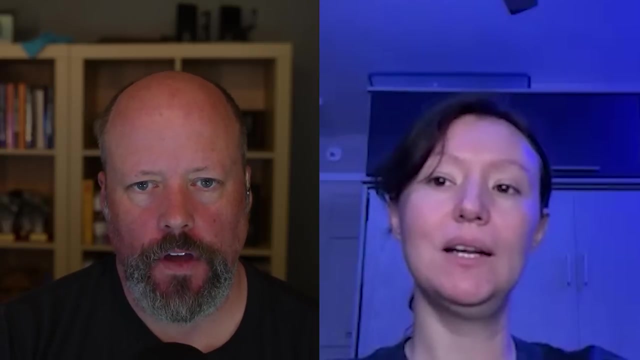 into press releases, but i'm sure there's a few in there too. i think they may have even done a contest for their own thing. i don't know. i tried using it and i felt like it was not quite as robust as the mast right. but but there is an archive for almost every instrument out there, every. 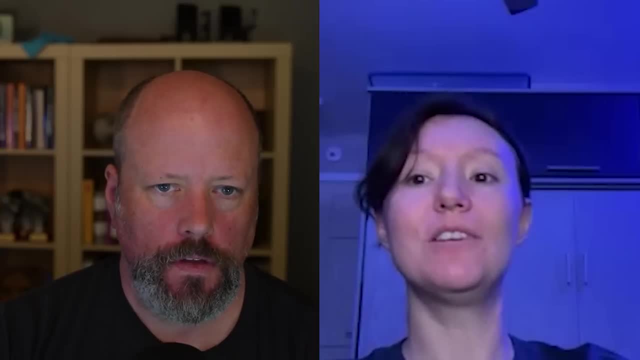 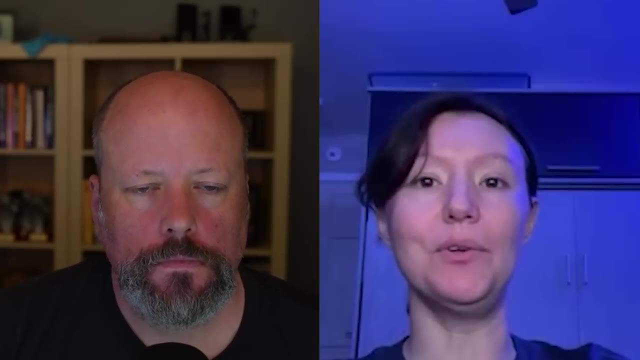 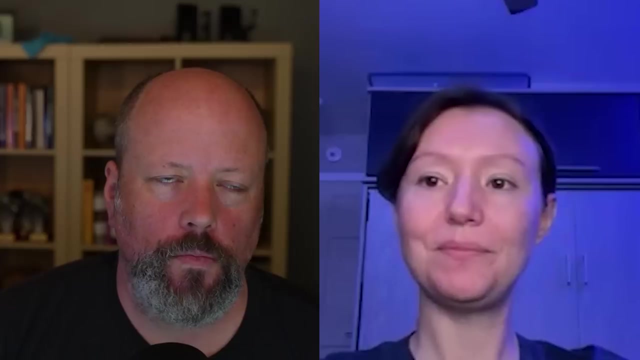 spacecraft, all of the nasa stuff, all the nasa stuff. yes, like it's like it, it's part of their contract. like they're, they're obliged to do that they have to, otherwise you know they're going to be in breach of their contract with the government. yeah, when people always say to me, like, why is nasa? 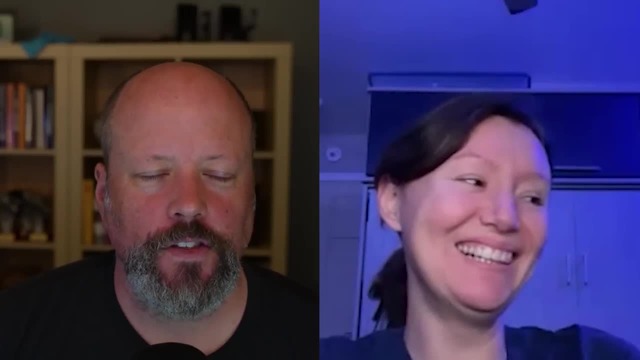 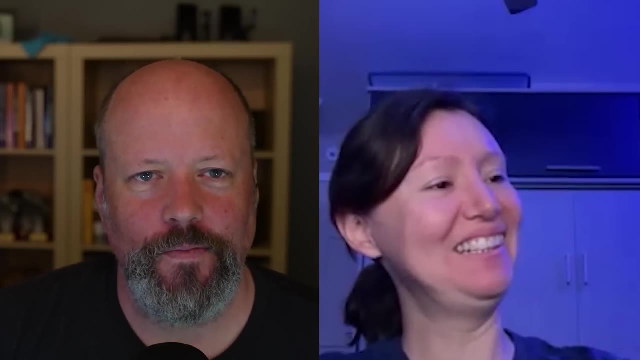 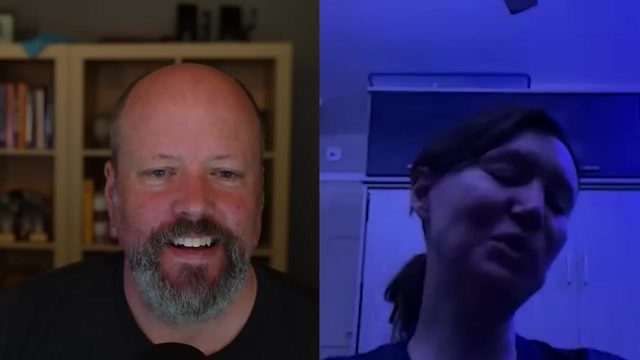 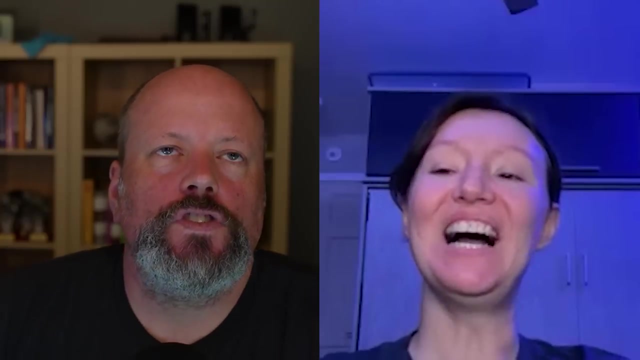 hiding images from the curiosity rover i'm like here. take a look at the raw images. the curiosity rover- 150 000 images. get to work, enjoy. uh right, they're all there, every you. I had a guy one time who was like: why are you removing the cosmic rays from? 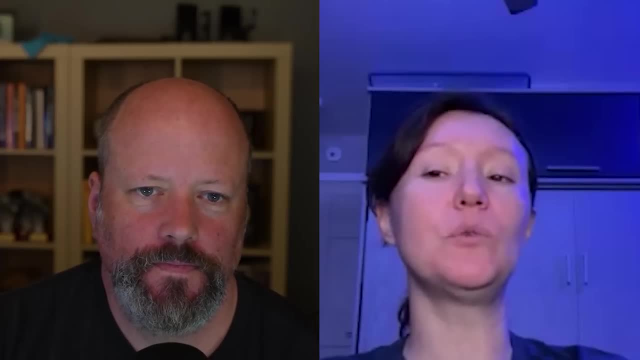 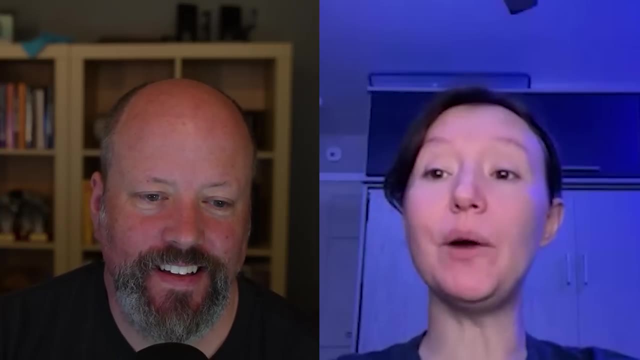 the images or i don't know. he. he was just like kind of one of those conspiracy kind of people and i was and i taught him: like you want cosmic rays, you got it, i'm gonna teach you how. and i just gave him a really quick rundown of what it was like and i was like, okay, i'm gonna teach you. 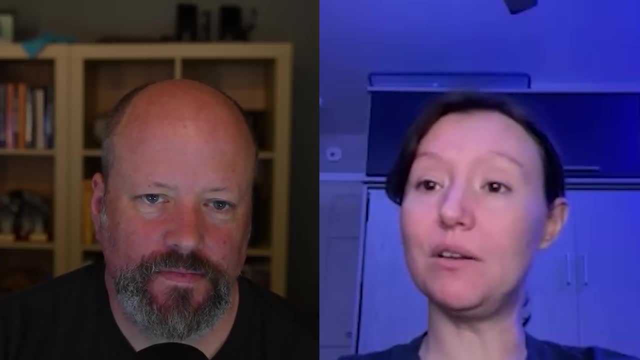 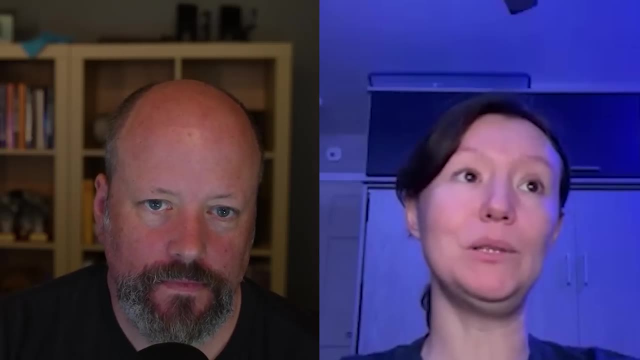 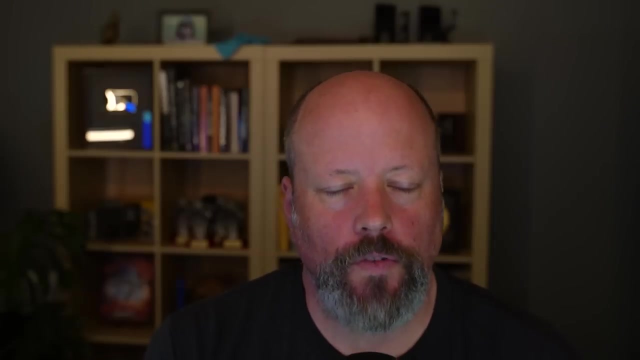 how to go through the archive and see all the cosmic rays that he could ever want. i'm like, yeah, if you can find out something about those cosmic rays, you're awesome dude. but, yeah, have fun. yeah, yeah, you dig into it. yeah, yeah, it's the same thing. like like bring. ground-based images are. 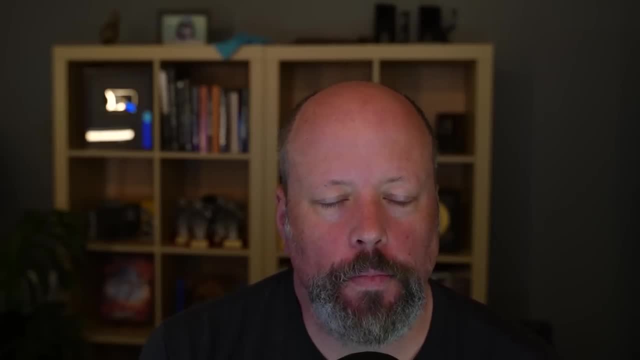 are getting a satellite trail moving through their image or getting an airplane passing through, like you, throw out those frames. they're they're not helpful, they're not giving you any value. um, so then, what do you do when you're in a situation where you're in a situation where you're in a 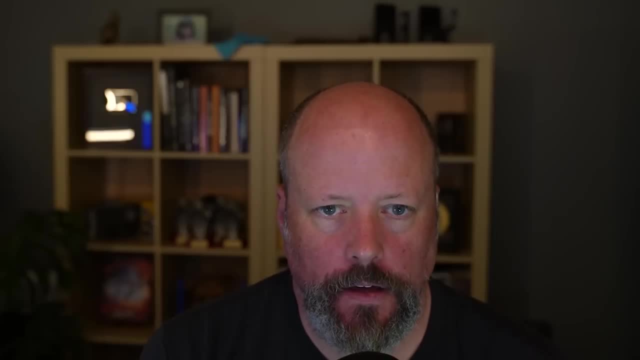 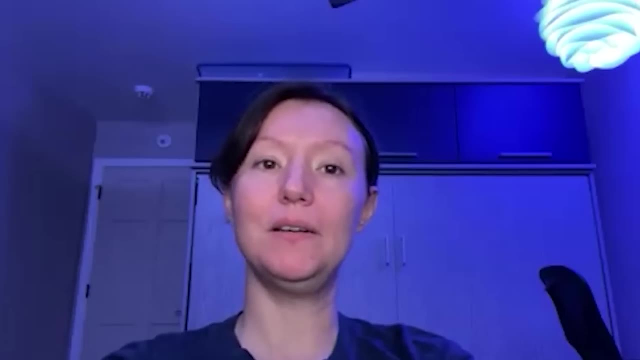 so then, how do you pull the raw data into something that you can actually work with it? well, there's, uh, another thing that isa created for people like me who want to get the data and like take. it's called a fits file, and i'm not going to try to remember what. 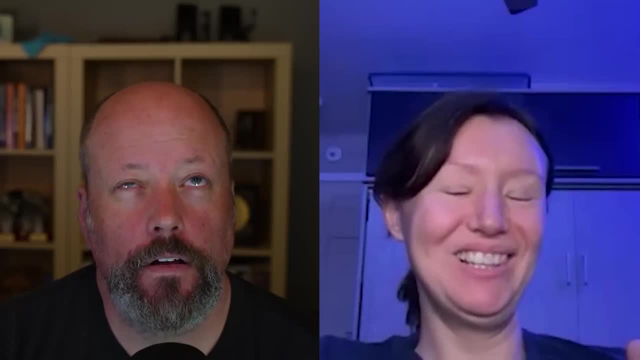 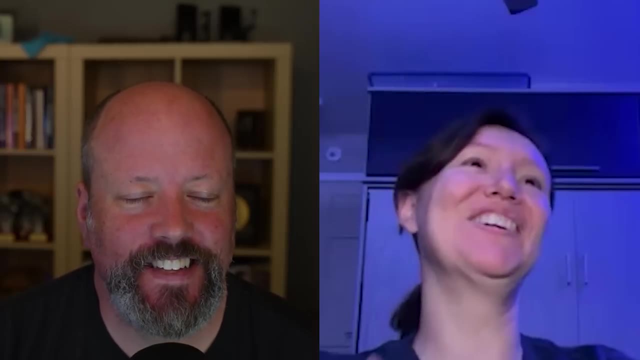 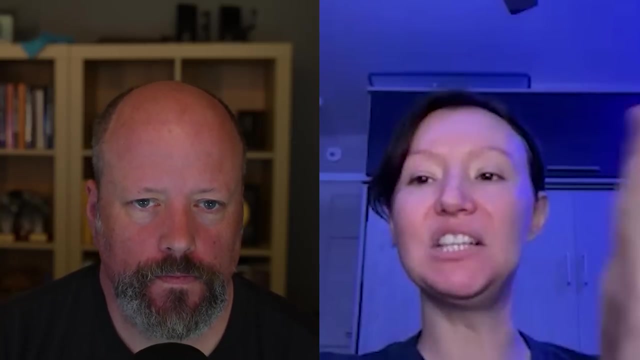 that stands for something, something: transport layer, no layer system, system fits image. yeah, you're right. anyway, fits f-i-t-s. yeah, yeah, that's all i remember, but anyway, it's, it's an image. that's the important thing. it's an image. you take this thing called fits liberator and you can. 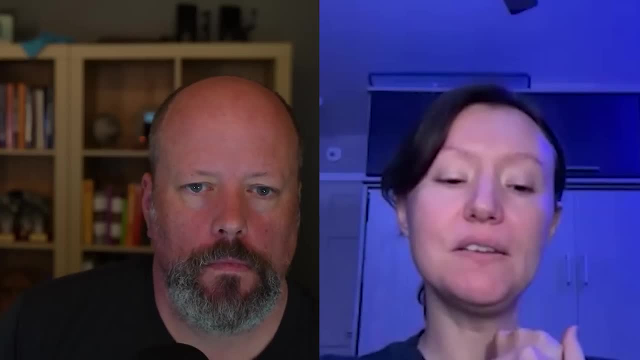 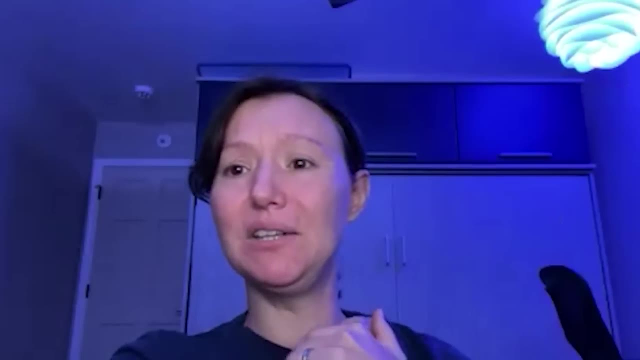 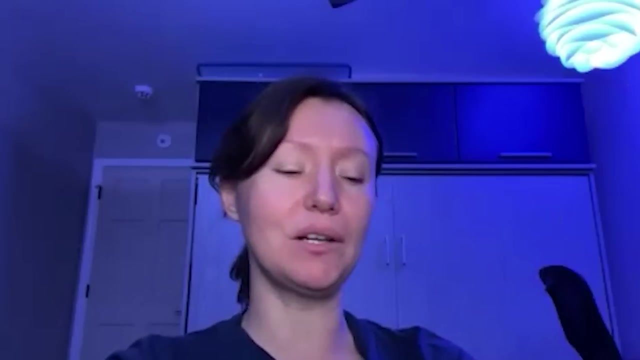 you stretch the data however you want and i i find that it's just the best. i've used, like the, the astronomical data- ds9 they call it. i've used that. i can't get a good stretch out of that. no matter what i like, how hard i tinker with it, i cannot get a good stretch out of the fits liberator. 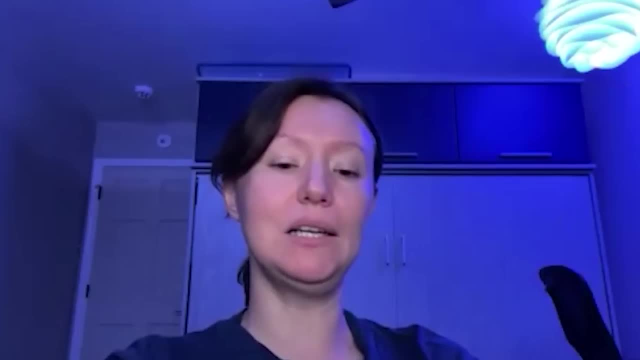 i just feel like it's the best. it i can get all of the the little faint stuff up until the very brightest and not have it like everything being at zero, everything be at 100 and i get everything between. i get the entire dynamic range with fits liberator. i save it as a tiff, you can save it as. 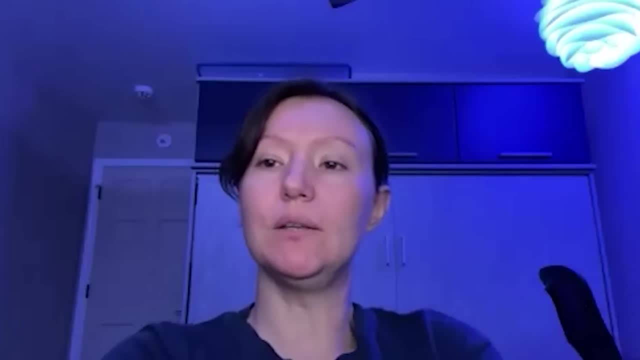 an 8-bit tiff and i can get the entire dynamic range with fits liberator. and i can get the entire dynamic range with fits liberator, which it's not very good like. it'll work if your computer is slow, but i usually just work with 16-bit. uh, you can save it as 32-bit, but your computer will. 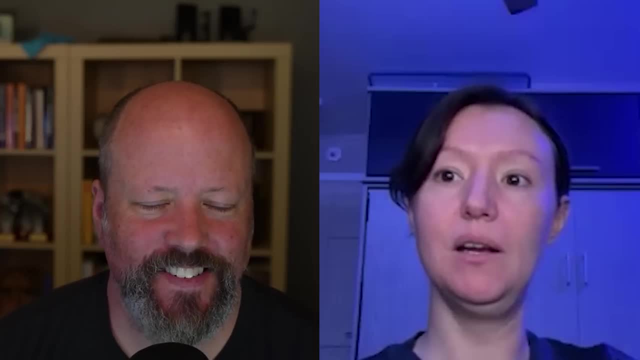 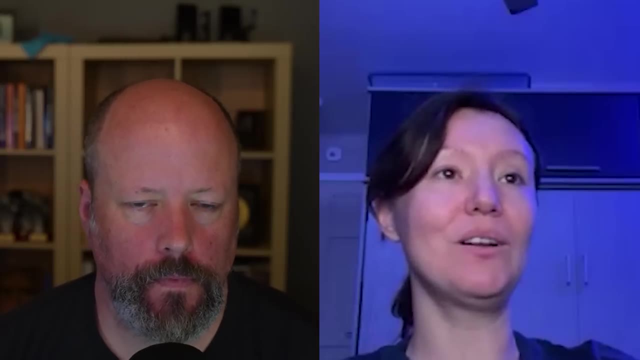 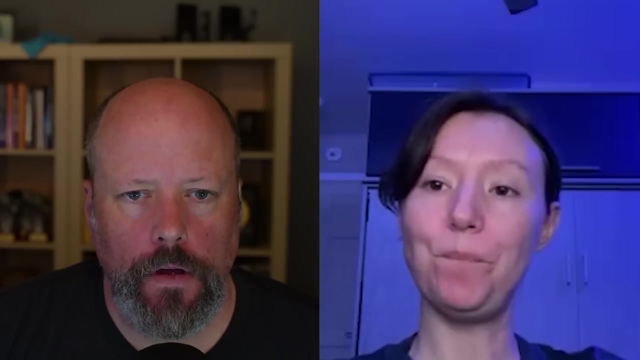 will just be like: what are you doing to me? right, right too hard, but, uh, your computer will tank. so i 16-bit is hard enough and good enough. so then you can open it with photoshop and what do? what are you opening out of that in photoshop? you're getting 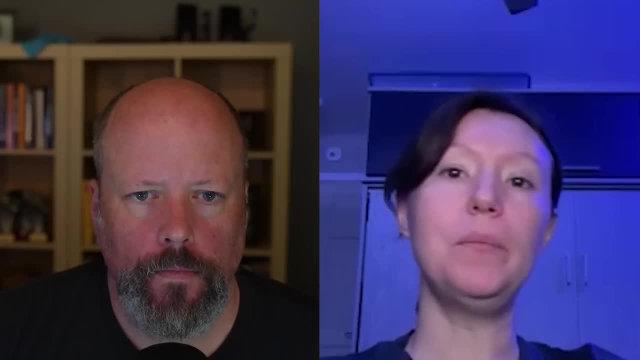 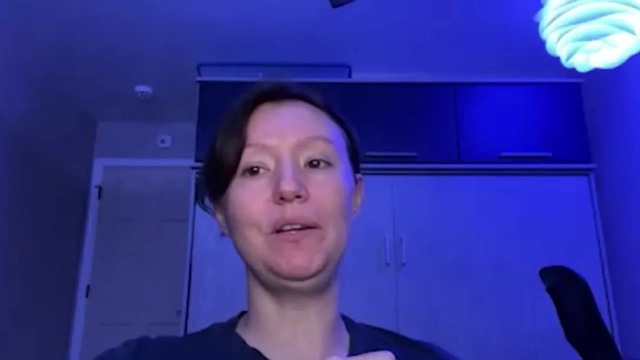 separate like layers of the different colors. no, you get a black and white image. uh, it's with jwst, it's not even aligned. you're gonna get it at different scales, like because with miri you're gonna get something that's like much lower resolution. right, because, because the wavelengths are getting longer with 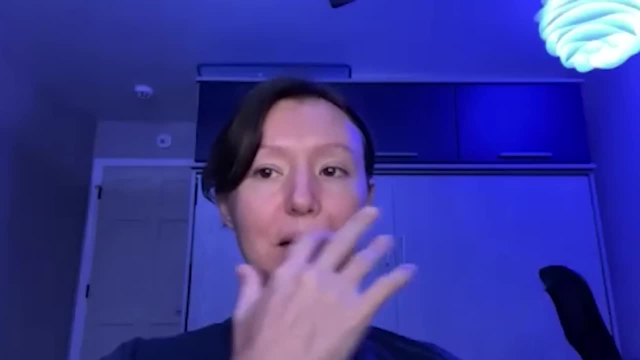 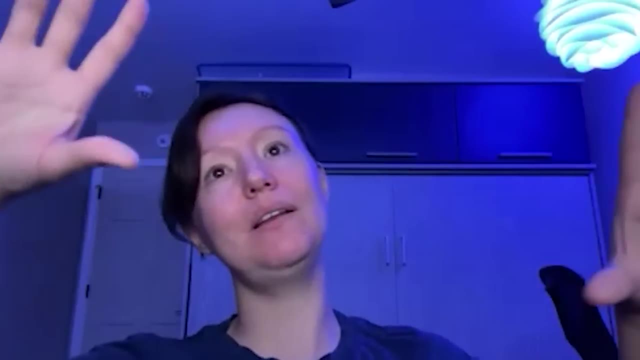 miri and then with near cam you're getting a higher resolution and then you're gonna have to like scale the miri data up to match that near cam and then you're gonna have to like scale the um, miris, smном and then i just have the jurors and jwc works and everything else. but i'm doing it. 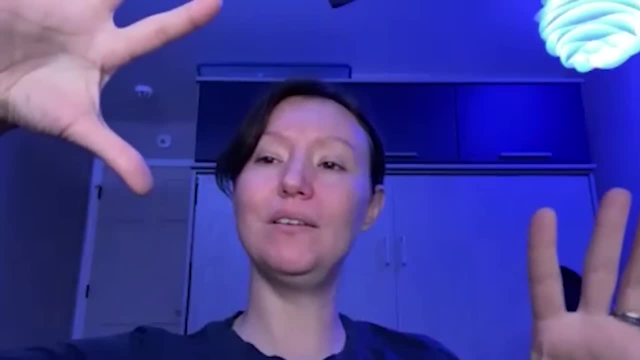 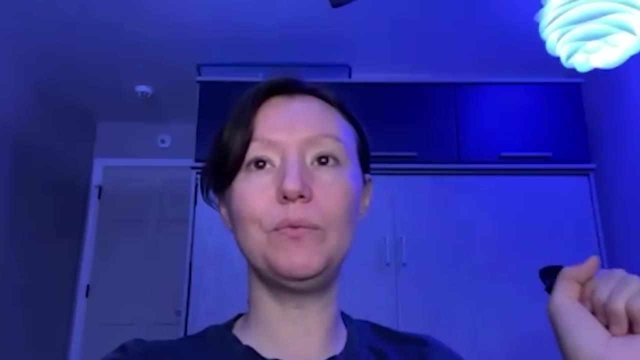 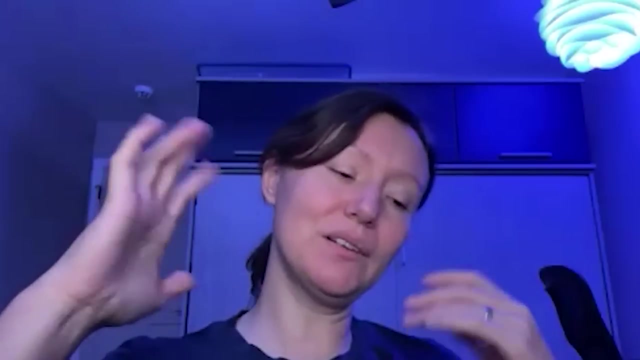 better, and then it's done in jwc, and then it's done in hacen and it's done in oh yeah, which is like the way jusj wc works, is like the cameras just kind of have like just a little, a little bit of rotation, so every single picture like it's not. maybe the pipeline will fix this later, maybe not. 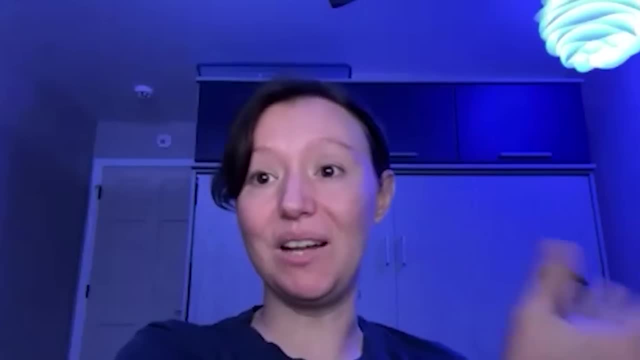 i don't know. i don't know what their plans are with that, but with it it's just the raw data, well, quasi raw, because it's already gone through the pipeline right, and so it's not technically raw at that point. but it's what it's close in color, the actual camera. 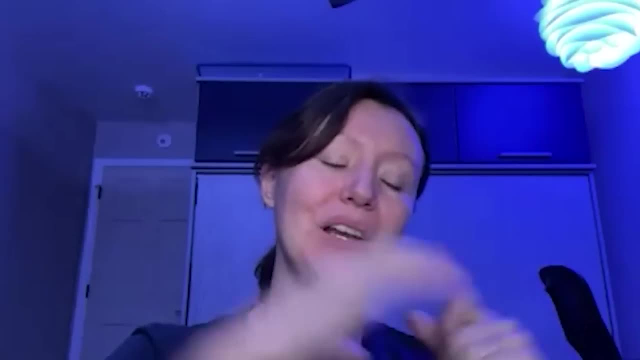 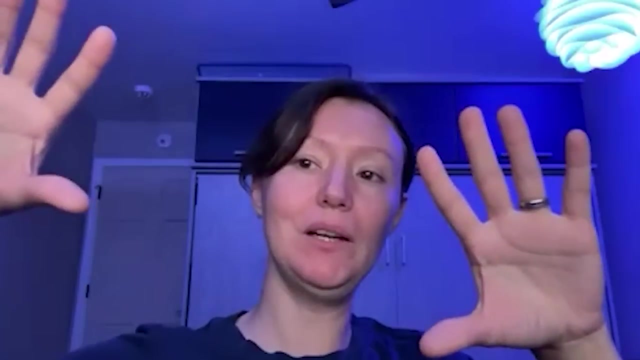 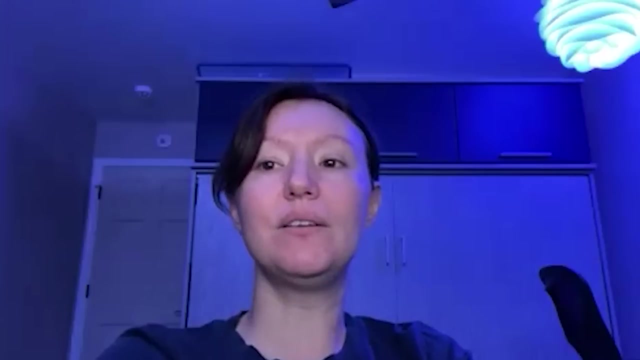 it's close enough to raw that we could call it raw. but yeah, so each little filter is going to be slightly off, another slightly off, and then maybe a little bit off that way. so then you have to align each black and white image, and once they're aligned then you can start deciding which. 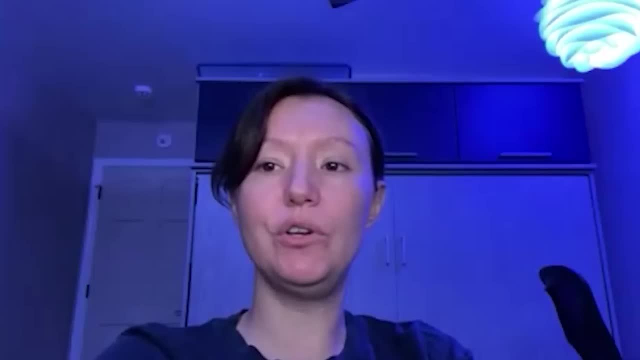 channels. you want those filters to uh to be seen through, like you want the miri data to be in the red channel and then maybe the neary, the near cam data, in the blue channel. then maybe you've got something in between that can go in the green channel. but if not, that's fine. 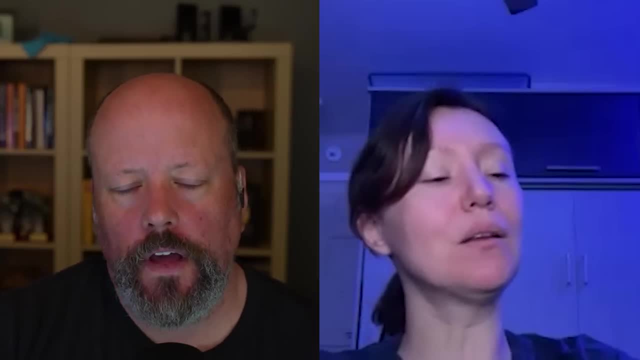 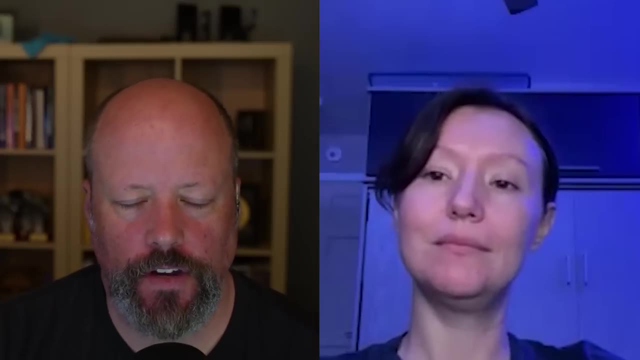 then you can just do a two color image, um, right, and so this idea of like the hubble, like when people think about classic images from the hubble space telescope, like they think about things like the pillars of creation, um, and of course, today i know, yeah, we just got the pillars of creation from 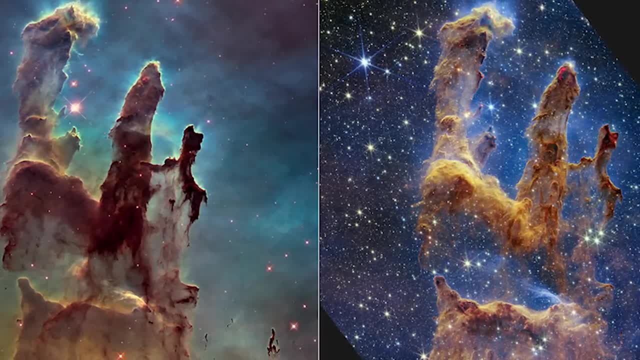 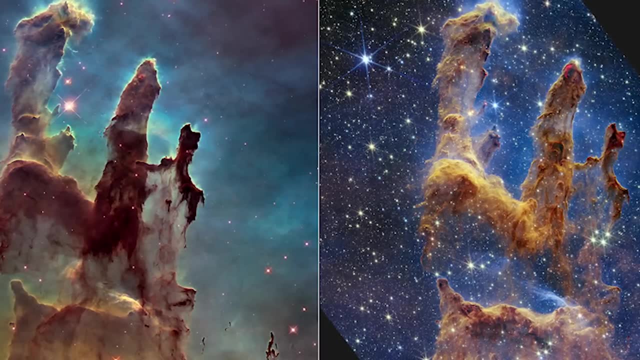 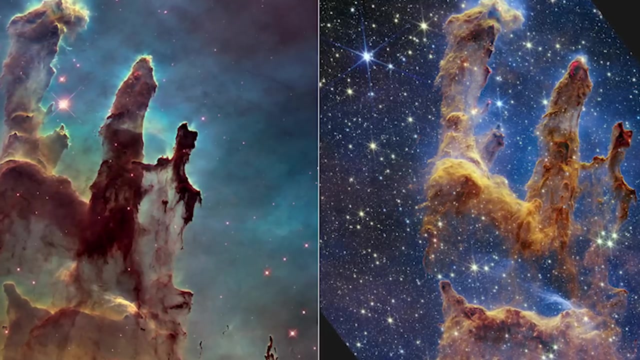 web. so did you work on that? so many stars? yeah, um, and so those are multiple images captured by hubble, recorded in black and white on different filters, that then somebody is assigning different colors to those different filters to produce an image that looks like it's full color. 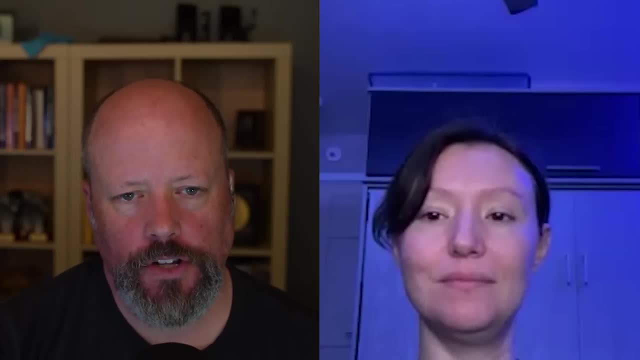 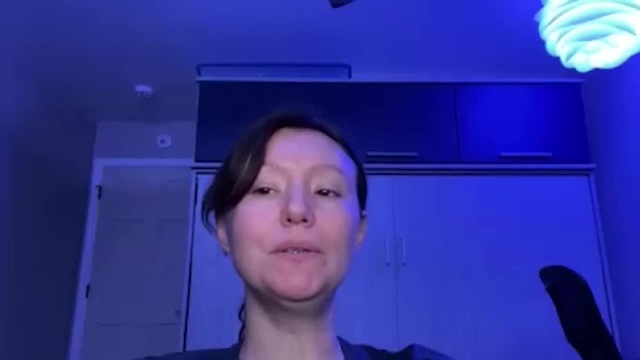 do you think people realize how much this is open to interpretation in terms of color choice is by image processors? some people do, but most people are probably. we've tried. i mean there's been a lot of outreach trying to explain it. so i mean some people more more than used to know that you know it's. 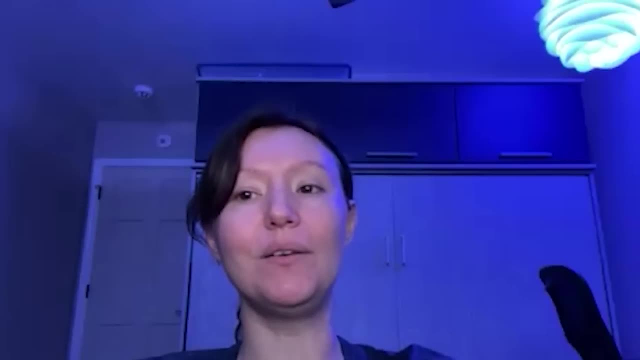 it's been processed and this is not how your eyes would see it, especially with you know, jwc and all these infrared cameras. i mean, at this time they are buying these, um, these like infrared cameras and we're just looking at things like they're using infrared light for all kinds of images. 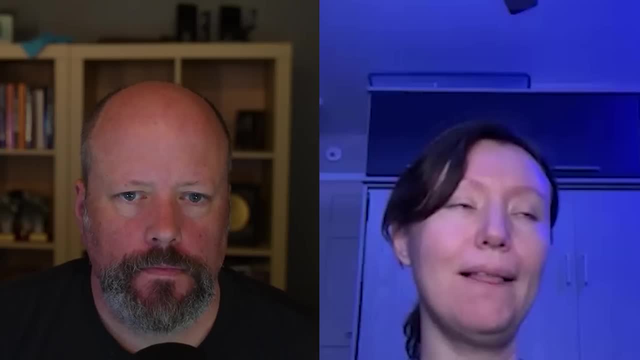 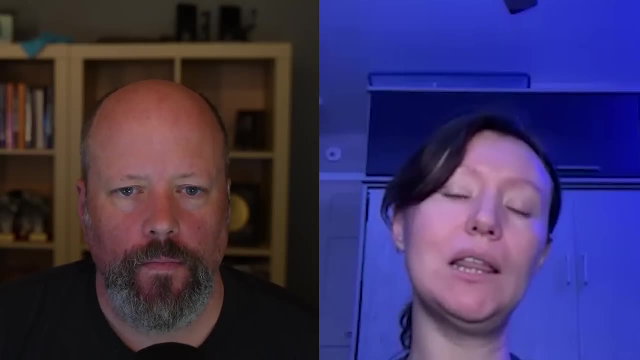 yes, my god see, if you just go to um. thank god, my god, these are, you know, infrared, low light, eles, severe infrared light they're. they know i can't see if you're at light, and the most they know about infrared is it's like, uh, night vision cameras or, you know, when you see those, uh, temperature families. andavoare lander. you know what you mean. the way you see like a heat, yeah, well, the infrared camera your ensures. yeah, yeah, yeah, I don't know it's- I know that it's ever since chandra that there have been important. Like chandra and Eve Anyausted三点, repente teams have reacted to infrared light using infrared work. I think Ts prepared this office of photography that took a. 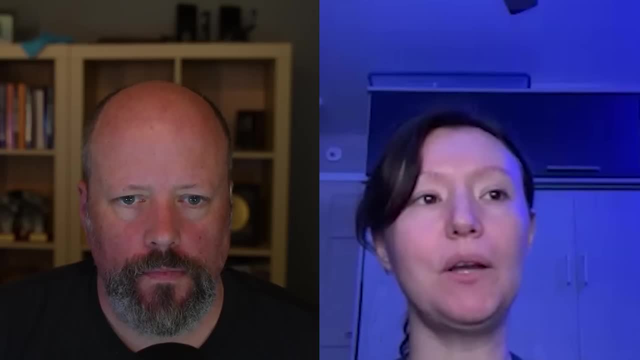 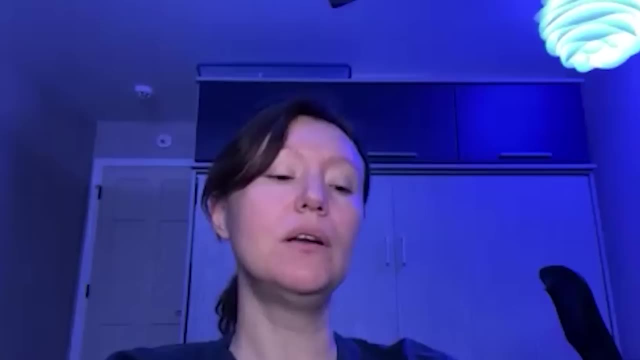 since, like chandra harvard, the harvard people have been trying to figure out how to best explain it to the lay people and they've come out actually with: uh, they have this whole aesthetics and astronomy thing where you can read their papers that they've published explaining what worked. 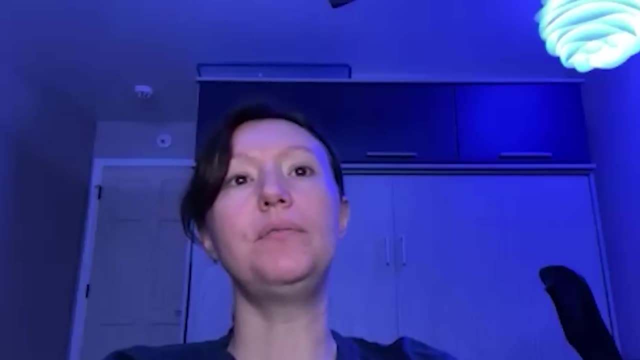 best and what didn't work. and they find that it's best to just call everything light, x-ray light and infrared light, invisible light, and try to say, like, compare it with it, like obviously with chandra, since they're x-rays, they can just say: when you go to the doctor, you get an x-ray and 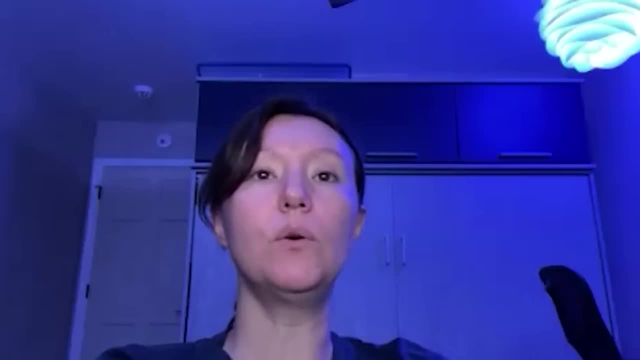 they take a picture of your bones and you know that you can't see that with your own eyes, but a special camera can and you know that's a photo just like what you could take with your phone or something. it's just a special camera that does the special wavelength that you can't see and i think that helps people a lot because 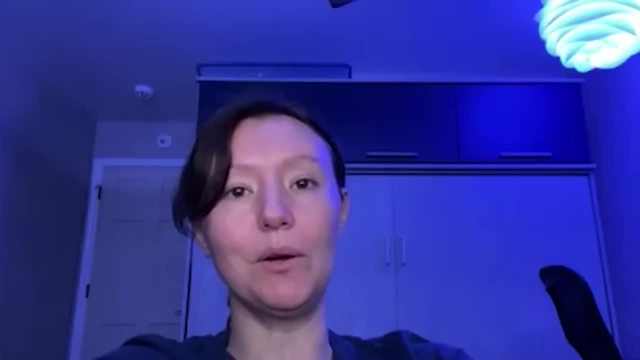 they're very familiar with x-ray photography in that regard because of medicine, and so then it's just another step up to say: and now we do this with infrared too, and that's just. you know the other direction on the you can't even say really electromagnetic spectrum, because everybody learned 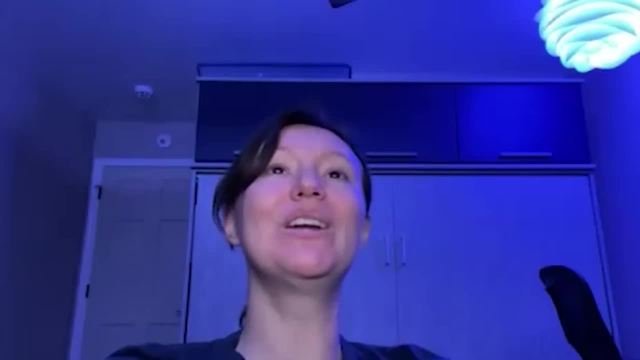 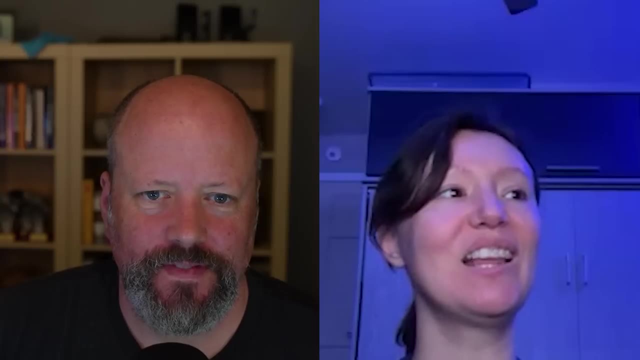 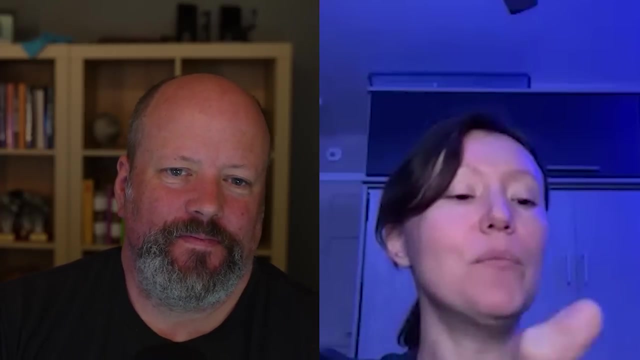 about it in high school, but not necessarily everybody figured. i mean electromagnetic spectrum that just does not sound like light electromagnetic, that's like a zappy, a zappy magnet. that's, that's right. that's almost like a solid, like i have a magnet in my hand and it will electrocute me. 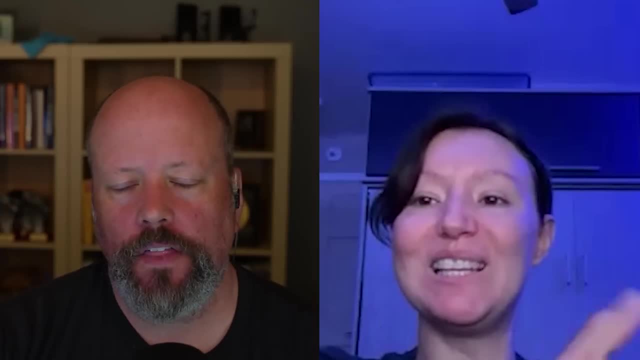 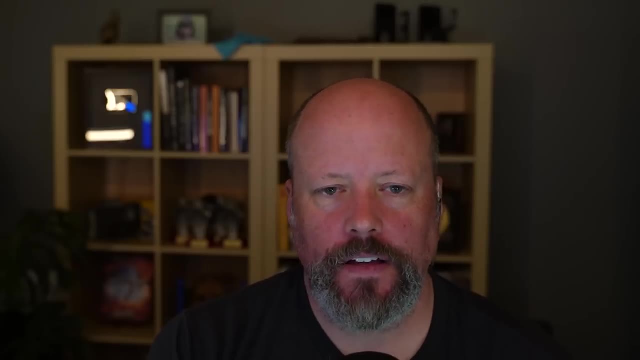 that's what it's. yeah, but like this idea that radio waves and microwaves and infrared and visible light and ultraviolet and x-rays and gamma rays they're all the same thing. they're just different wavelengths of the same thing. they're all the same thing, they're all the same. 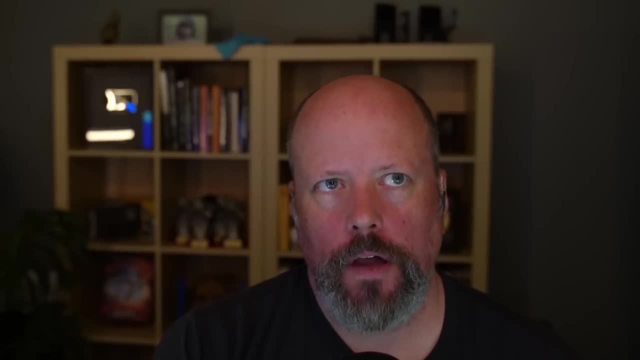 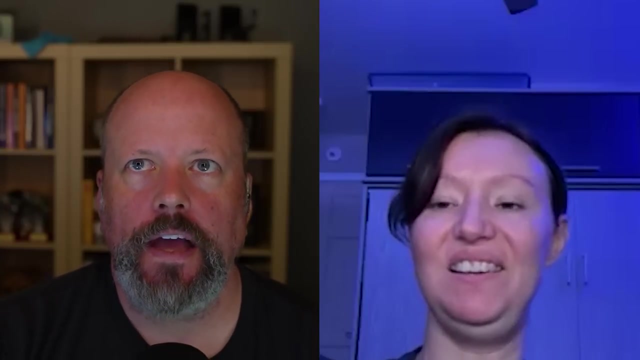 radiation, and i think it's become a lot more useful for people to understand this, because what web is doing is it's observing galaxies that were visible but now have been pushed into the infrared because of the expansion of the universe. yeah, that's cool. about the deep ones, yeah, and so. 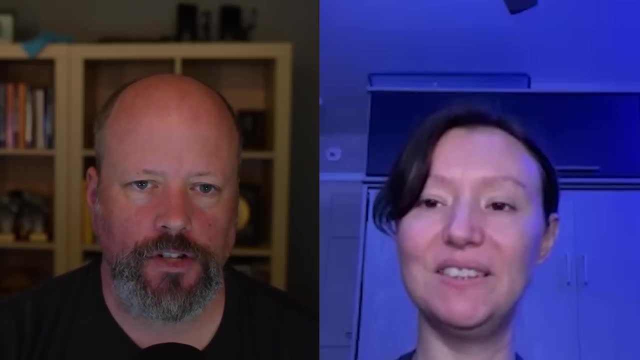 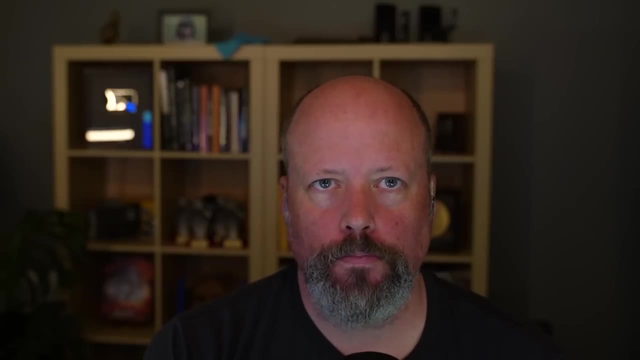 when you're taking an image, when you're when you're showing off an image of a galaxy- it was taken by web- you're- you're kind of trying to reverse time. and you're trying to reverse time, you're you're pulling in these images at infrared wavelengths and then you're kind of going. but if 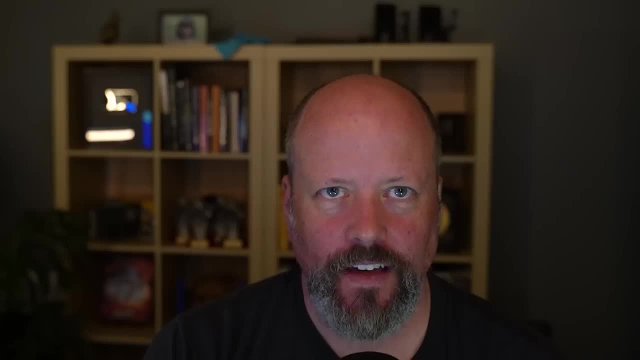 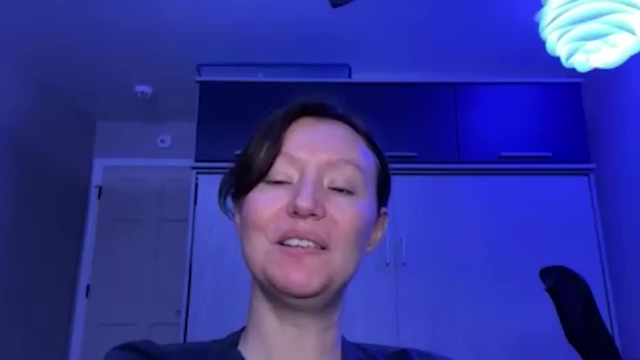 you could see this galaxy with your own eyes today. this, these are the colors that you would see. how, how do you sort of approach that right, like if you can go far enough back? i i don't even think like jwc hasn't even really done a true deep field yet. not yet unless it's yeah, unless it's a you. 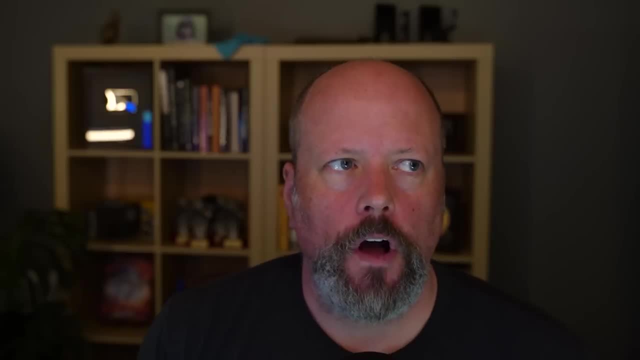 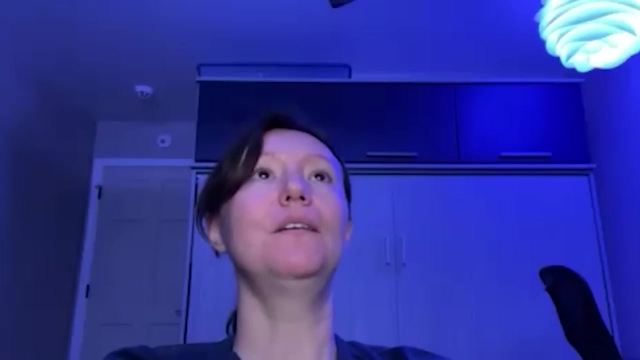 know proprietary, but i don't. yeah, they're working on. the cosmos web is one of the main surveys that they're doing and they've been releasing that in in bits and pieces, but they're. but there are plans to do a, a gwst version of the deep field. yeah, yeah, so. 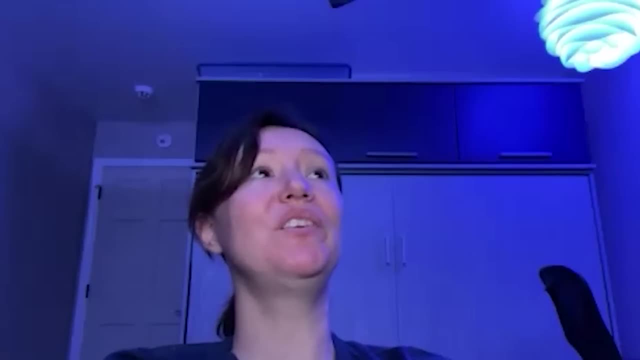 yeah, that's really cool because by the time that light gets here, it's basically a visible wavelength in it. you can tell, because when you process it, the the filters actually start acting like rgb filters. it's like, oh, this one, actually it comes out in it. it's like i don't have to do. 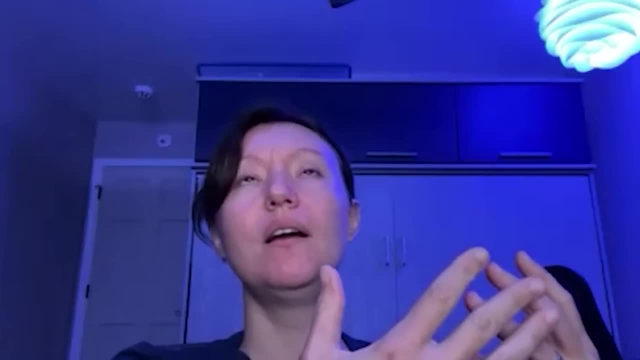 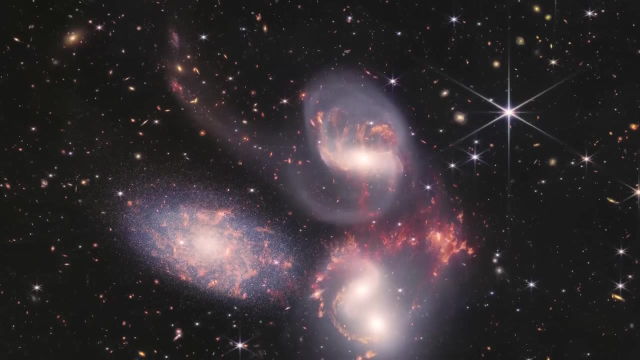 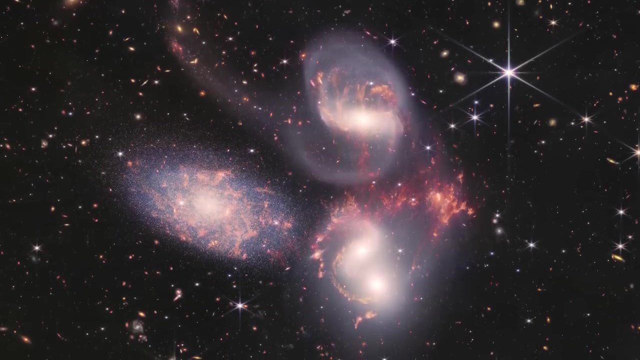 anything with the, with the nearby galaxies. it's like you saw the. uh, was it safer to text that or was no wait, it was the other quintet, steven's quintet. right right, steven's quintet. yeah, they had to work really hard to get those to not look like all green and uh, yeah, the green is the big. 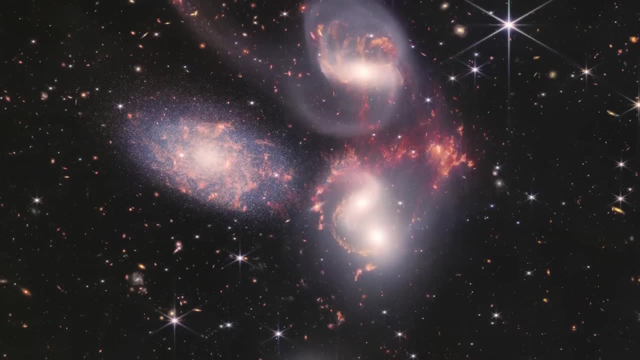 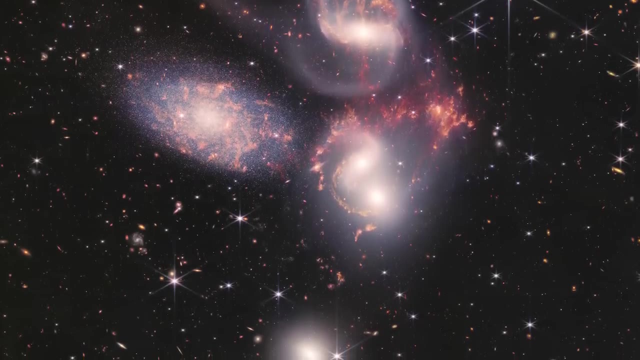 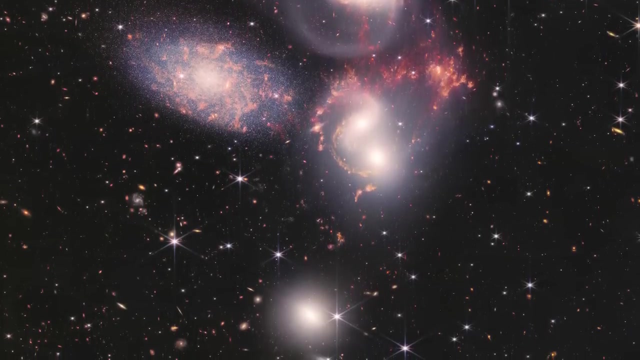 problem like things. things look really green a lot of the times, like when you just go, okay, longest red, medium green, short blue, it's for whatever reason- everything just ends up looking green, like we get these weird green galaxies. so you have to work really hard to make it look aesthetically pleasing. 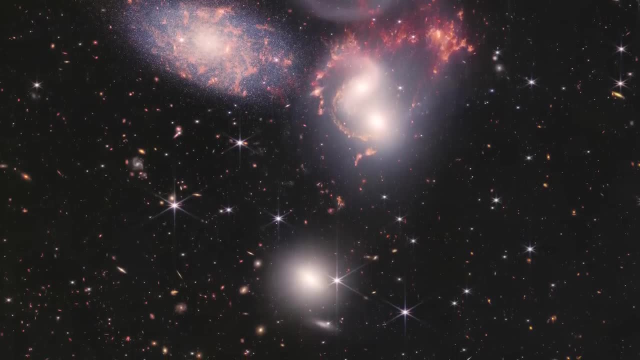 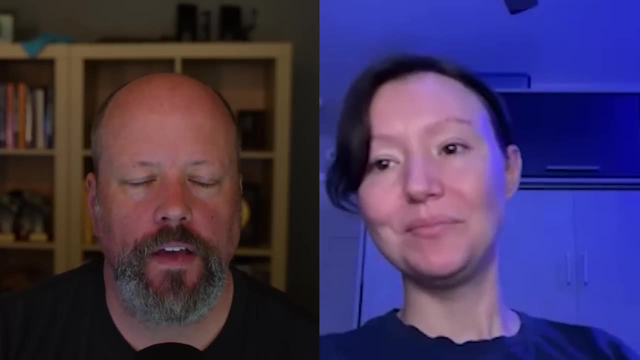 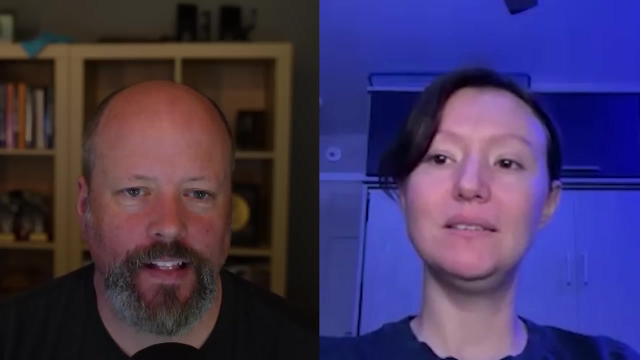 because everybody, like when they see the green, they're just like this galaxy is sick. well, i, i think it's really cool- i've been- i've been mentioning this a couple of times in some of the that i do- that i think you have figured out the web palette which is these eldritch horror, sick. 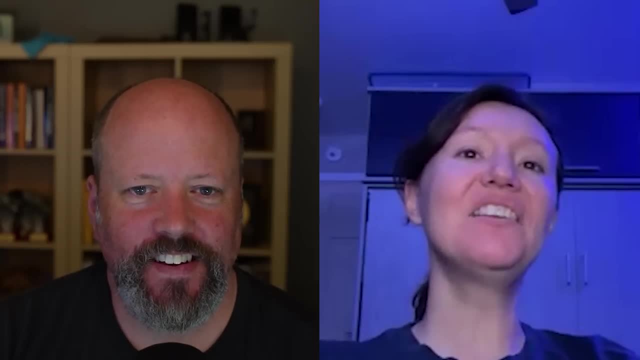 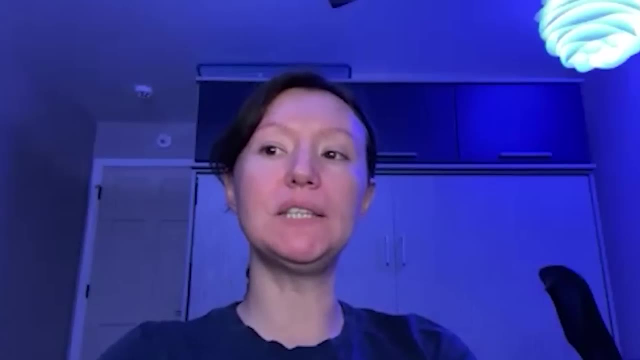 galaxies. yeah, that one. uh, right, that's something that i i when i have a difficult set of filters. i started doing that with the hubble data. if you get that weird green cue, you can, instead of doing an orange and cyan, which is a two color image, and then start highlighting things and pushing it into. 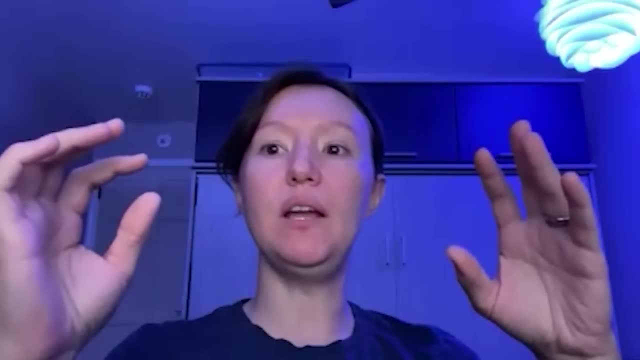 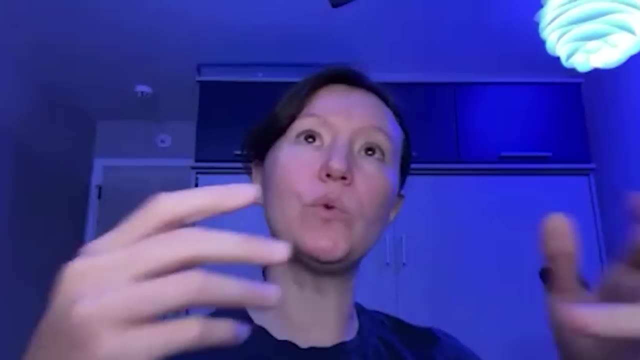 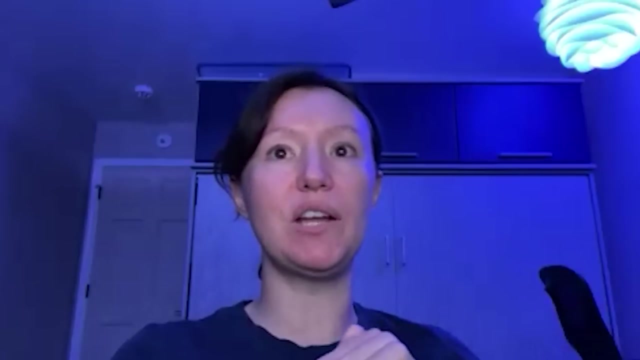 that third color by adding, say, red, for, uh, you know the the longest wavelength like, overlay that red on top and then, if you have like a shorter wavelength and overlay that blue on top, and then you start gaining a lot more depth of color instead of just that that you know orange and 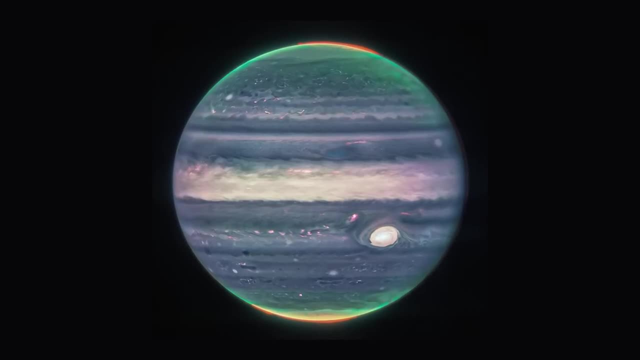 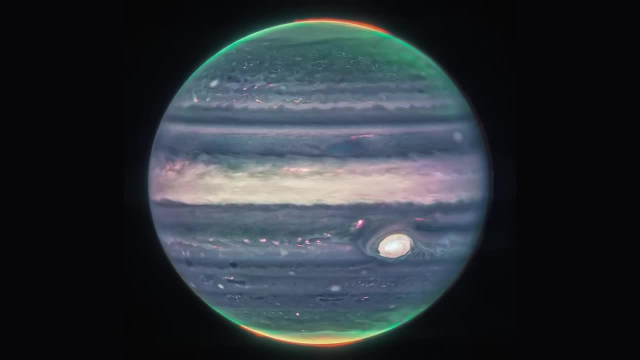 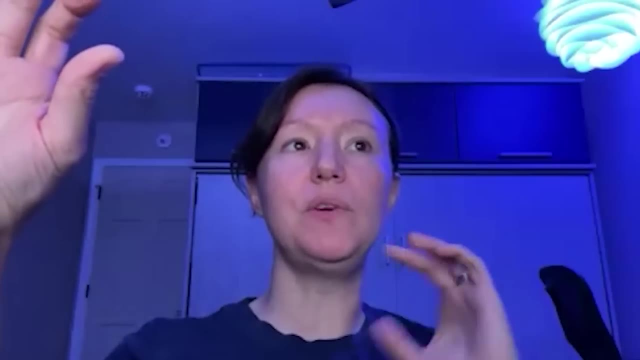 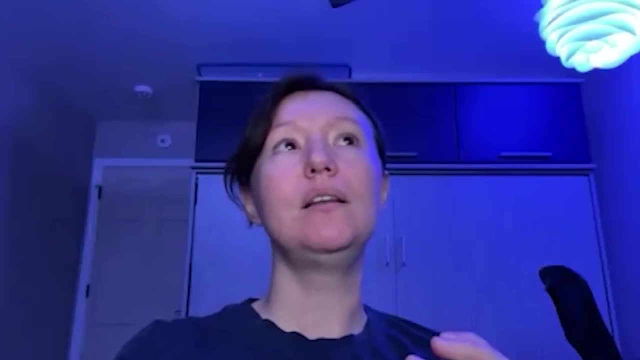 feel like they're missing that dimension of color, that third dimension of color, because the green was just, seriously, it was just 50 of the red, 50 of the blue combined together, and now we, we just made up green if and uh. so yeah, to push that dimensionality of color and 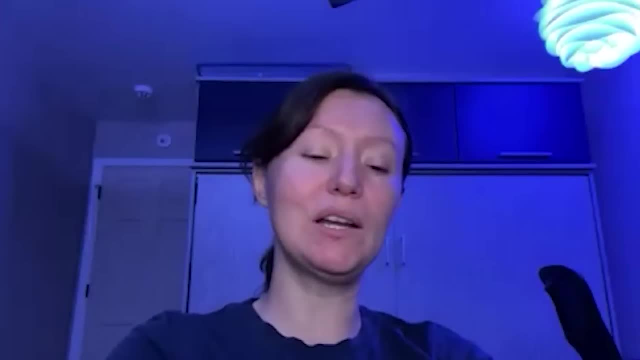 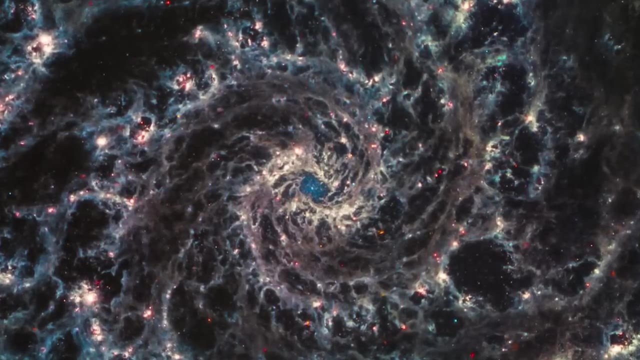 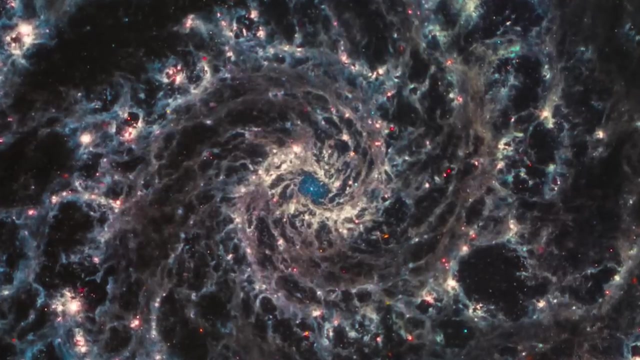 give it that extra like- oh that's, that's more like like i with the, the eldritch horror, as you call it. like you can see these little dots of red. they look like my little berries, or i guess you could say creepy eyes or something, but they give your eyes something to sort of like dart around and 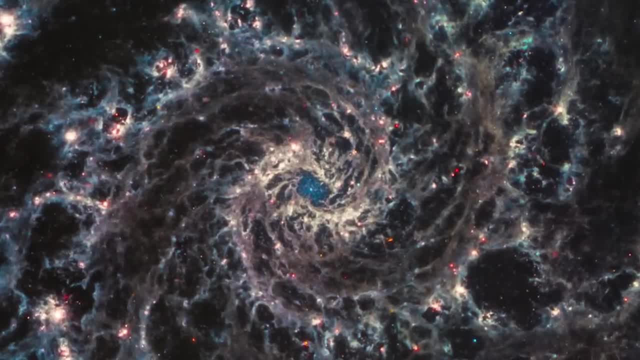 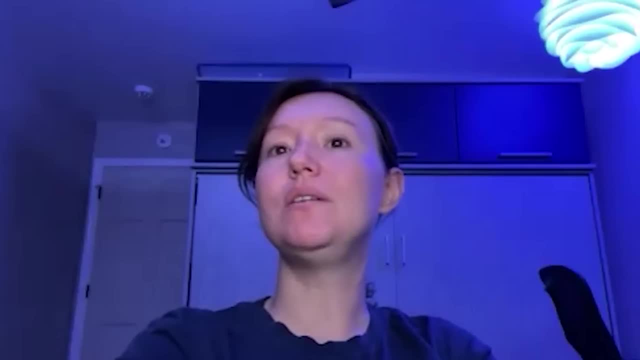 look at and focus on: like what are these things? whereas if it was just orange and cyan, you would not have those little highlights of color and they're not even like. you don't change the image a whole lot, and yet that tiny change makes a big difference aesthetically. 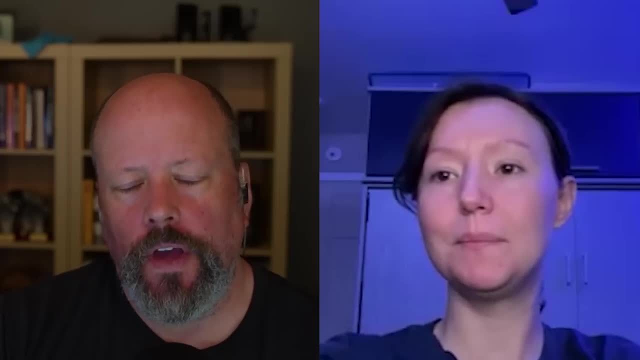 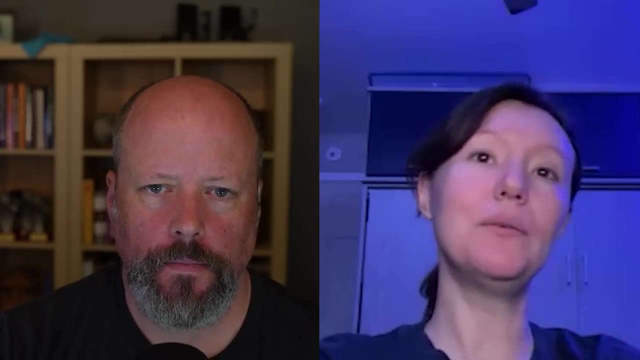 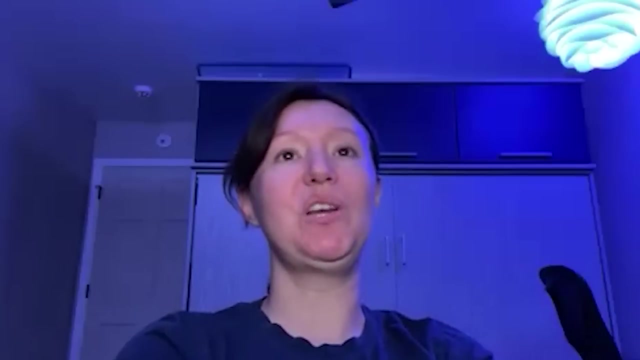 so i mean, fundamentally, is that what you're doing every time? is you're kind of going what's my red, what's my blue, what's my green? a lot of times, yeah, like if i'll just stir it together really quick, at first i'm like this isn't working. most of the time with jwc i'm like, yeah, this is okay. 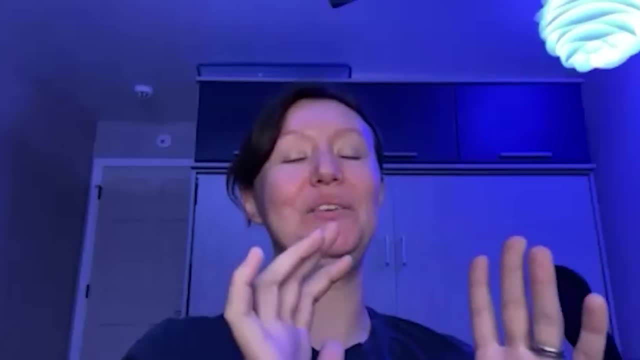 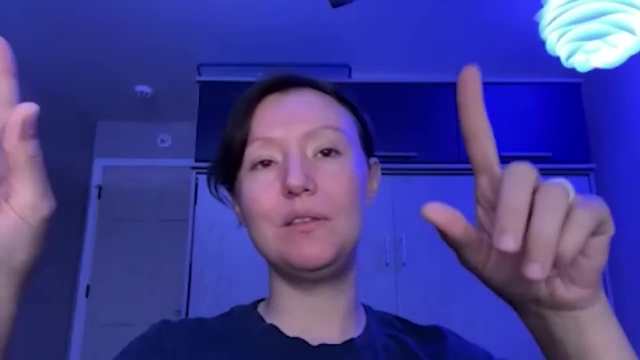 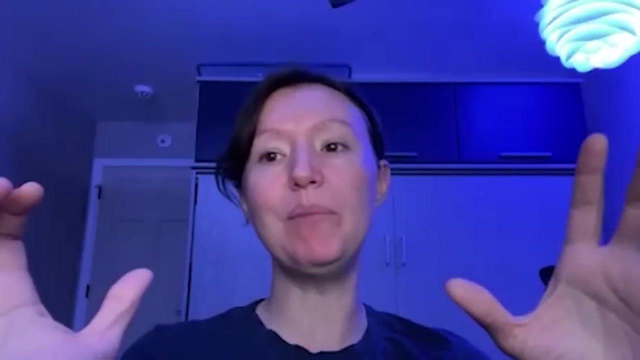 so then i will put it back to the black and white and i'll look, study the each black and white thing and say, okay. well, this one seems to be very detailed and i want to really like get this one to have the most impact on the image and 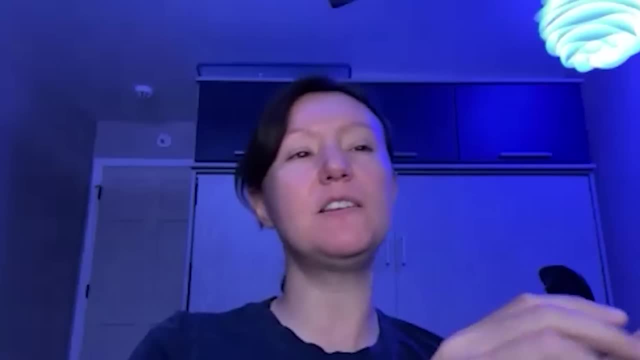 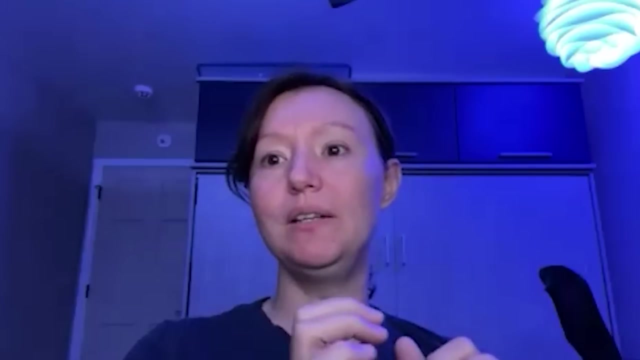 then i look at others, like, but this really highlights something different, like what's going on over here, like, so this does need to be in. it's just not like the main basis of like, say, the, the tone of the image, like there's like the, there's color and then there's value, right? so 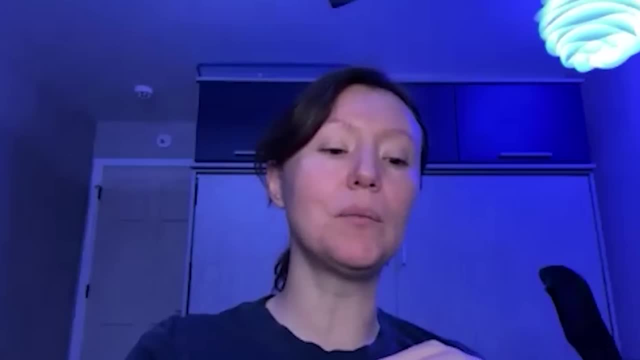 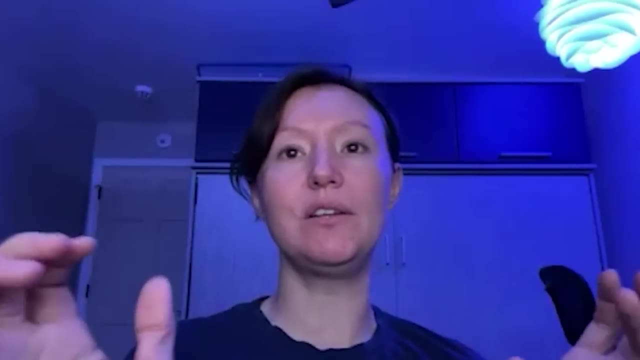 for the values you're. you can really just look at like the black and white part and like you see the entire, like the strongest structure in the galaxy. that's where i want my bases of the image. and then you start putting color and then like that's where all the the more there is like i won'tero if there wasn't a good image. so, yeah, i love it. i love, um, just how the viewpoint or the lessons and the layers are in this. yeah, i just love what took place and just really want some 痛 will do well, so, and so that was mine, but i want no comments. thanks for coming down that way, don't. 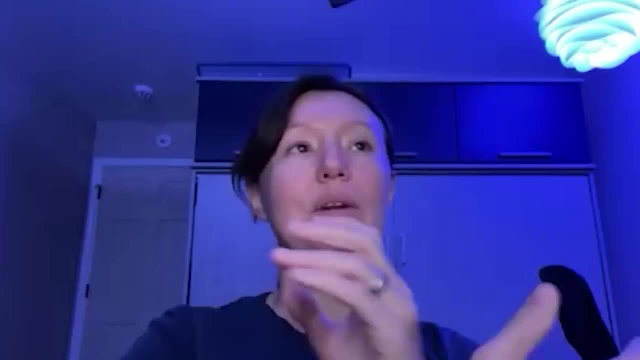 you start focusing on the color. well, well, that's what i do anyway. i don't know if other people yeah. so it's a lot of going back and forth between the black and the white and then trying to get the color to not only make sense in a scientific way, like if i just start throwing the colors randomly. 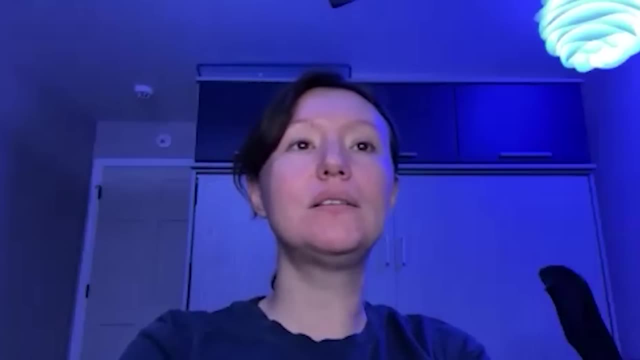 uh, like scientists, the astronomers themselves are going to look at it and be like: why is it reversed? because they know they've looked at enough pictures. they're going to be like: that's a background galaxy, it should not be blue and this is, and uh, so, unless you put a big like, 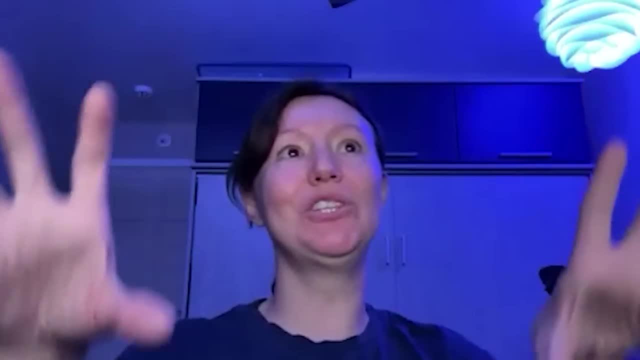 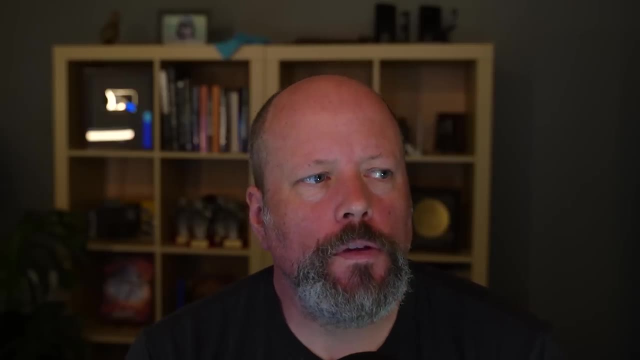 thing in the, in the description, be like the colors are reversed here, which i really try to avoid that, because then you have to explain it. but but i think about like, when you think about some of these, these objects, knowing the, the, the science of the, of the object is, is important, like um, you've got the like some of the galaxies- again we talked. 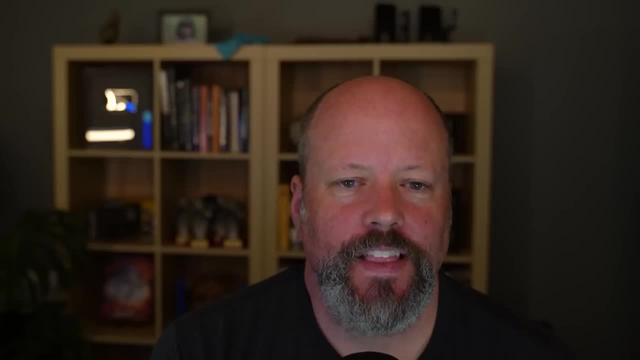 about the elder tor galaxy. in this case, web is showing you the. uh, the sun has shown up. web is showing you the, the regions of star formation and in the other kinds of images where the and in the other kinds of images where the other kinds of images where the. 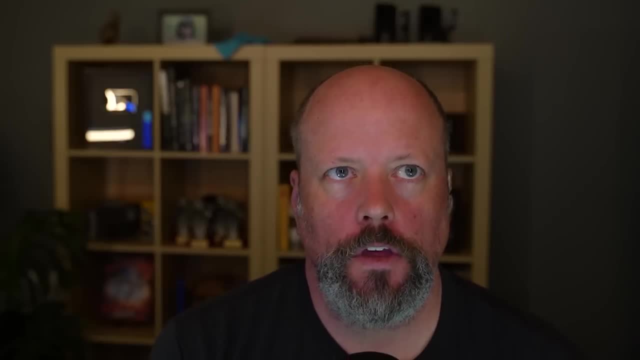 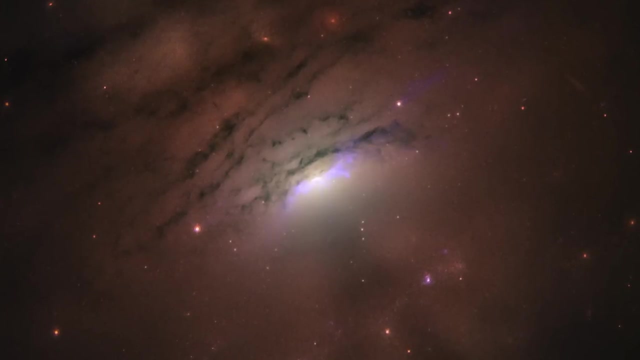 galaxy is a lot farther away. web is showing you regions that have been redshifted dramatically from what they were before, and so they're they have different meaning. like you have discovered things in your image processing that have led to scientific discoveries. what happened? i think you're talking about the, the crepuscular rays galaxy, right? i see 5063, right? i guess yeah, but 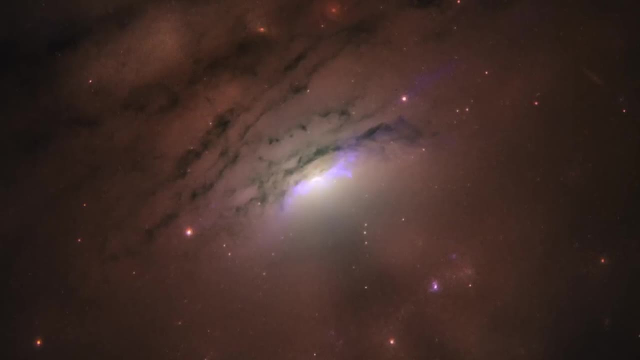 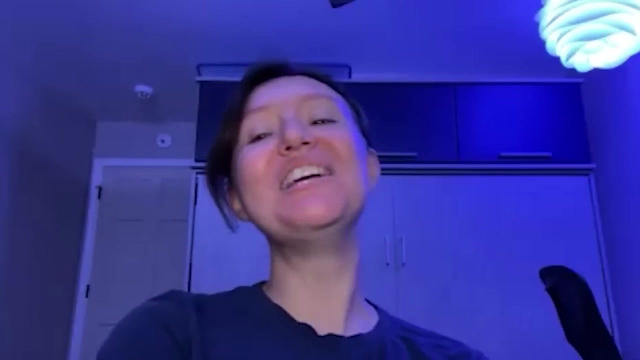 it was the crepuscular rays, that was the. that was the story that i remember, right you right that you saw something and said: is this a lens flare? and then reach out to some astronomers. i never thought it was a lens flare. i was just like, like, blinking my eyes, like, am i, is it an? 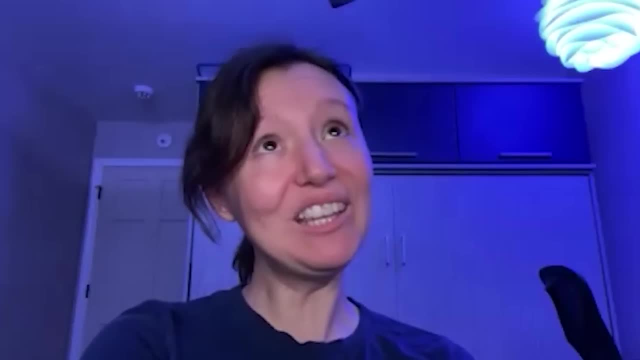 optical illusion like: are my eyes actually seeing what they, what i think they're seeing? so yeah, i was just sort of like. it's sort of like if you sit here with your morning coffee and you check on the what you check on the news, right, i was just looking at the archive. 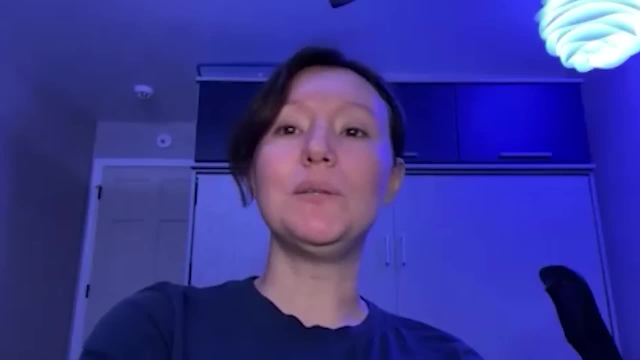 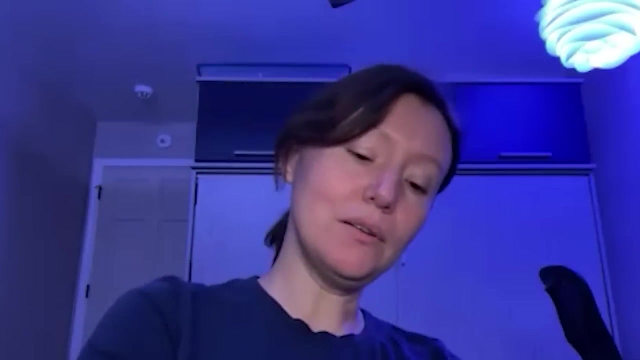 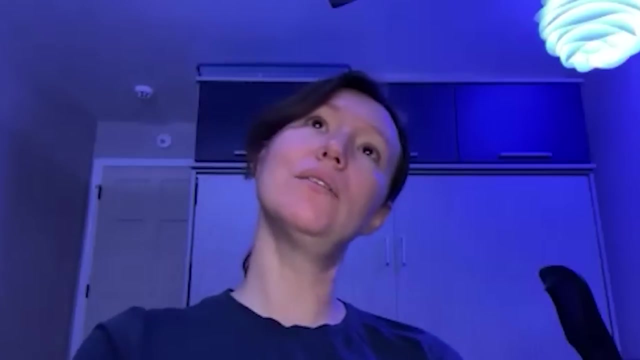 and i was like, okay, i'm gonna basically just look at whatever happened in the past week and i think it was aaron barth's, his, his survey of agn- and i was just like, oh, those can be kind of neat. so i and i was like this looks promising, this thumbnail. so i just took it. 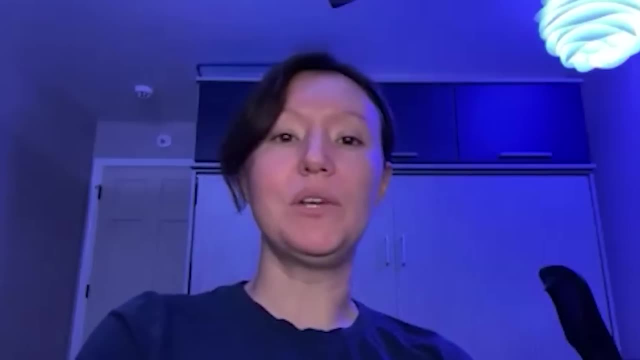 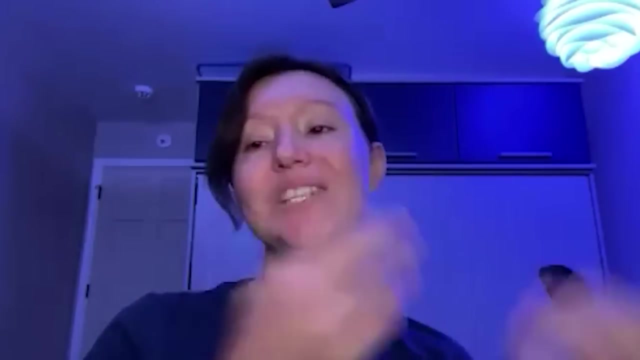 into photoshop, not knowing whether i'd get anything out of it or not. i i already knew it's only one filter too. it's like a snapshot survey, I think, and they don't even really get usually get with snapshots a lot of times. it's just that's it. you get black and white, but 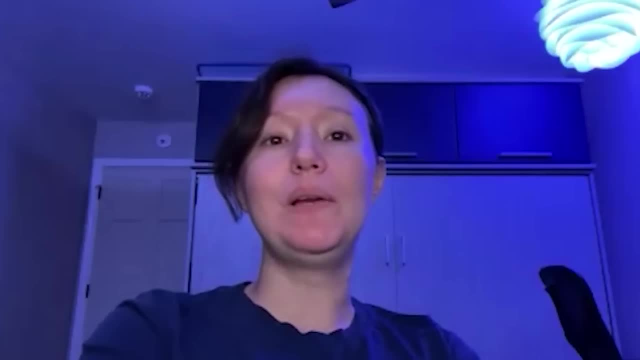 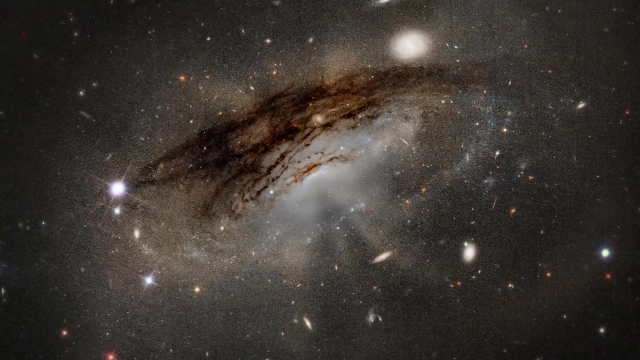 sometimes I just post those black and white images because they're still beautiful. but anyway, as soon as I opened it in Photoshop in Fitz liberator, I still couldn't see it. when I open it in Photoshop, I was like there's like this faint, like cone-shaped line. I'm like that's weird, because it doesn't look. 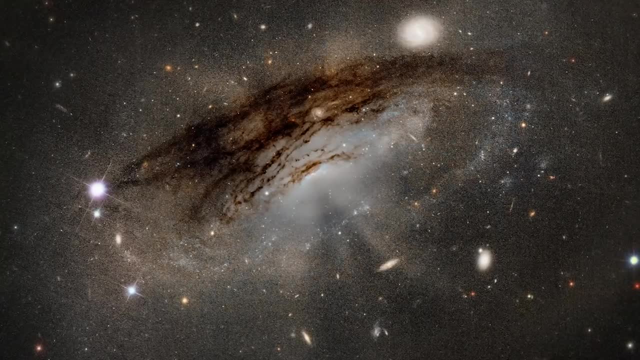 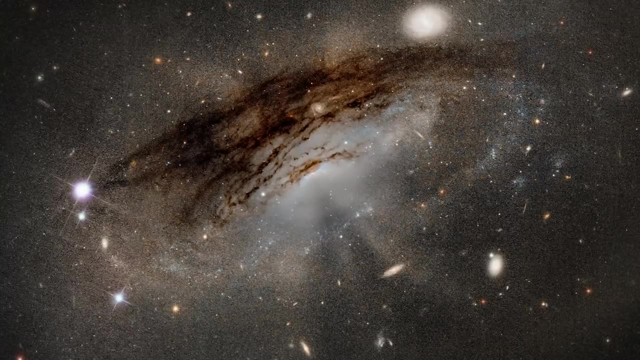 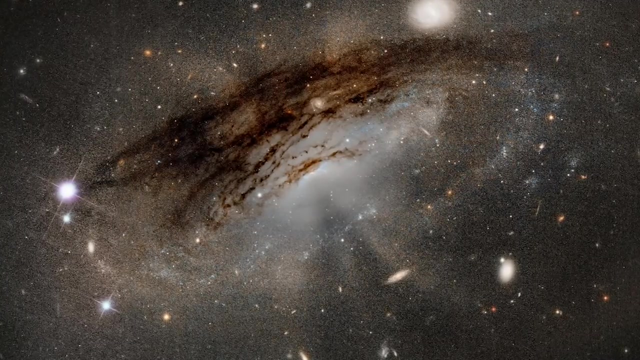 like it doesn't look like you know those like some galaxies can have the peanut bolts right, mm-hmm, like it doesn't look like that. it doesn't look like the X plus. I'm not viewing it edge-on, quite so, I'm just like: what could this be? I know it's an AGN, because I knew that. 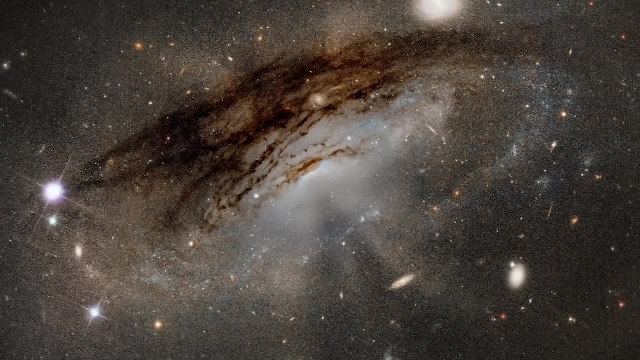 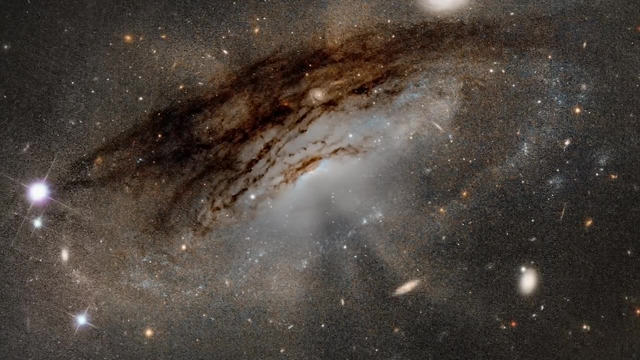 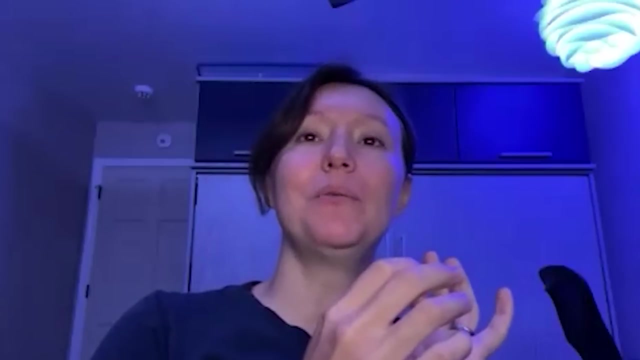 for, even downloaded it so immediately I thought: could this be shadows? could these be rays of shadows that are be cast by this bright nucleus? I don't know. so I'm like trying to temper my excitement of finding something I've never seen before with realistically, because I've done this before. I'm like 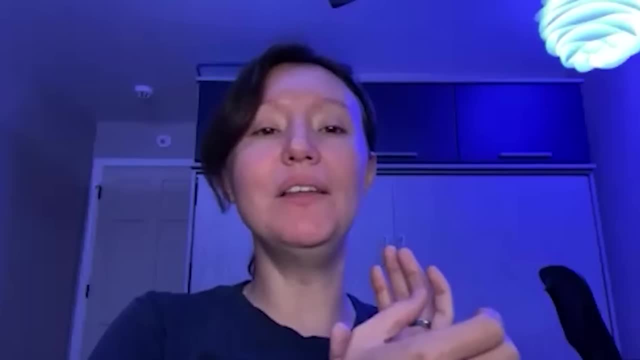 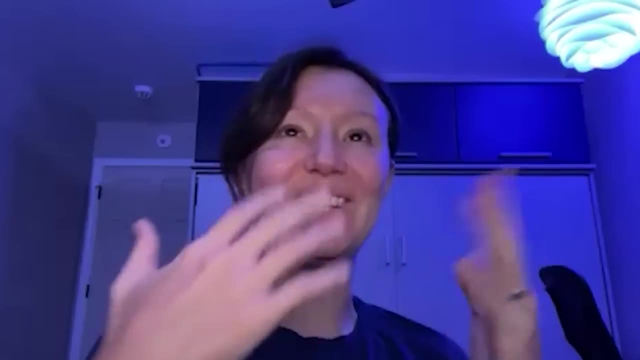 oh, I found something neat, and then later on it turns out it was wrong. so I'm trying to figure out what's going on and then I'm like, oh, I found something neat, and then later on it turns out it was wrong. so I'm trying desperately to keep telling myself like you're probably wrong, Judy, this is. 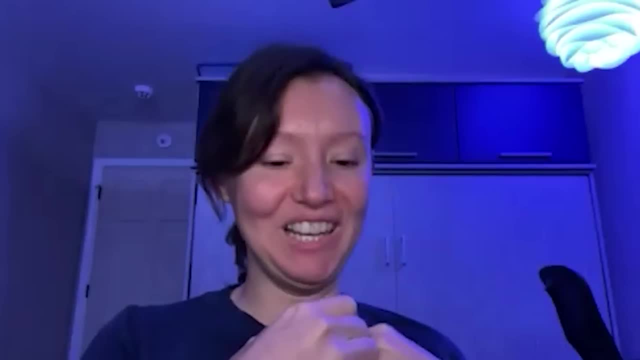 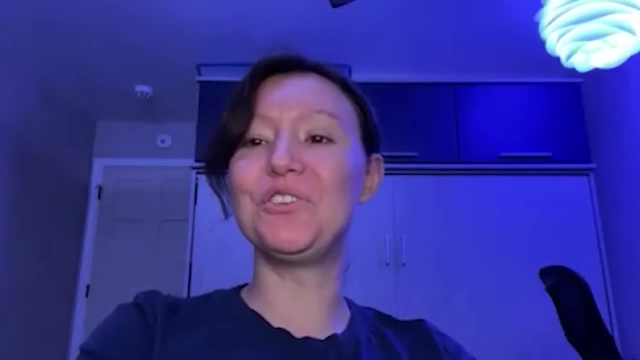 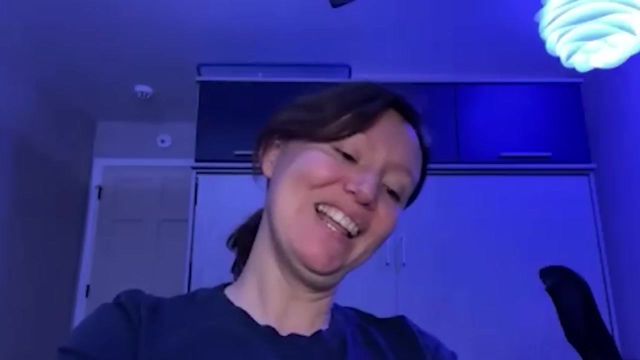 nothing. you know you've done this before and so I just like go post it to Twitter and then, you know, let's see see what the astronomers who follow me like, who just happen to see it, see what they think, and it gave them pause too. they're like: hmm. 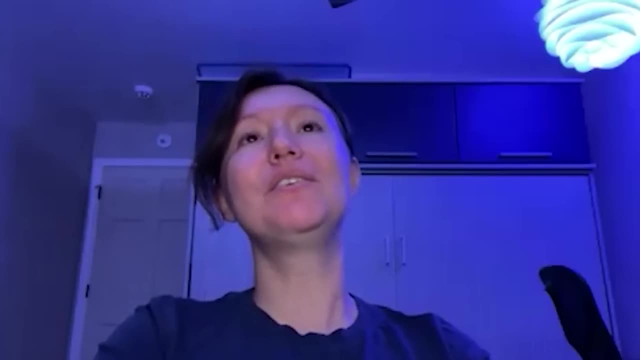 and if you were just like: oh, this is just, you know, and I still think some of them are, they don't think that it's actual shadows, but it is yet to been really confirmed. they've tried, we've been trying a few, a few times now, to get. 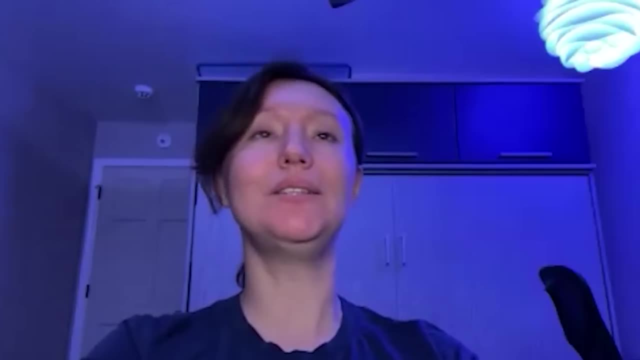 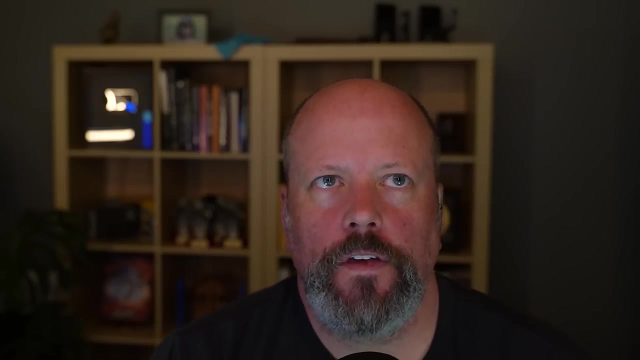 more Hubble time to try to confirm or deny whether or not they are. I think two times now that I mean the first time it was fourth, fourth quintile, but then the most recent one, I think was the first quintile, just still didn't quite make it. and so if it's, if it's real, then you've got this actively. 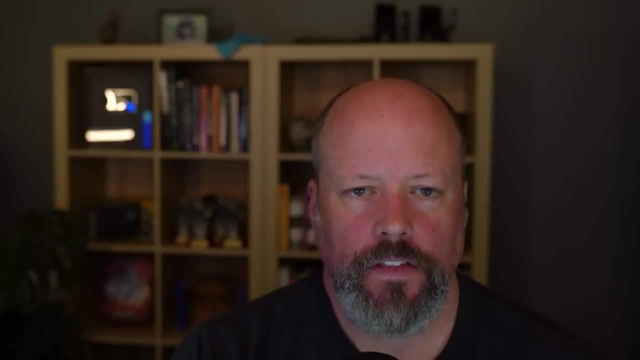 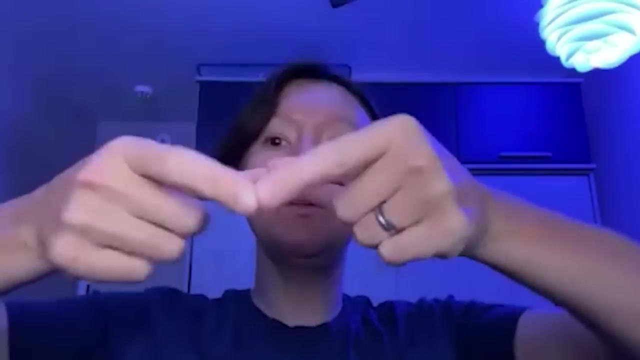 feeding supermassive black hole at the heart of the galaxy that is surrounded by a column, a pillar of dust, and it's casting a shadow out into space. it's like a dust donut around the light. yeah, the light, the light in the center and, depending on how you're looking at it, it's like a dust donut around the light. 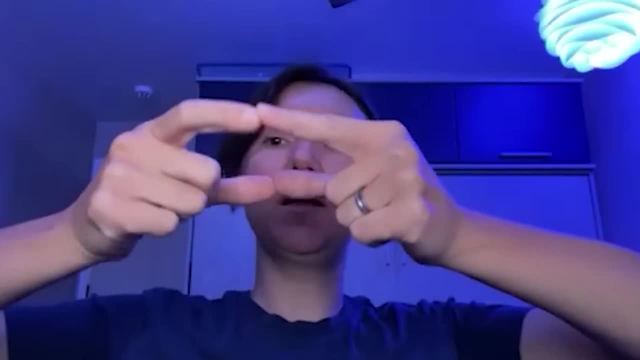 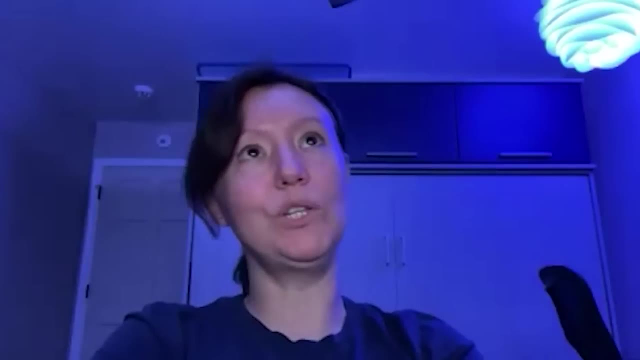 that dust is angled, it's gonna be casting light and shadows and you know depending on which way. so with this one, I think that it's sort of a- I've got a picture but I can't show it right now. it's like a distorted, a distorted. 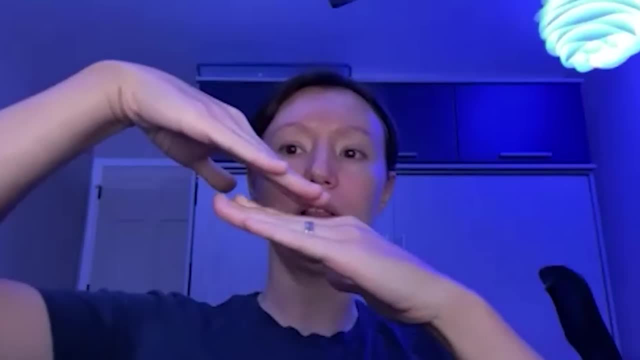 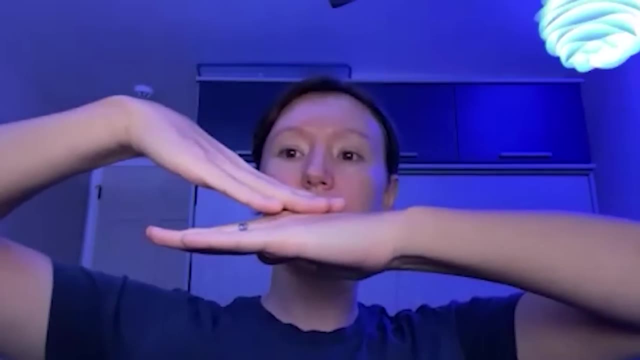 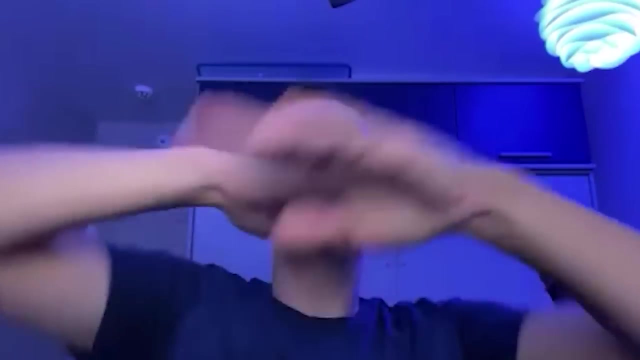 torus of dust where there's sort of a like here's, here's your edgewise donut, and then they've got sort of another one, like lift it up and crossing it like this, so we've got sort of two, two donuts, but I mean it's, it's a. 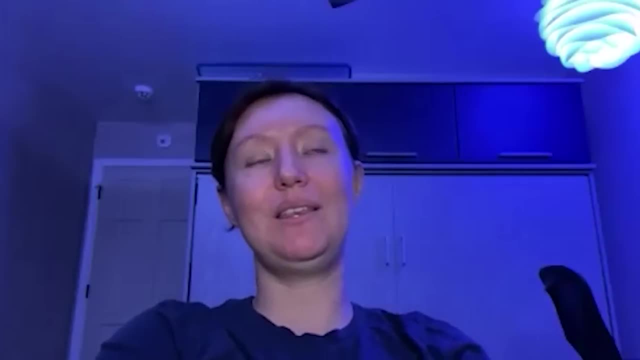 it's a difficult shape to describe, but because there's two of them, we've got two shadows coming out, and so that's what they think. that's also kind of hope, because it's just neat if it is. so I really hope that it. that's what it is. I. 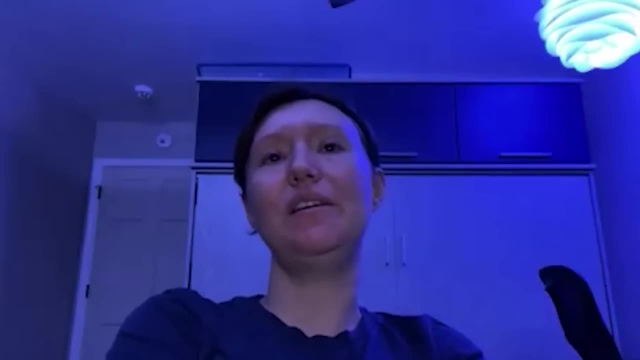 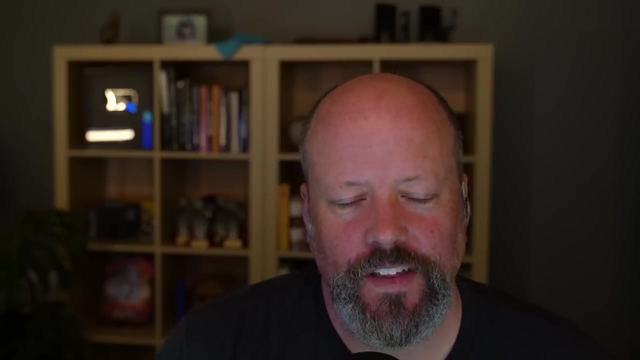 think it's not just it, because it also it is a disturbed galaxy. it's it's had some interaction in the past and you can see, obviously, that it's not, you know, a perfect disc. it's very. you're bringing a good scientific skepticism to the potential, and so I think that's that's important. and there was another recent 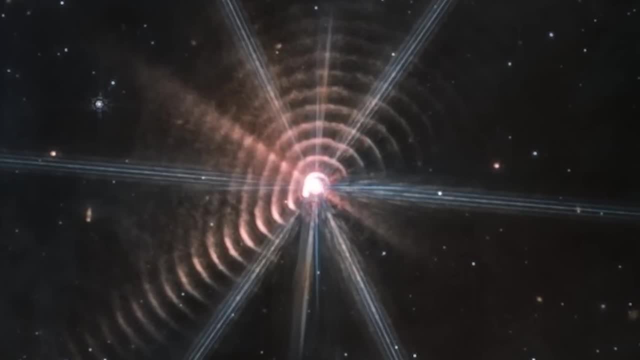 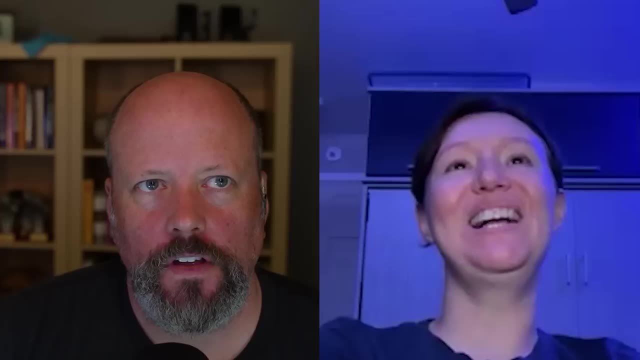 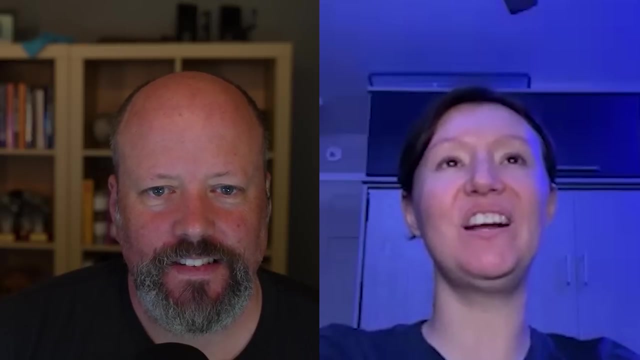 image that came out of web that I'm sure everybody is quite familiar with, these really cool concentric circles coming out of this wolf ray star and it's a. yeah, I'm glad that you said that correctly. I I did an interview recently where I just kept saying: right it. and then after the interview I was like that's not how you. 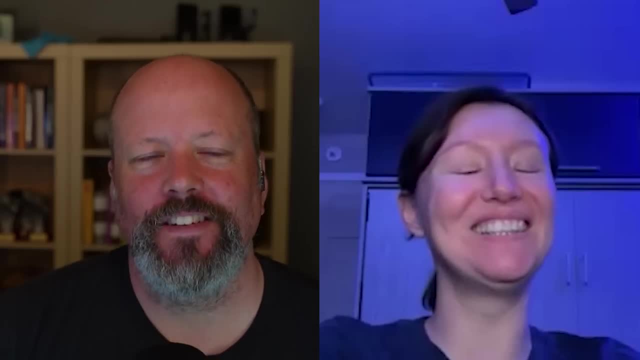 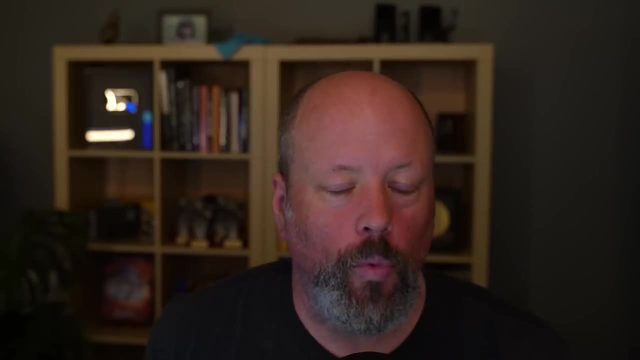 say that guy's name, it's right. maybe I don't know, this is why I can't watch myself, but but it's funny. but so you once again, you were like: what is this, what am? is this real? am I seeing this? and I I gotta confess that I get a lot of news. 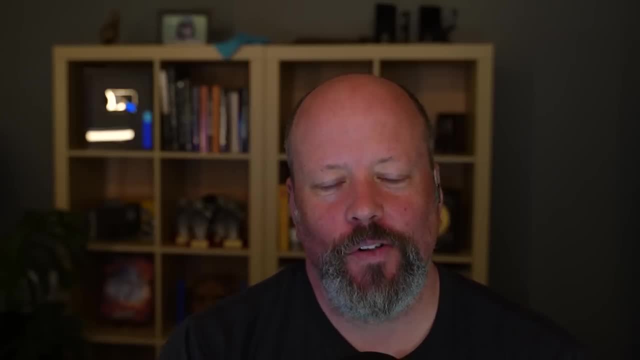 stories out of you- and I will often watch your Twitter. you put together an interesting image. I'll usually Nancy Atkinson will pick up the story and she's she's gonna write the the article about it and, and in this case we got stopped short by the scientists and they were like please don't write about it. 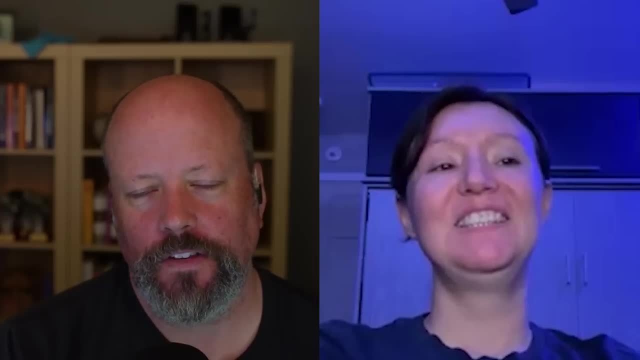 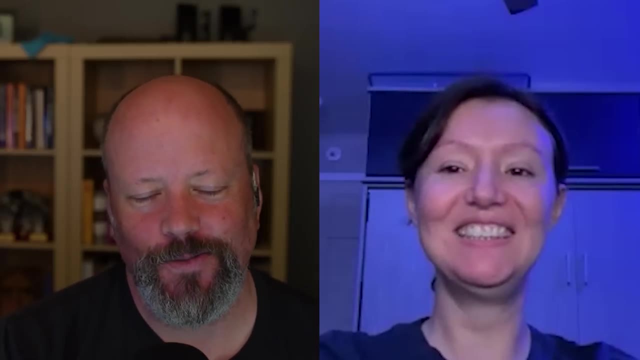 yet we're working on it and we want to have something that's peer-reviewed before. yeah, I felt bad, so we sat on the story and we were the only ones who who sat on the story, and we waited patiently until the scientists gave us the go ahead. 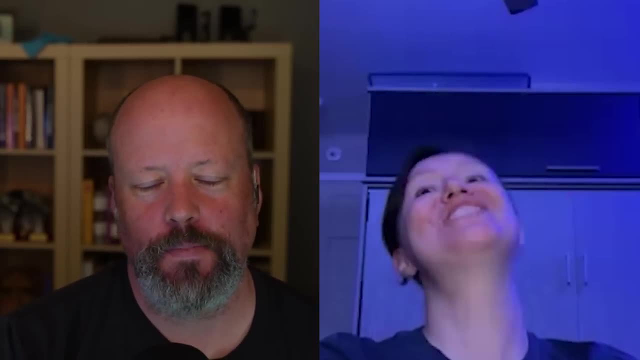 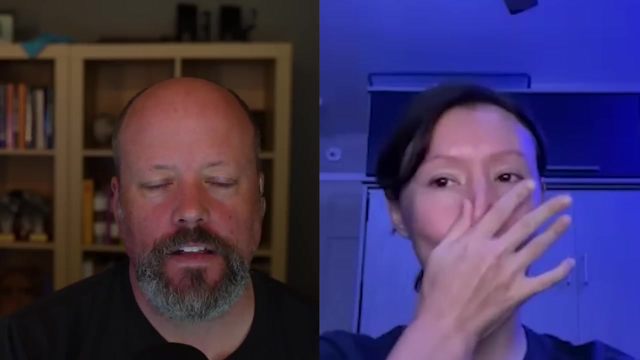 Well, everybody else, everybody else is just wild and speculated about it. Yeah, Yeah, So, but but you were the source, Like I had never seen anything like it And and you had had done some basic image processing on it, and just said: 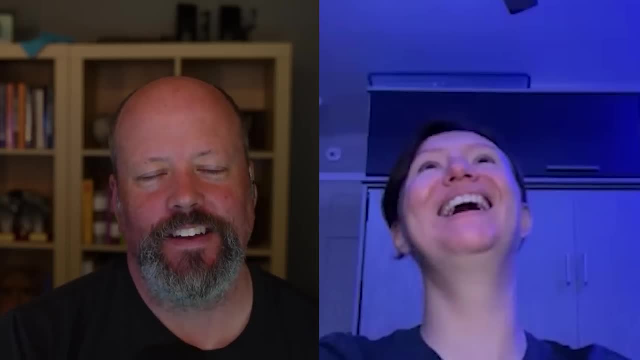 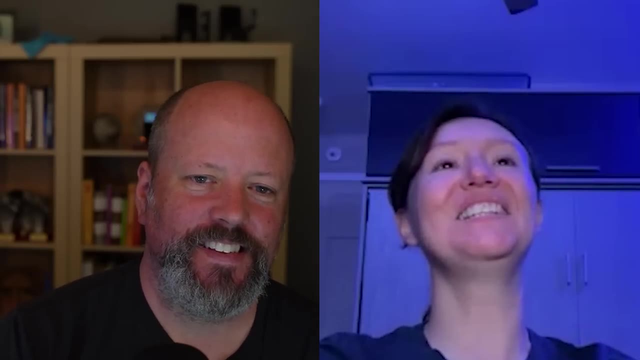 this is weird And I don't know what's going on, And does anybody know? And it just led to this whole big thing And I love that And I couldn't be more sorry to the- uh, the guy that actually like the PI, because he. 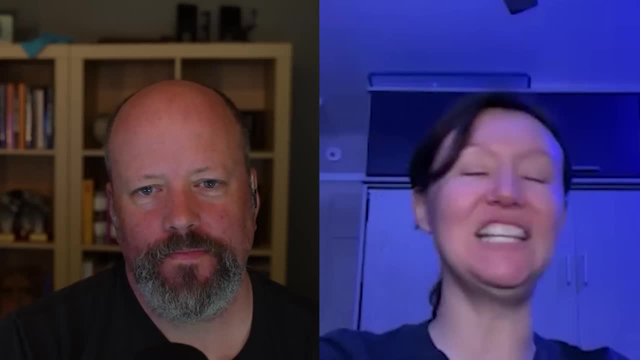 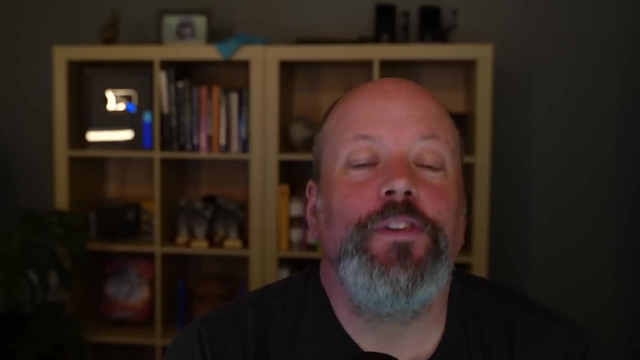 he's just. I mean, I I could just feel him like shaking his head at this whole Twitter thing. I'm just like I'm sorry, but it's awesome. Yeah, Well, that's the heart of it is that it's awesome. 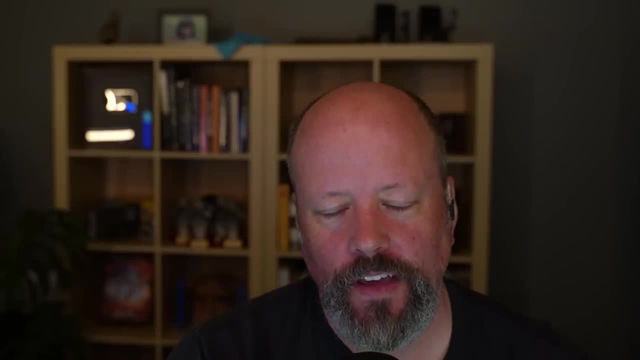 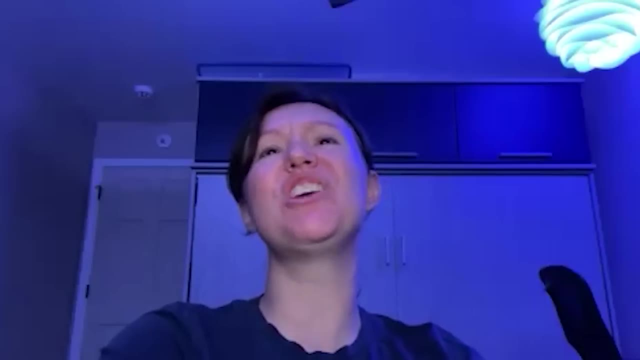 It's really cool And it's an interesting mystery And don't worry if you don't know what it is, It's okay, But but I I just the other day I got someone saying this isn't real, This is. 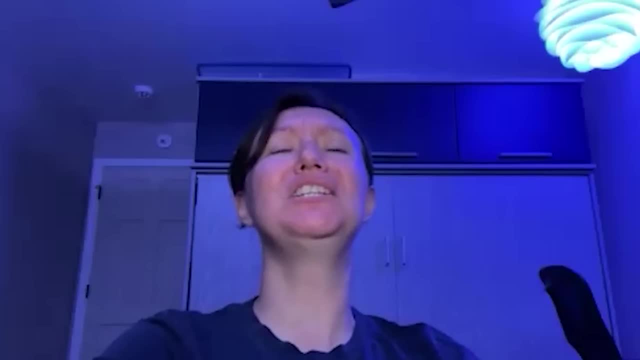 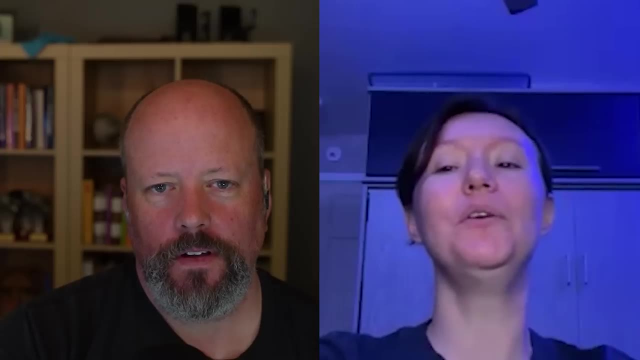 I don't know, Anytime I put this silly silly like. this is actually just a light echo or this is quantum something, something I'm like I'm just going to ignore you. Any of those would be fine. Those would be also be really interesting. 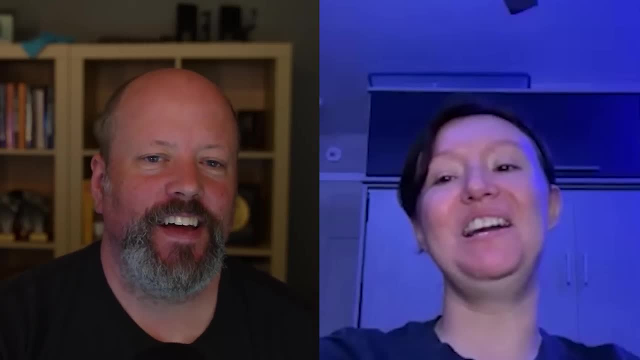 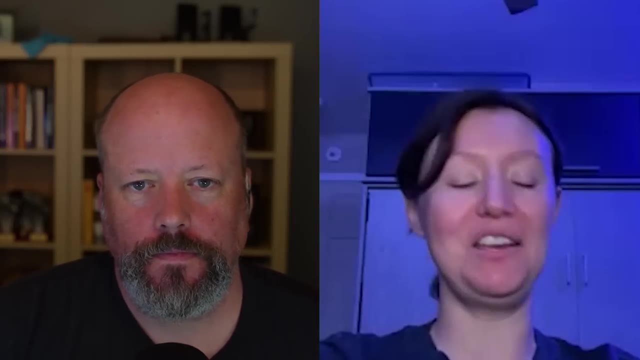 Any of that's perfectly acceptable. It's not that, no. but even I can tell you that it's not a like light echo, because they've taken data from, you know, X point in time to Y point in time And it's not moving like a light echo. 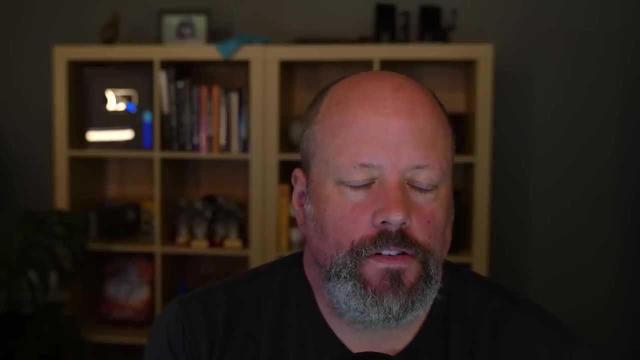 It's just it's not moving like a light echo. It's just it's not moving like a light echo. It's just it's not moving like a light echo. Now, if people want to get into doing this kind of image processing work, 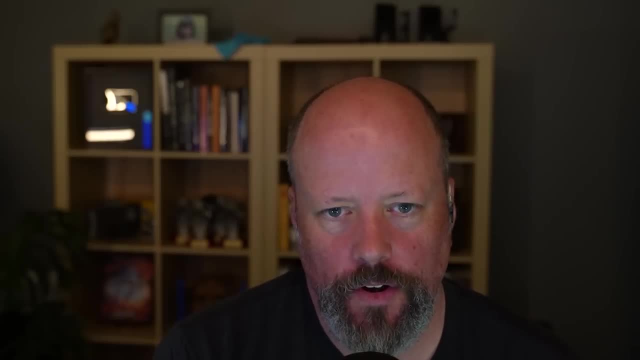 and I highly recommend space GEC on Twitter. follow Judy's Flickr account. Some of the most amazing images are there And again it is a. it is a fresh list of images that you will have never seen anywhere else, or you will see them on Judy's feed first. 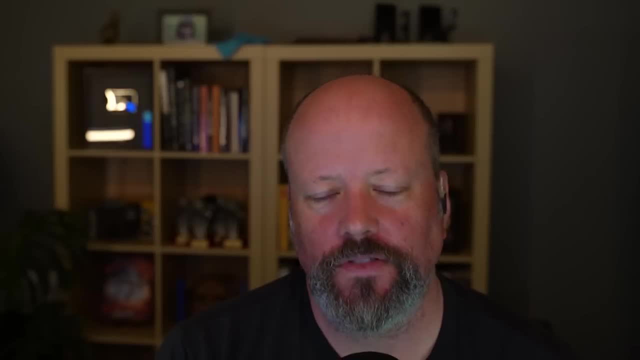 And then you'll see them on astronomy picture of the day and on the NASA picture of the day and attached to a press release, And and and and so on and so forth. So I highly recommend it, But if people want to follow in your footsteps, 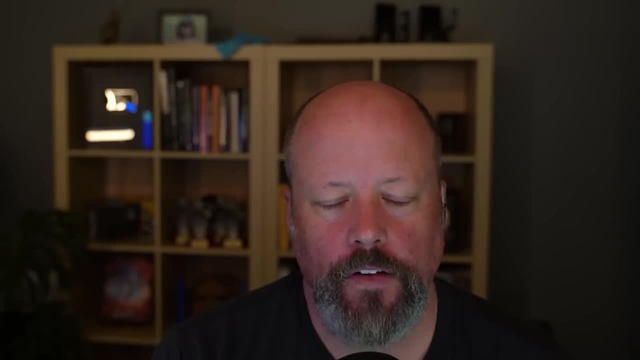 because I feel like you're kind of drinking from a fire hose of data and that there's. I feel sad for the enormous amounts of cool images that nobody will ever see, because nobody's taken the time to sit down and and look into them and dig them out. 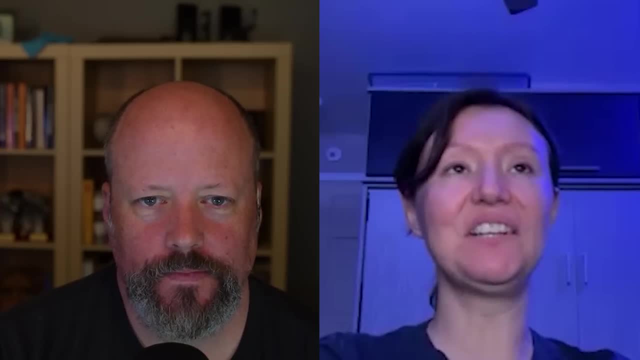 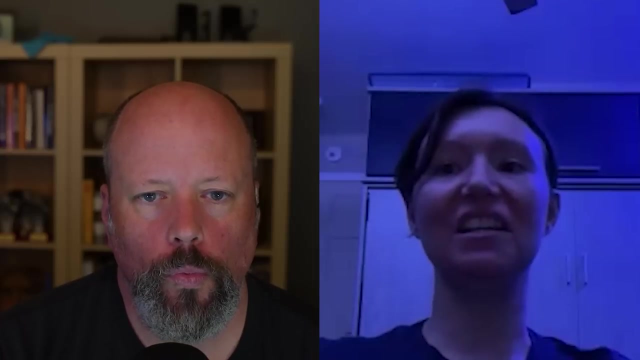 They will eventually. I just- oh my gosh, I've been taking such a long break. I feel so bad because I just have not posted anything in over a month now. So, but if people want to follow in your footsteps, I actually like. 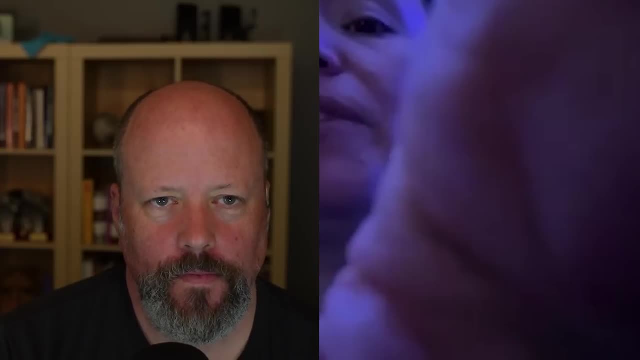 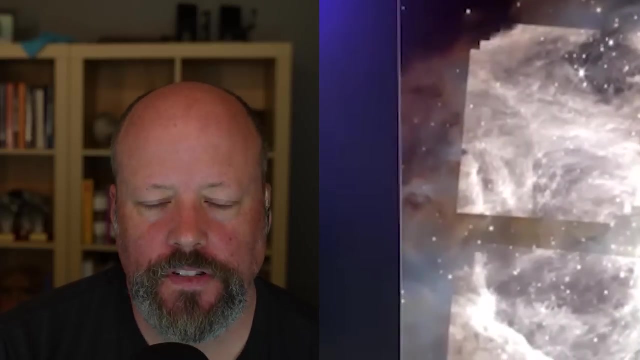 what's the best way to do it If they want to follow in my footsteps first off. uh, look at the look at the tutorial that I put. All right, We'll post a link to your tutorial in the show notes so people can. 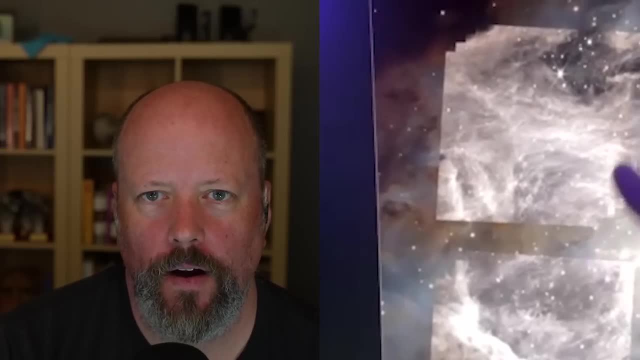 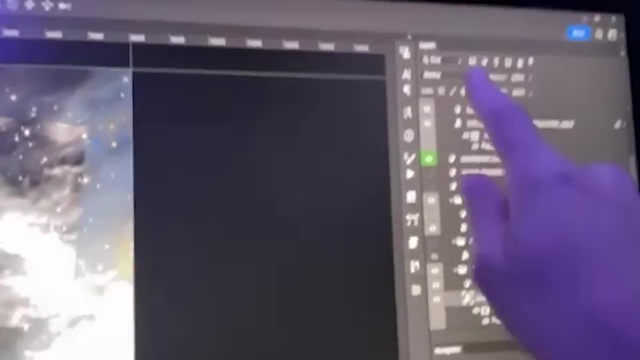 can, can find all the sources in the software and stuff. Wow, This thing that I have been working on, it's got. it's a. it's part of the early release data, but it's got. it's got 12 filters. 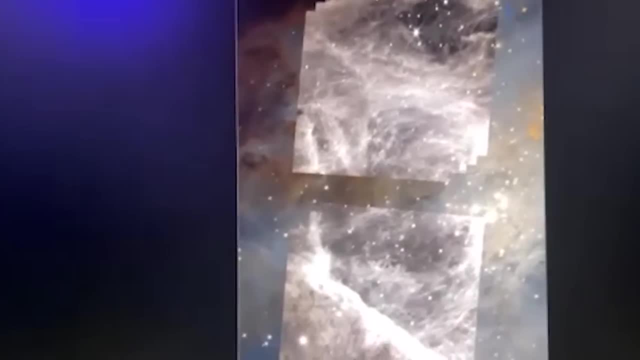 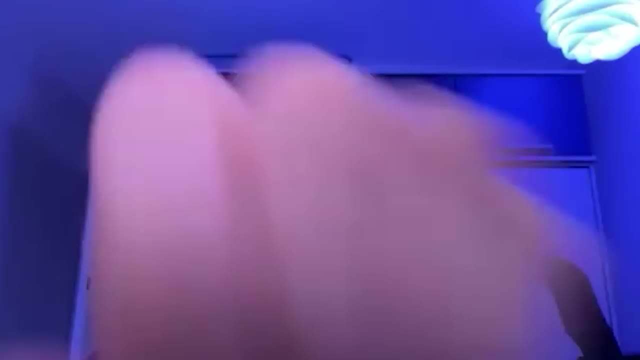 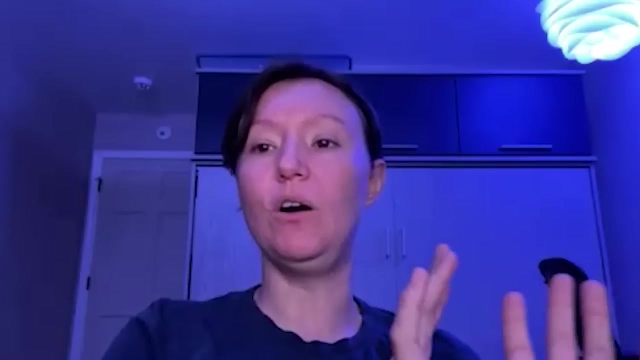 It's a big. I've been trying to clean it up and make it all pretty. Let me switch back to myself real quick, Uh, but I actually my plan with that is to put a Photoshop file on Google drive and let anyone download it. 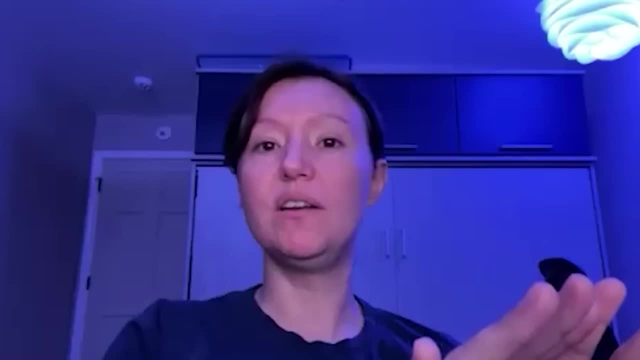 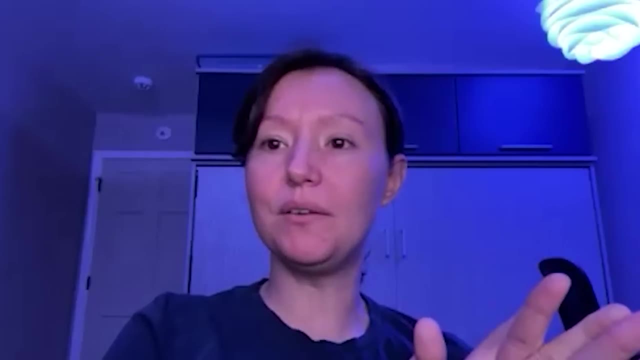 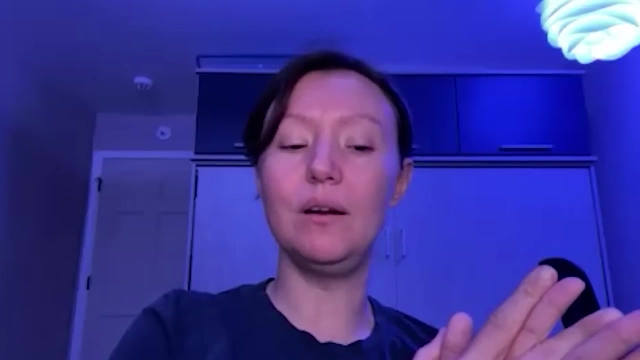 Nice And process it the way they want and see what they come, come up with, And I feel like that's one of the great ways to learn- Yeah, Not only about how to process, but how to look at scientific data and start understanding that, how. 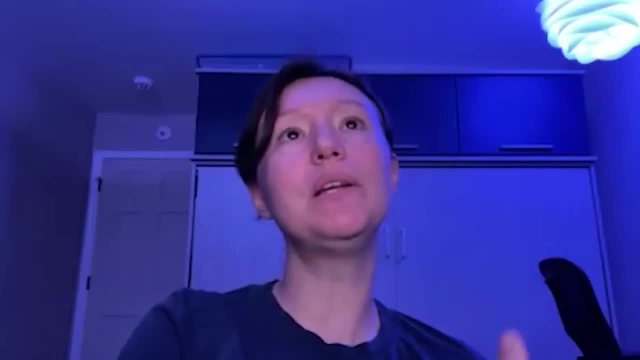 like how astronomers see it. So that's what I want to do. I've just been like really dragging my feet on it. I've- actually I did come up with a way of quickly getting those stars filled in, and it looks pretty decent too. 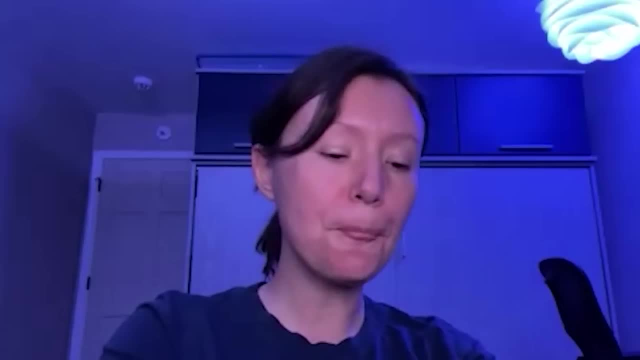 And I just have to do like the last 10% of cleaning, like cleaning up cosmic rays and making sure it's aligned, and then I can post it and then people can have fun with it and need to do it. Yeah, But I. 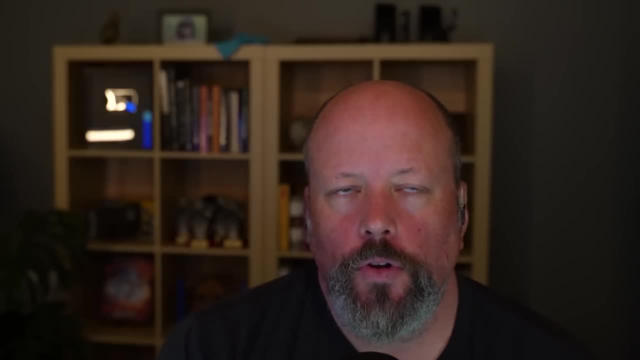 I mean I think that, like your trick of not trying to be the astrophotographer and the image processor was really wise, And, and after you sort of explained it to me, I'm like: Oh, I totally get it, because like 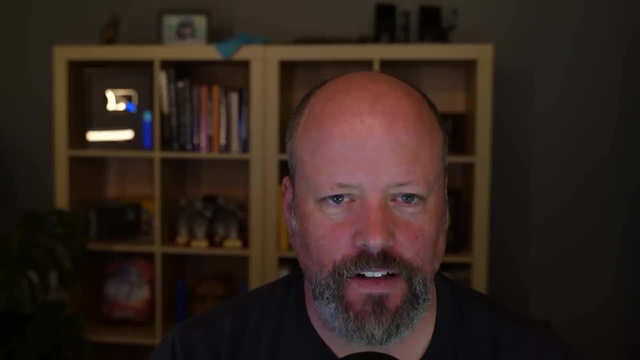 why not work with the best possible data from the best possible telescope? Hone your image skills And yeah, if you want to take your own pictures, go ahead. But but you will always feel sad that your technical ability to display the images doesn't match your vision. 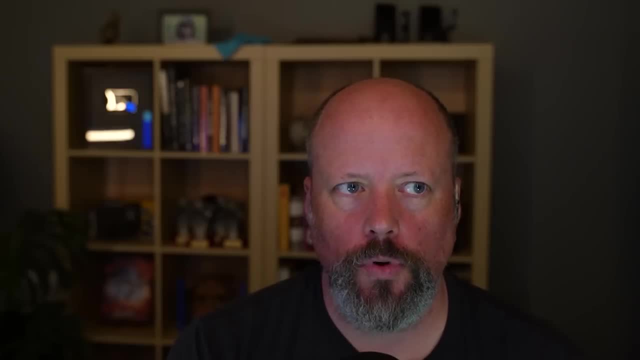 But if you go the other way around, really hone your craft in, in in working with the underlying images, then when you do your own astrophotography, you'll know how to take better pictures to to produce a better final image. 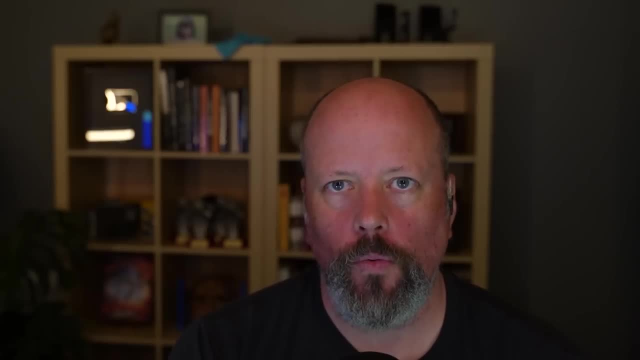 And I think a lot of people go the opposite way, And I think your way is exactly right And in your case, you will probably never take your own pictures, but still. but I think it's the right way to approach it. So people want to become. 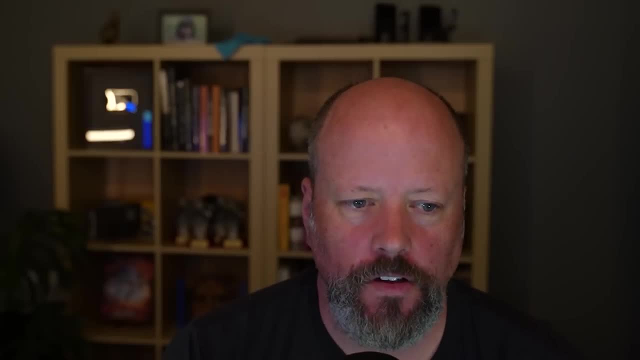 and so we always ask me, like: I want to buy a telescope, I want to get into astrophotography. What should I do? My advice is becoming: do what Judy does: learn to get really good at image processing. Then your data will make you really happy when you. 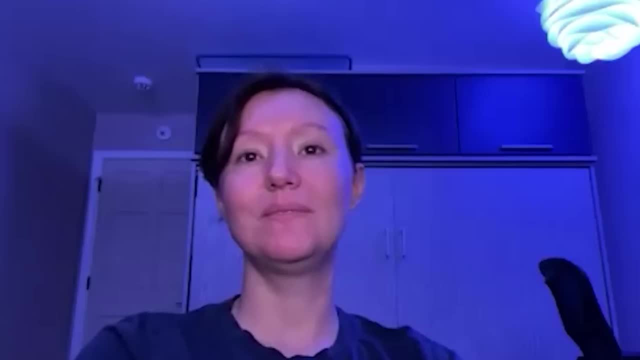 when you try to do your, when you actually start taking your own pictures. That's awesome. I never, I never thought about it, but it like that, but it does like. that does make perfect sense. It really is two separate skills. 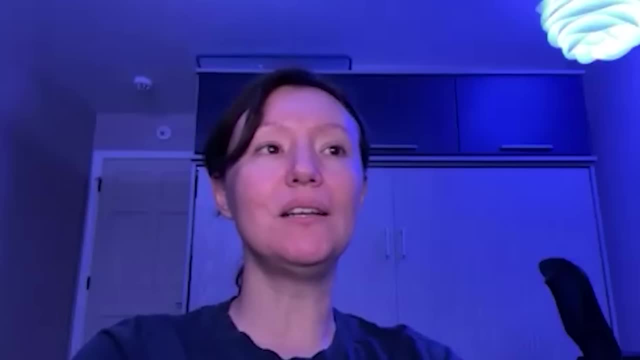 And if you don't like, yeah, like to get good data is one thing, but then, man, if you finally get that really good data and you can't- you don't know how to process it- That really would like, that would be sad. 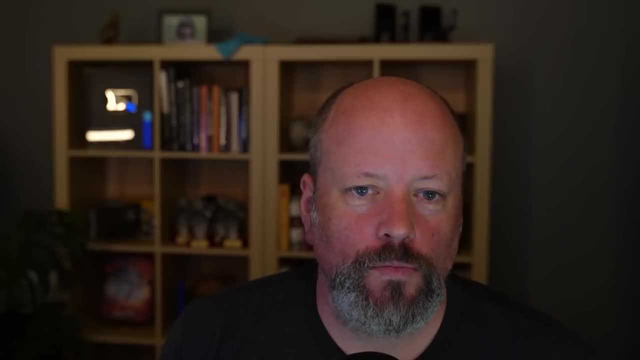 Yes, Cause, like, like man, I think we even did this. I took a bunch of pictures. I couldn't make it do anything. I send them over to you. You were like I just took a minute and it was a thousand times better than anything I was. 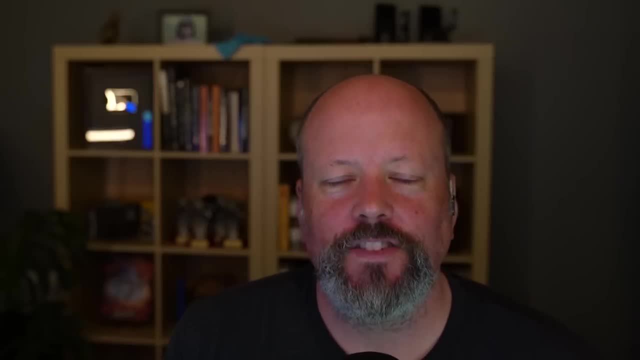 able to produce because you just knew what you were doing. And so that's the feeling that I had. I was like why I'm doing this the wrong way? I shouldn't be learning to use a telescope, I should be learning to image process. 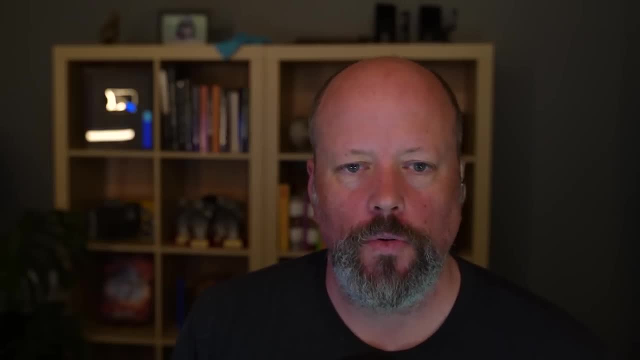 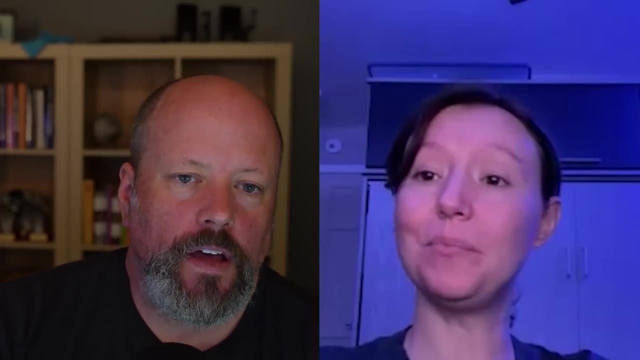 And then I'll come back around and use the telescope Once I know what I'm doing with the images, because that's the final output And I think it's it's really important. Well, Judy has been. yeah, lots of practice data that anyone can. 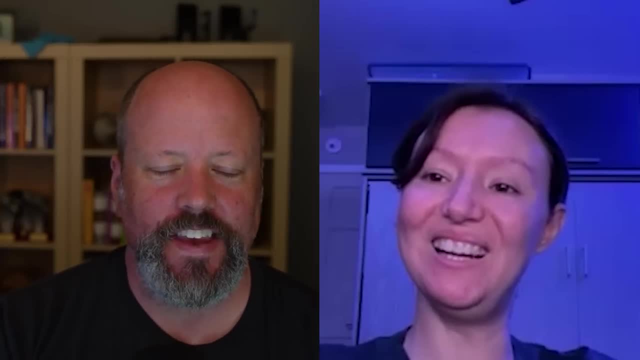 That's exactly it. Yeah, You got 30 years of Hubble data and now you're. and now the James Webb data is starting to pile up, Plus the ESO data, plus curiosity. It goes on and on. Well, Judy. 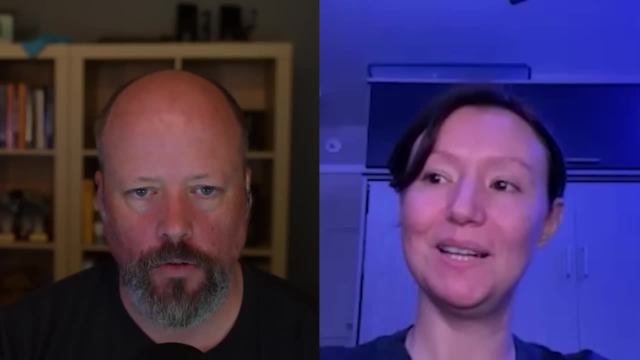 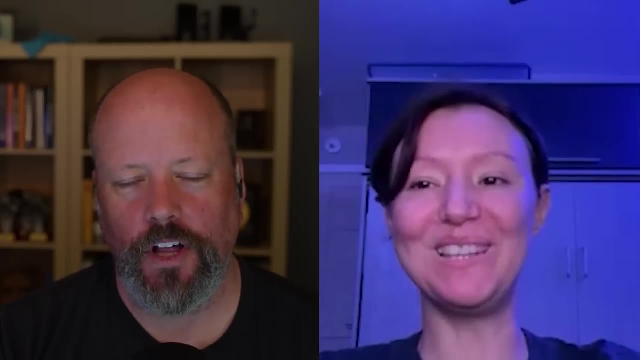 it's been a pleasure talking to you. Thank you so much for the contribution that you make to the astronomical community. Like I said, I follow your work religiously. It turns into a lot of stories on universe today And I know that you're making a difference in the scientific 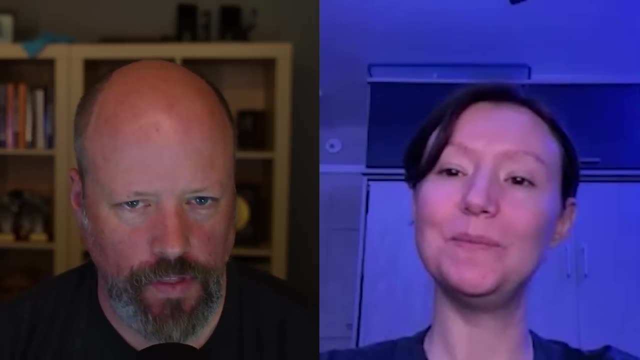 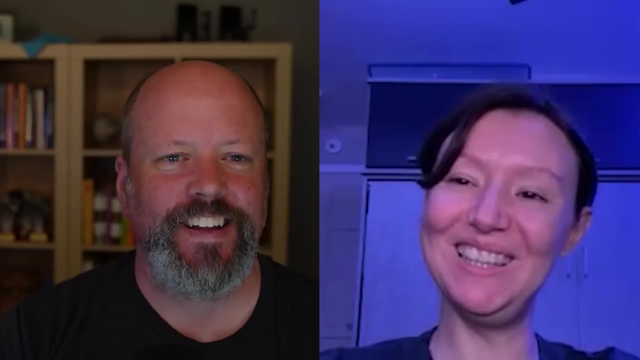 the scientific community as well, And I know a lot of people out there really appreciate what you're doing, So thank you. Thank you, Frazier, And you're almost welcome. All right, I look forward to. I look forward to this picture finally being released. 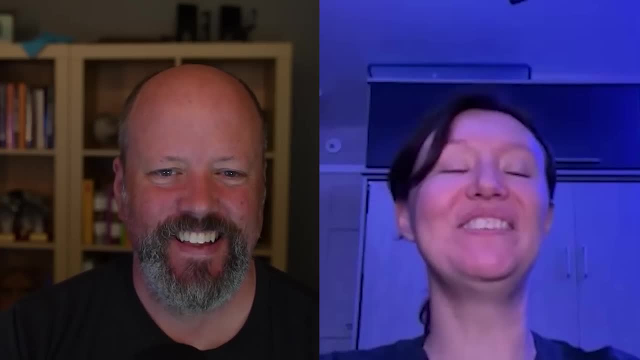 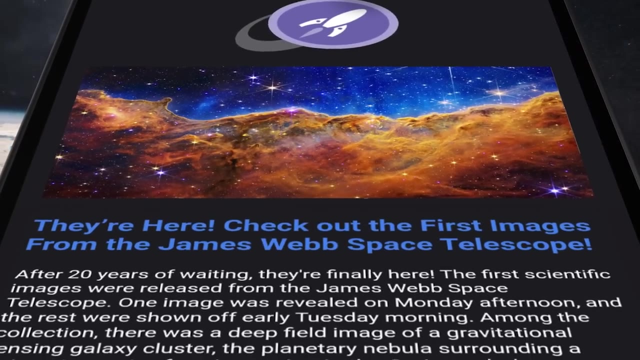 right, I uh. maybe this will finally motivate me to go in and finish it. Awesome, All right, Take care. All right, Bye, Bye. You can get even more space news in my weekly email newsletter. I send it out every Friday to more than 55,000 people. 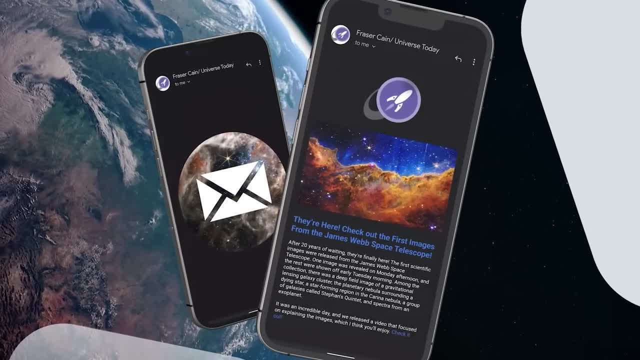 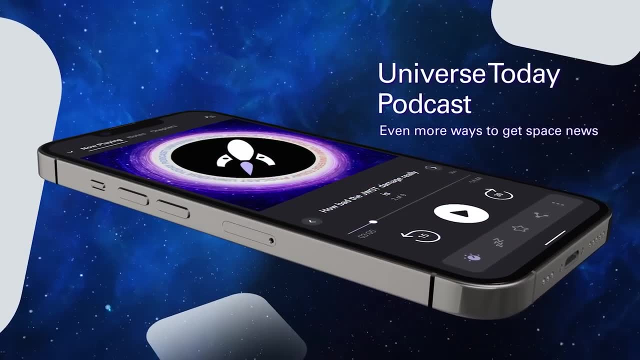 I write every word. There's no ads and it's absolutely free. Subscribe: add universe todaycom slash newsletter. You can also subscribe to the universe today podcast. There you can find an audio version of all our news, interviews and Q and A's, as well as exclusive content. 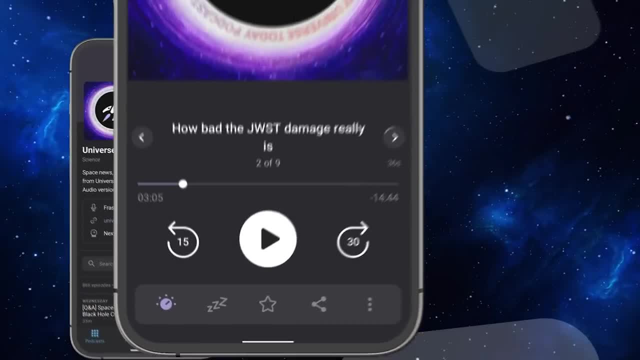 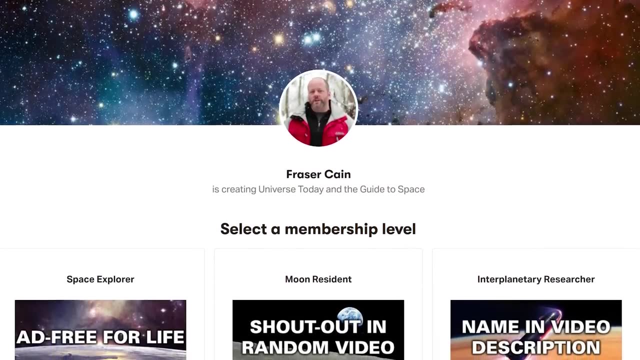 Subscribe at universe todaycom slash podcast or search for universe today on Apple podcasts, Spotify or wherever you get your podcasts. A huge thanks to everyone who supports us on Patreon and helps us stay independent. Thanks to all the interplanetary researchers, the interstellar adventurers. 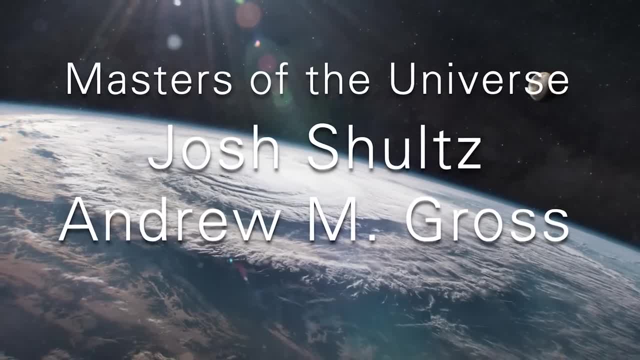 and the galaxy wanderers, And a special thanks to Josh Schultz and Andrew M Gross, who support us at the master of the universe level. All your support means the universe to us.